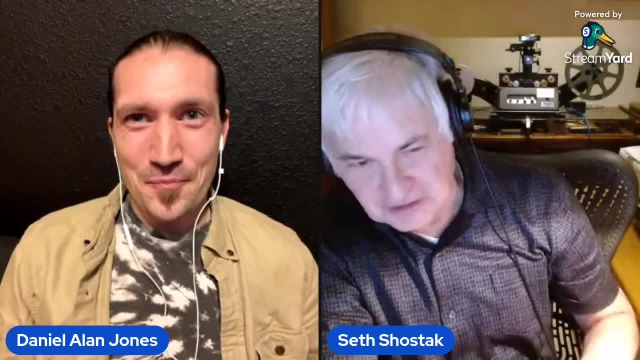 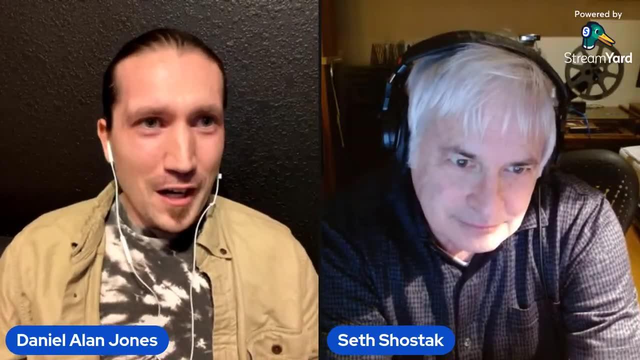 Doctor, it's an honor to be able to have you here with us. Welcome to the Vortex. Thank you very much, Daniel. So you've done an amazing job of not only communicating scientific ideas and being able to provide them to the public in a way that makes sense. 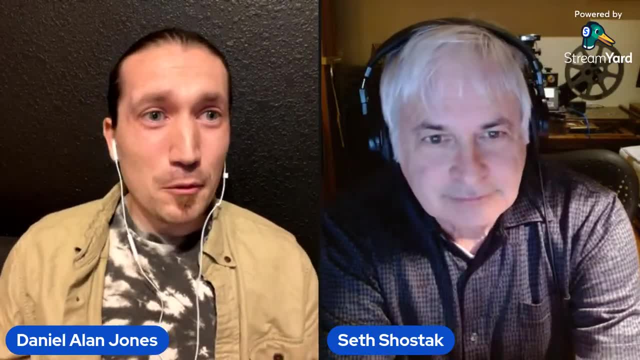 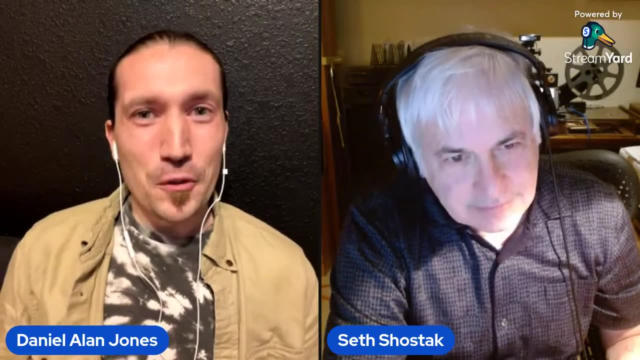 but you're dealing with a lot of really interesting subjects that many people usually relegate to science fiction. When it comes to SETI, this is the search for extraterrestrial intelligence. What's fascinating about this is that it's not just extraterrestrial life you're looking for. 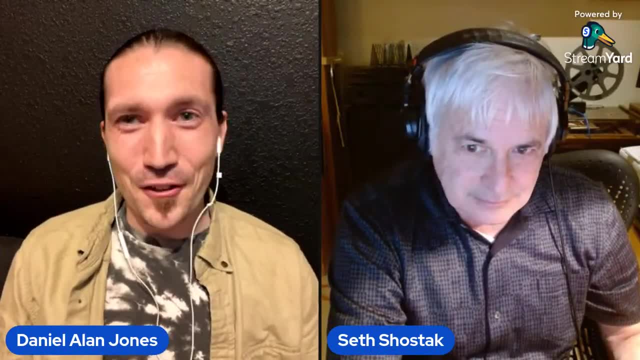 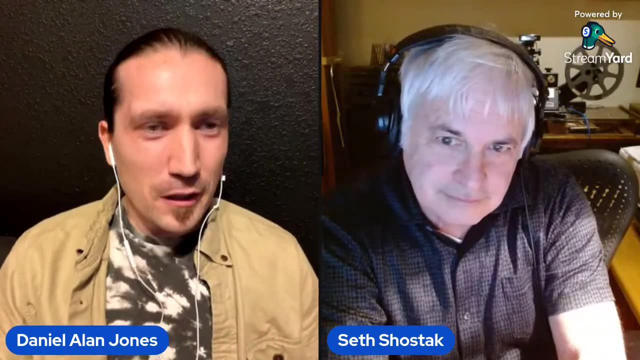 although that's a proponent of it. it's intelligent life. So it's not subtle, it's not just extraterrestrial life, it's intelligent life. So give us a little bit of a history, A preface of how this organization has come about. 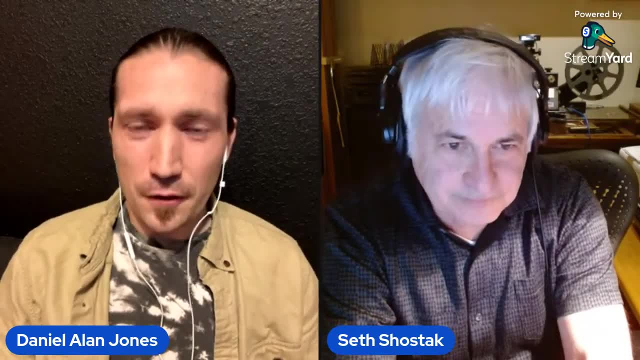 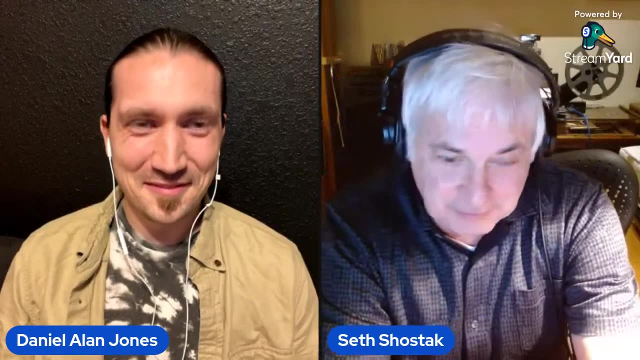 and sort of the journey it's taken to get to the point where it is now, if you don't mind. Well, the idea that there might be aliens out there, that's nothing new actually. You know, you can go back 2,500 years and the ancient Greeks, the classical Greeks, if you will. 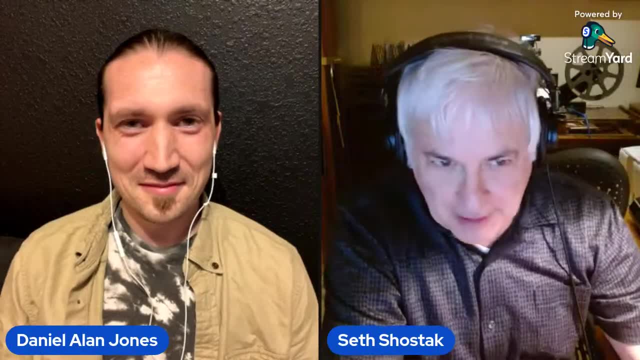 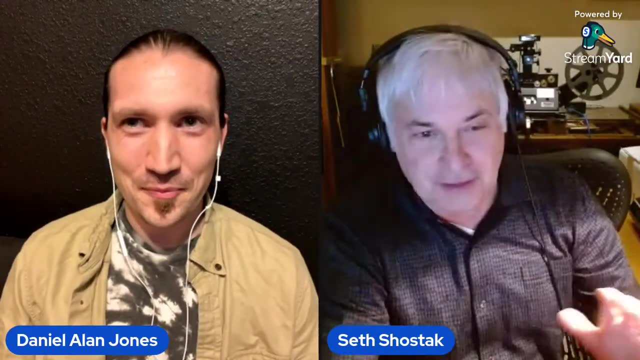 they were already talking about how probably everything in the sky was occupied by either men or men-like creatures, or women or gods right, They just assumed that, And the Greeks were not big on doing experiments, so they didn't invent telescopes or anything like that. 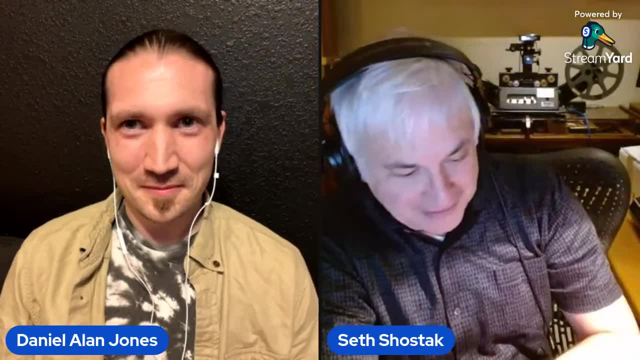 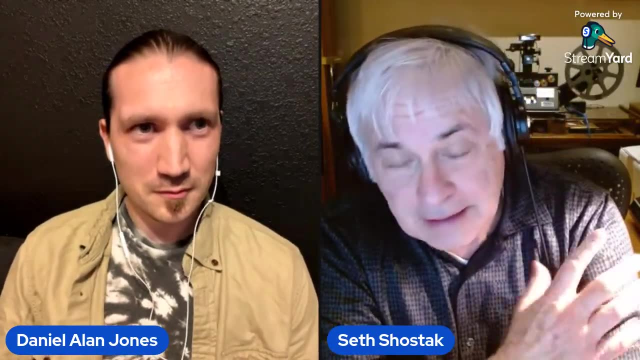 that might have helped them to learn more about these places where they had, you know, these places they had populated with inhabitants, But they, at least you know, sort of broached the idea. Really, there were some experiments that were being done by people like Tesla, right, 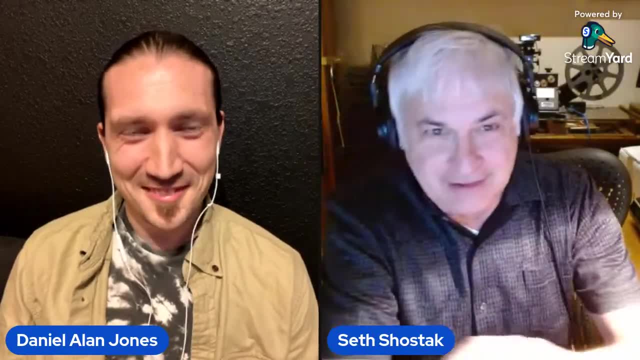 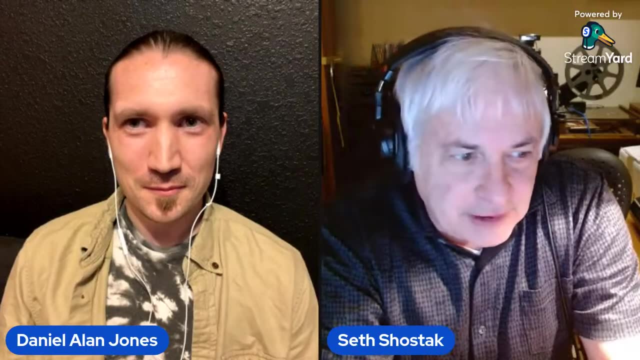 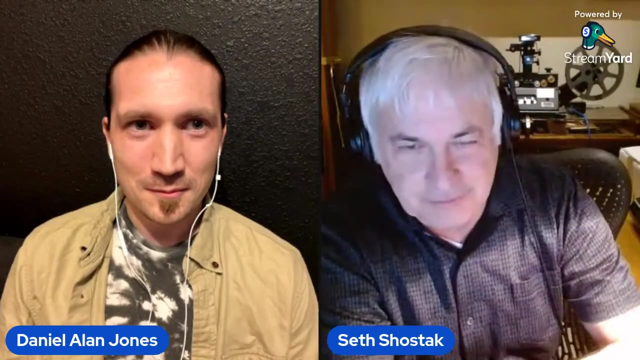 Nikola Tesla, not that automobile guy, but the electrical engineer who was doing things near the beginning of the 20th century in which he was trying to see if he could prove that there might be somebody out there. He was building these big static electricity devices. 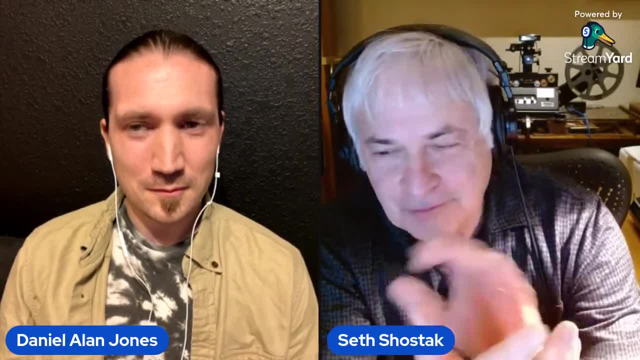 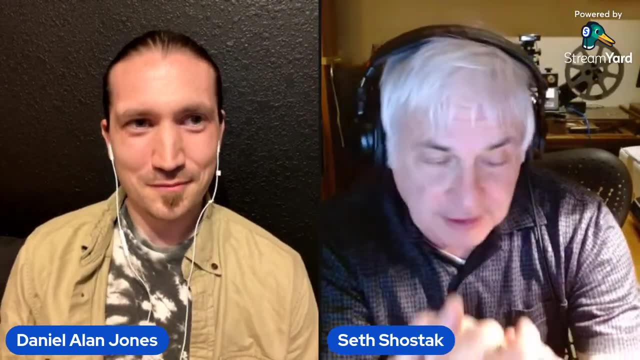 Tesla coils and so forth are sort of the follow-up to that, And he was trying to see if he could pick up signals from other worlds and, in particular, Mars. So, and, by the way, I think that he felt that he had picked them up. 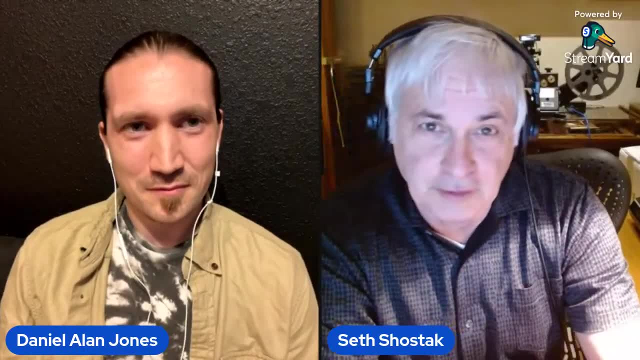 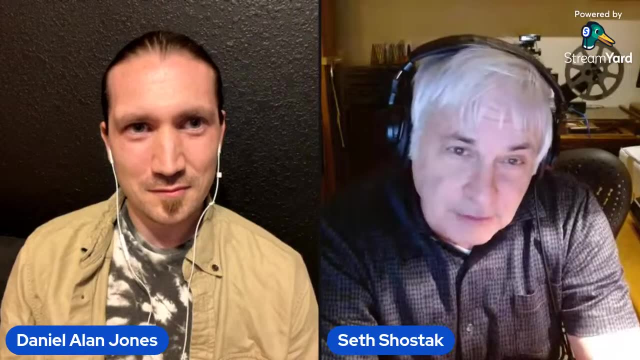 Marconi, who was of course a radio pioneer. he also thought he had heard the Martians. The Martians were busy with their own broadcast schedule, I guess, But in any case, you know, that was sort of the history here. 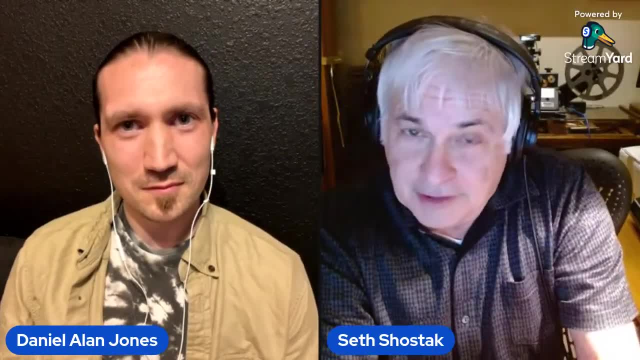 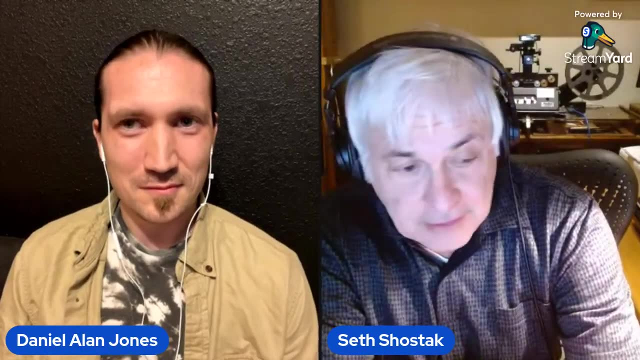 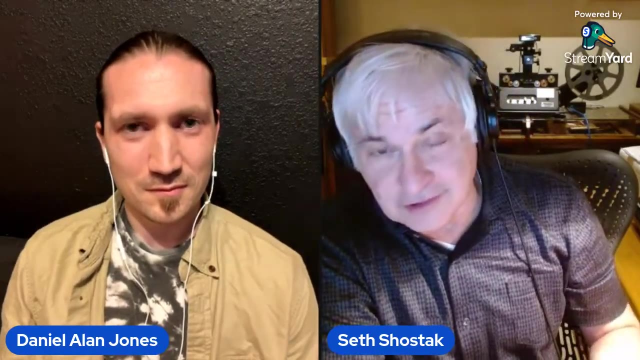 But it wasn't based on very much astronomy. We didn't have enough astronomy to really know whether Mars or any of the other nearby worlds actually had any inhabitants. But beyond that we also didn't have any way to find them, And that changed after the Second World War and in particular in 1960,. 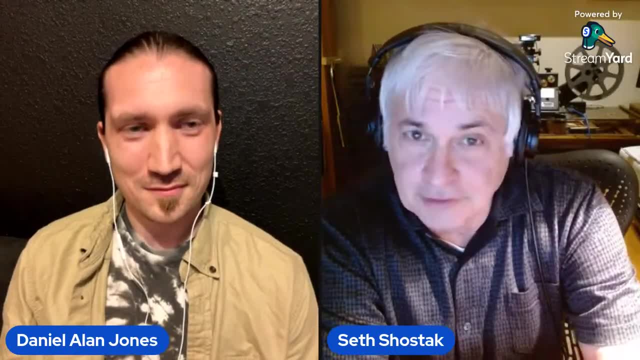 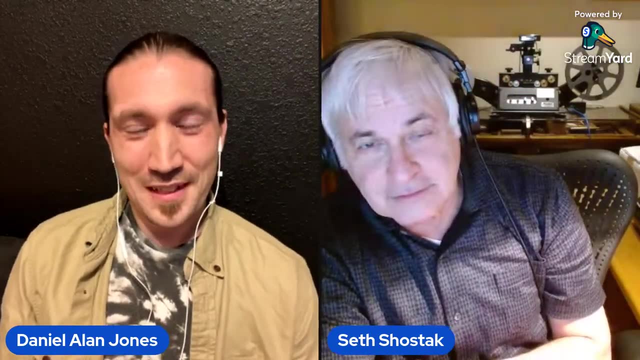 when a guy by the name of Frank Dray, who was a scientist, did the first modern SETI experiment, which he used, you know, sophisticated receivers to try and pick up signals coming from the skies, It's incredible to see how far things have come. 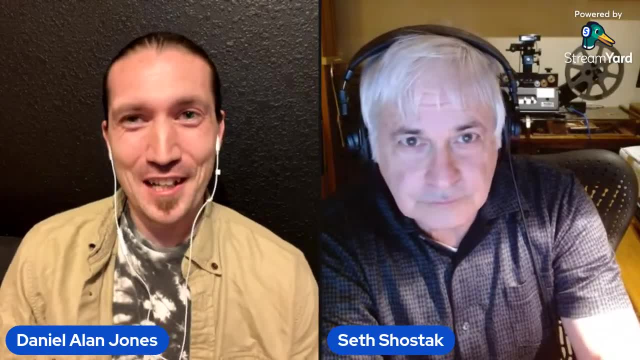 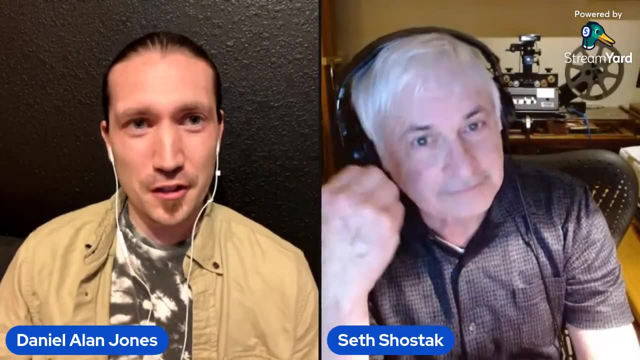 And even in just the short amount of time- the few decades it seems to lead up to what we're dealing with now, and all the possibilities, I think there's a lot of potential for the scientific work that you've been doing for a number of years. 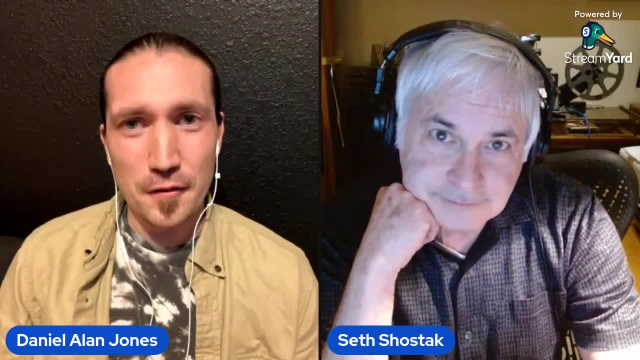 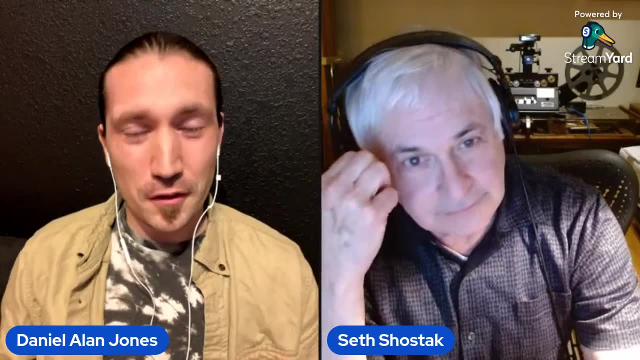 as well as how this connects to a larger scale of what people can learn about, with not just what's here in our world but the rest of the universe, and how that changes the scope of awareness for all of society. And, that being said, when it comes to SETI, it's something that you know. 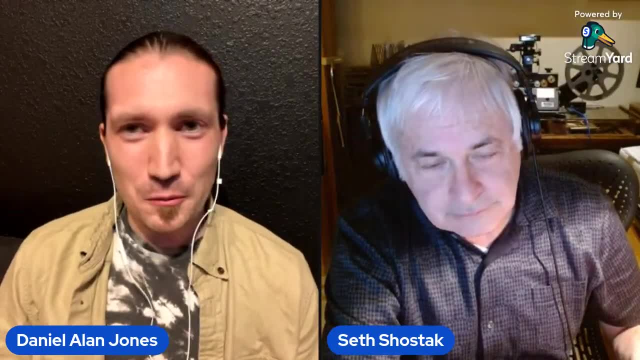 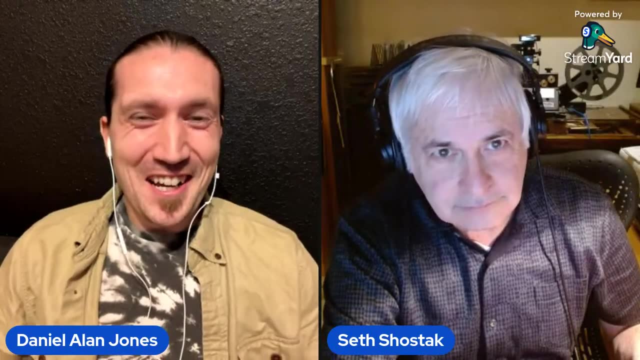 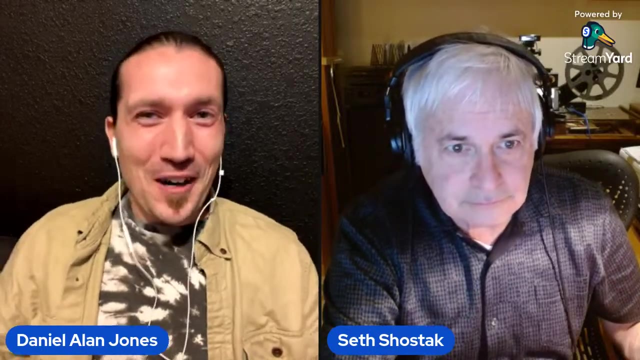 people, I think, generally wonder: how are you going to communicate, How are you going to search, How are you going to find these aliens? And to do a little bit of a you know less considered scientific method of here channeling in, of course, Enrico Fermi, wondering where are they? 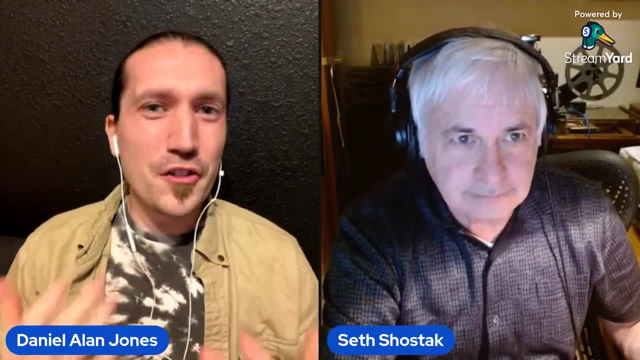 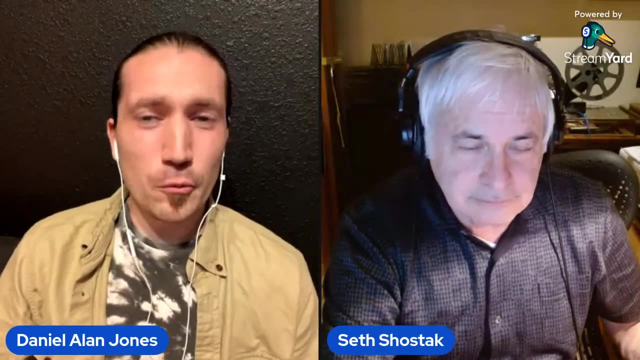 And so you know how are some of these things being done, What are the techniques and methods behind SETI's instruments that are being used to try to ascertain the evidence? What are the types of things that we can see that most people, probably you know? 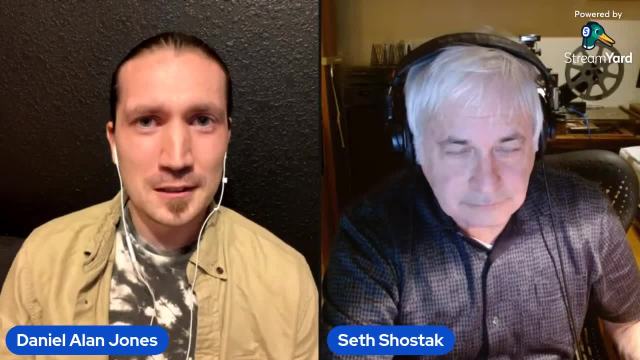 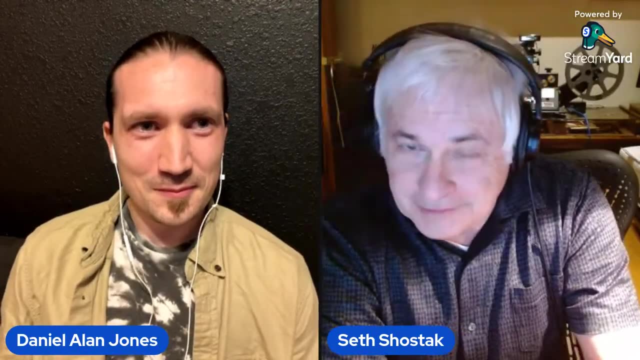 think are too technical, that help this type of effort to go Well. there's no doubt, Daniel, that the technology being used for SETI experiments today. obviously it's quite a bit different than it was even 20 years ago, But the basic idea is very simple. 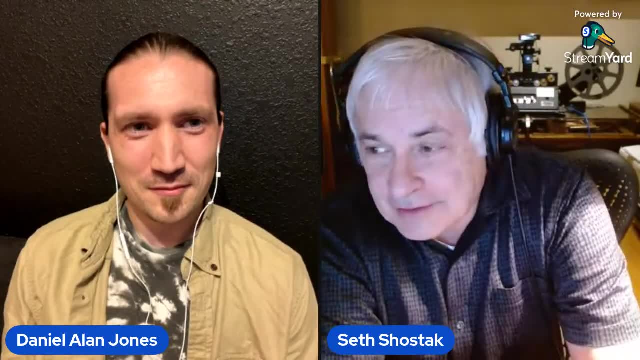 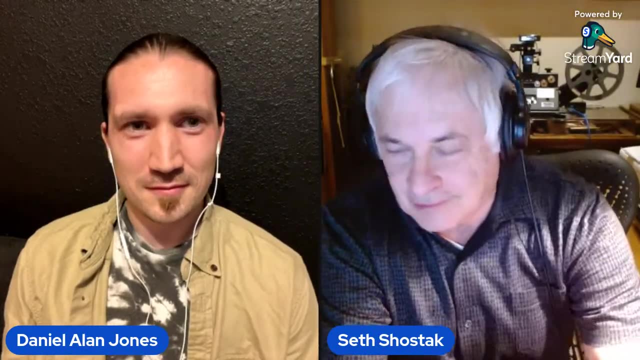 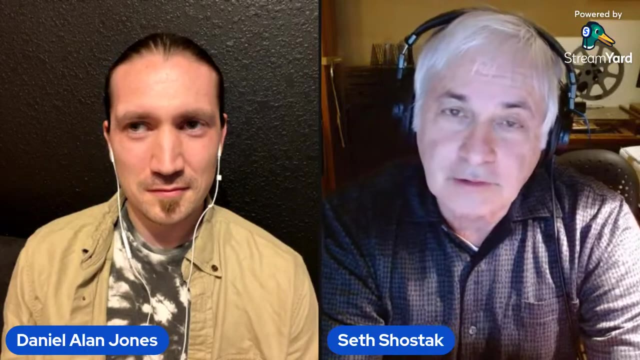 Everybody can understand the idea right, And that is that look, if the galaxy, or, for that matter, the universe, is populated by beings, whatever they look like, beings that you know have developed science and technology. okay, then they're probably using radio transmitters. 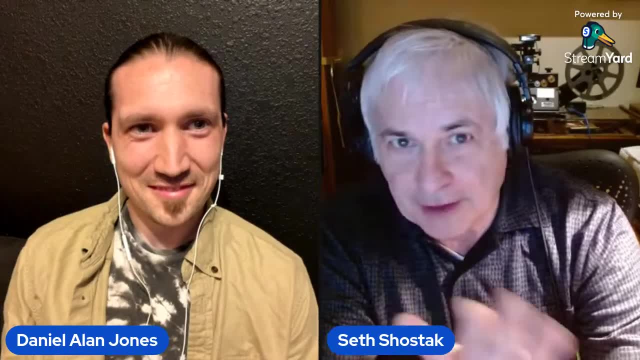 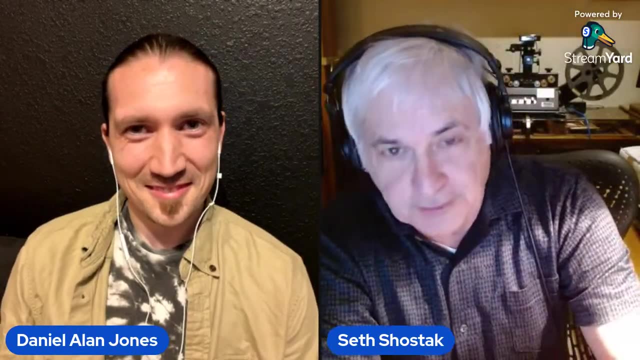 Well, when I say radio, that means television too, and radar. All of that is radio, That they're using transmitters to try and get information from one place to another, And it might, you know, just be the top 40, or it might be, you know, telephone, long-distance telephone. 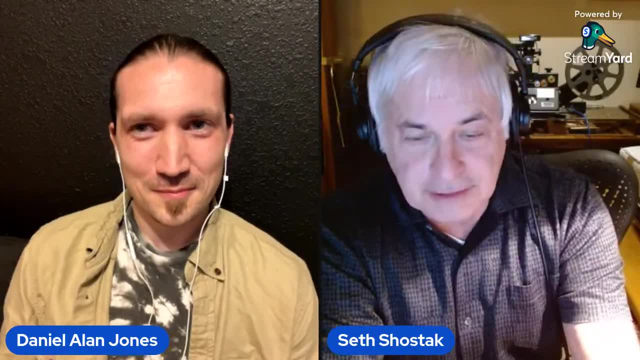 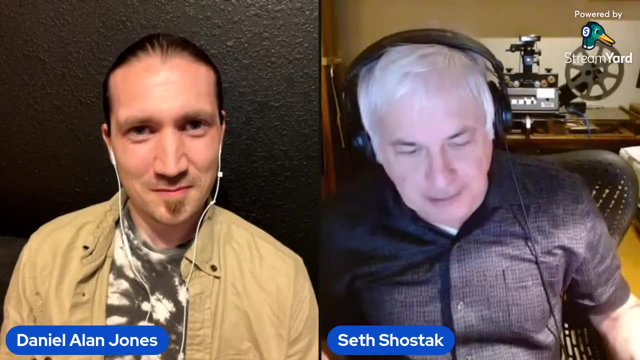 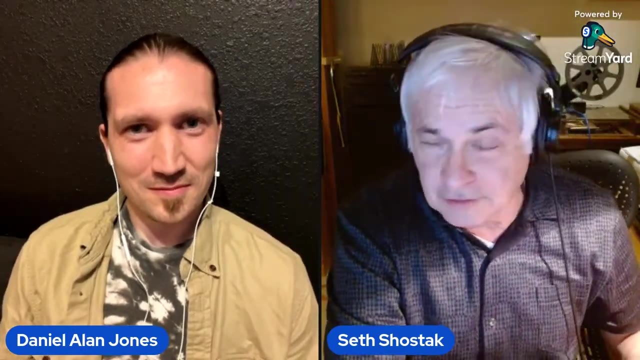 I mean whatever, it is okay, You can send any kind of information on a radio beam, okay. So the idea was: well, look if the galaxy is populated by other societies, presumably all of them using radio, if they've gotten that far with their technology development. 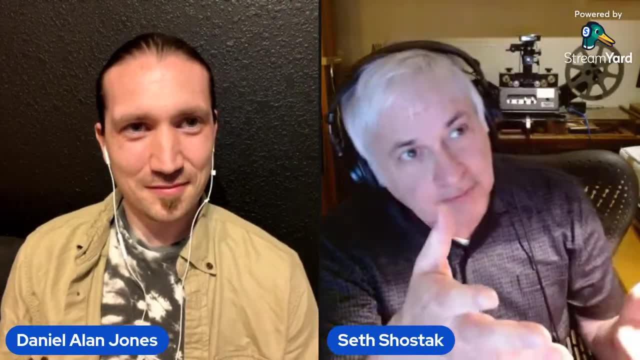 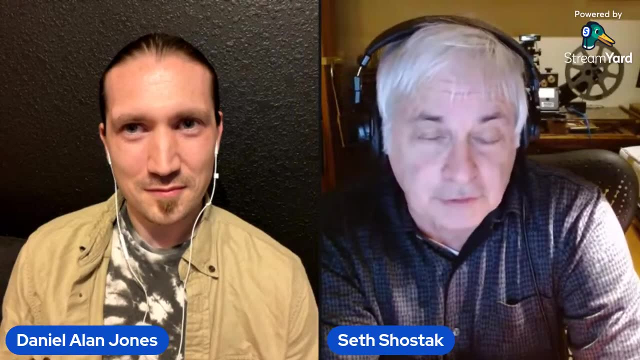 then if we just point a big antenna at this guy, aim it maybe in the direction of some nearby star systems, maybe we'll pick up the radio traffic. We'll just eavesdrop on their radio traffic. That's the idea And that hasn't changed right. 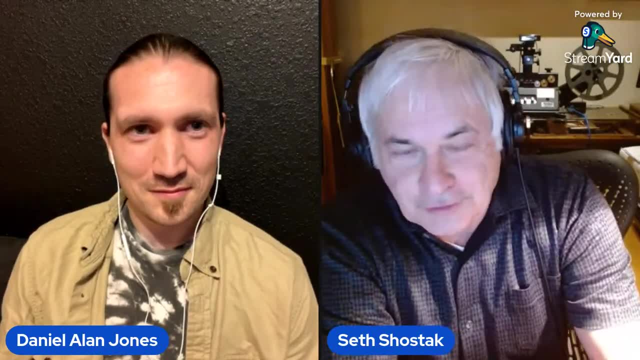 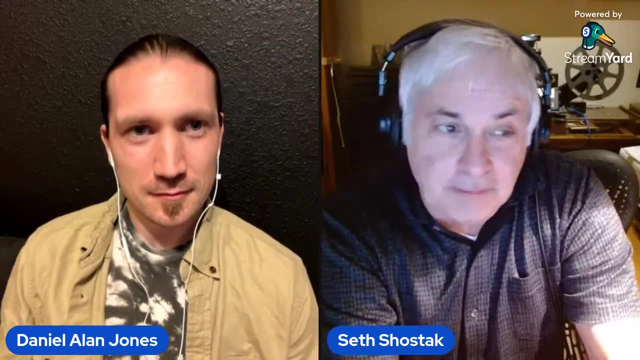 We don't broadcast inquiries and ask for the aliens to reply, you know, and say, hey look, we're the Earthlings, and let us know if you're out there, right? Because I mean that might or might not work. 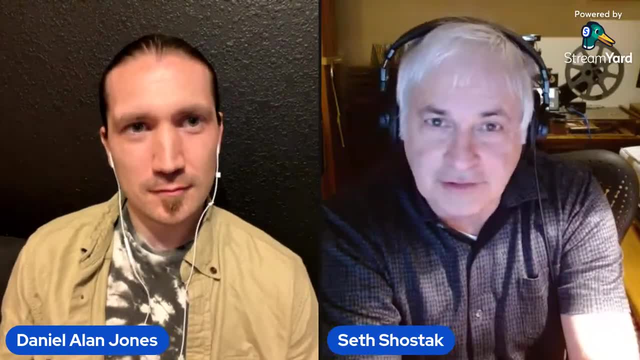 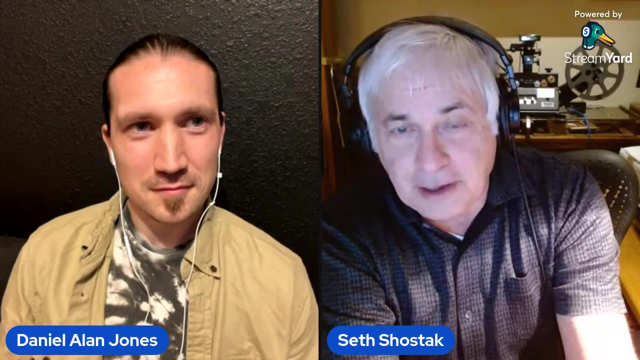 but you know that's a sociology question. But the real problem with it is that the nearest aliens might be. who knows how far they might be? dozens of light years, they might be hundreds, they might even be a thousand light years away. 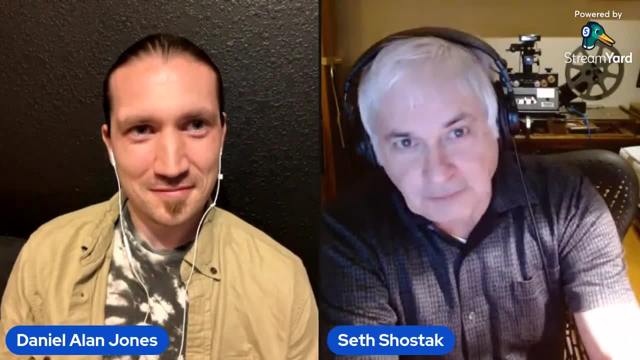 And that means you know you say something to them and it takes up to a thousand years, say, for them to get the message you know, and then another thousand years you've got to wait for the reply to come here. 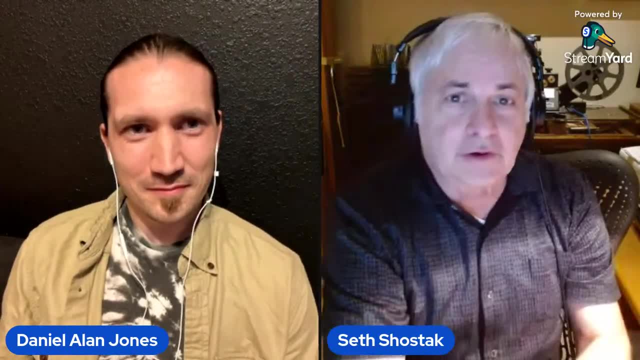 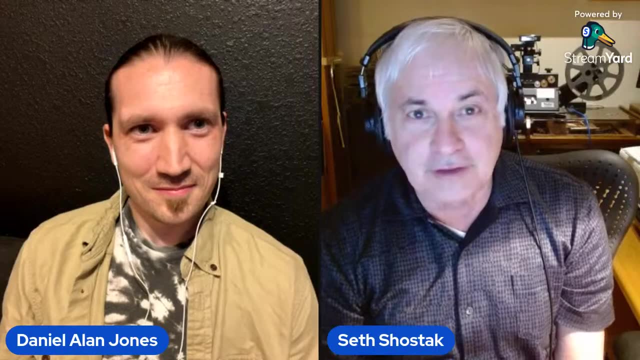 And at that point you know you're not so keen on the whole project. So the idea here was: look, we're not going to provoke them into talking to us, Let's just see if anybody's using the airwaves. That's fascinating. 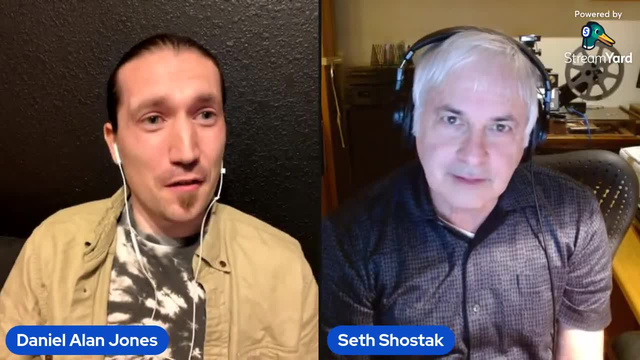 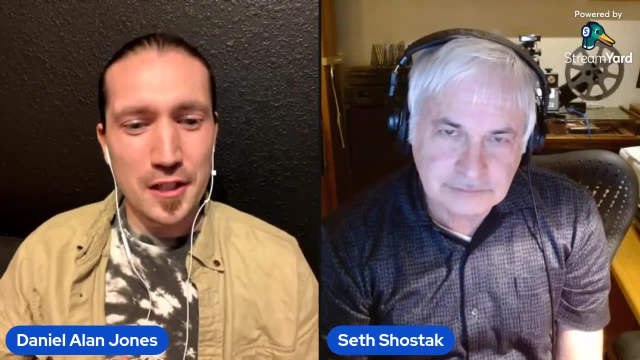 I think that it's, you know, one of the things that we see. obviously, throughout the last century, technology has made vast improvements, as you mentioned, And when it comes to the exponential factor that this technology is improving, some refer to this as Moore's law. 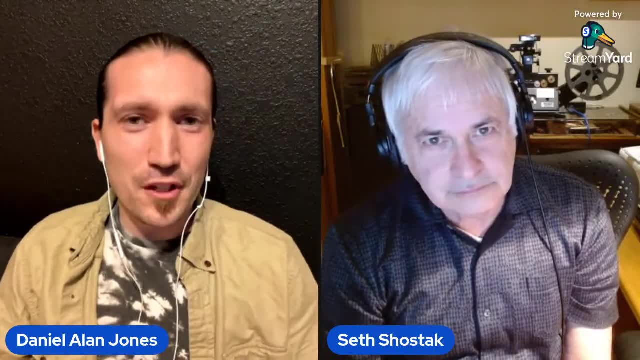 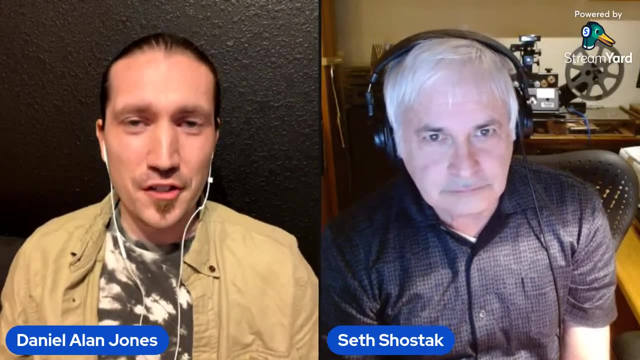 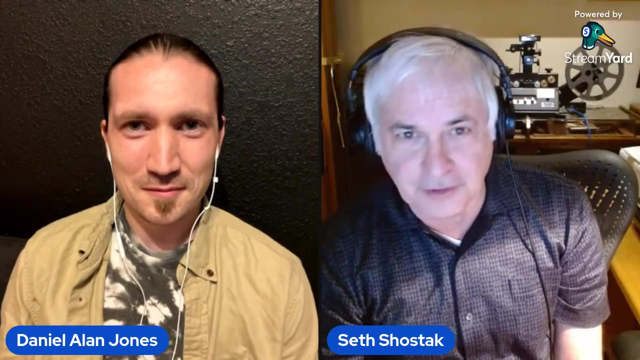 Could you describe how maybe that comes into effect with the ability for something like SETI to be able to find more or to gather more data with the advances in modern technology? Yeah well, Moore's law, named after Gordon Moore, who was one of the co-founders of the Intel Corporation. 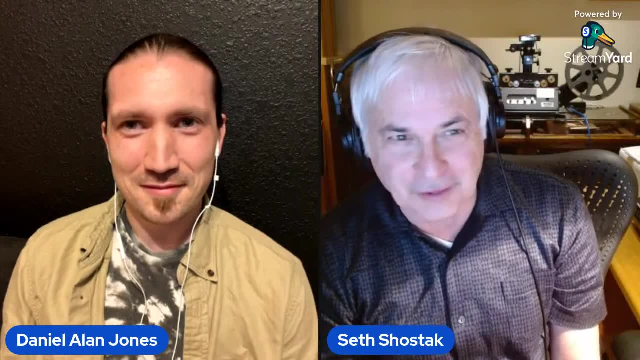 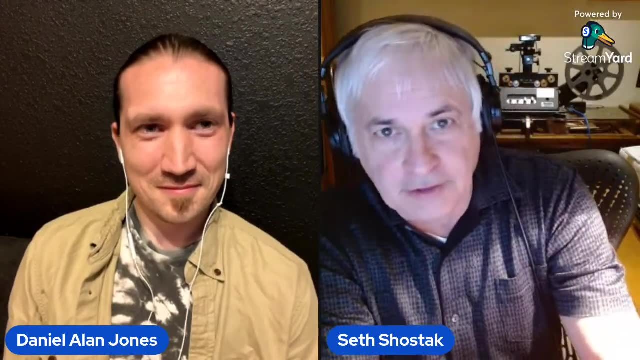 If you have a PC at home, you know you've got products from the Intel Corporation, the Intel Corporation in there, in particular the processor. But I'm speaking to you here from the Silicon Valley. We're located about an hour south of San Francisco in the lovely 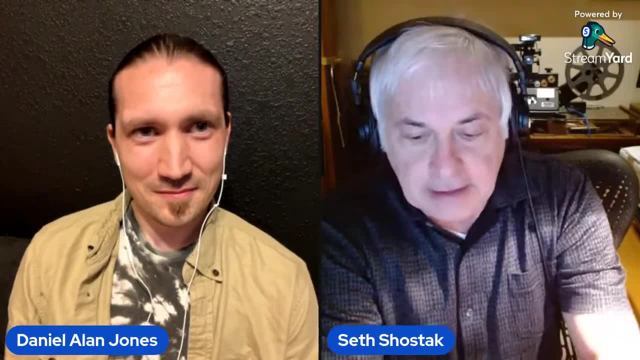 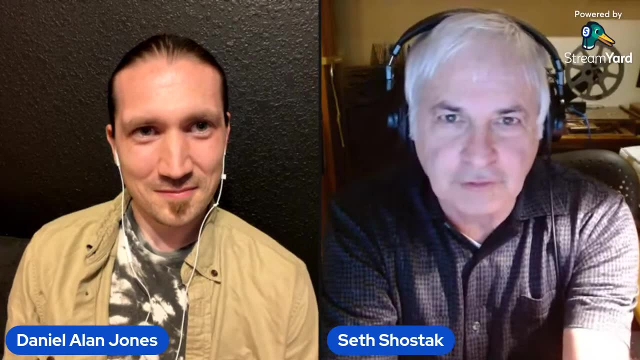 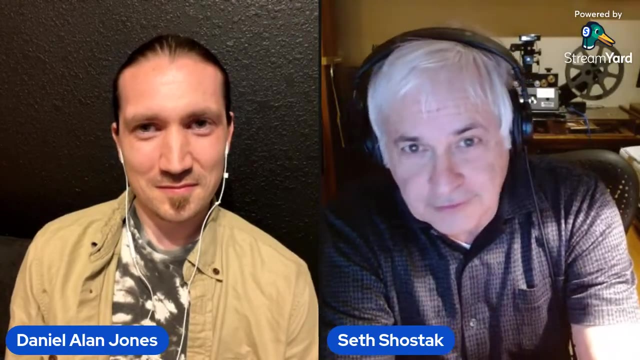 glamorous town of Mountain View, which is again the Silicon Valley. Now, in order to sell more computers? right, you need that the product have a certain degree of obsolescence. right, You buy your laptop and you know it probably still works after five years. 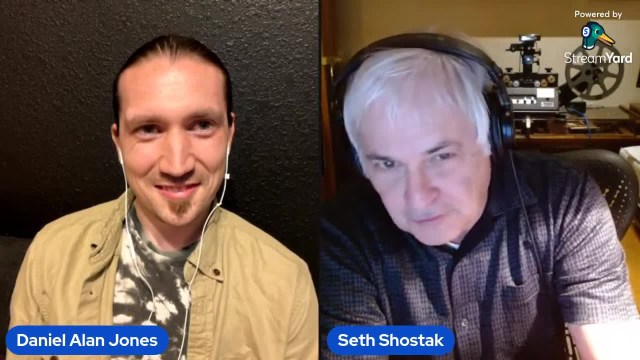 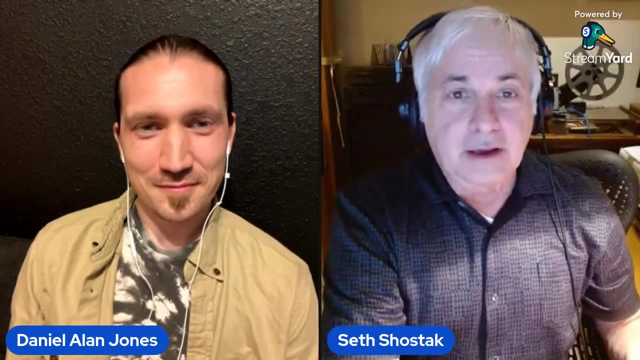 It might still work after 55 years. right, There aren't any more. I mean moving parts, maybe the fan, But I mean you know there's a very long lasting technology. It's not like your car. So, as a consequence, there isn't much incentive for you to replace your computer unless. 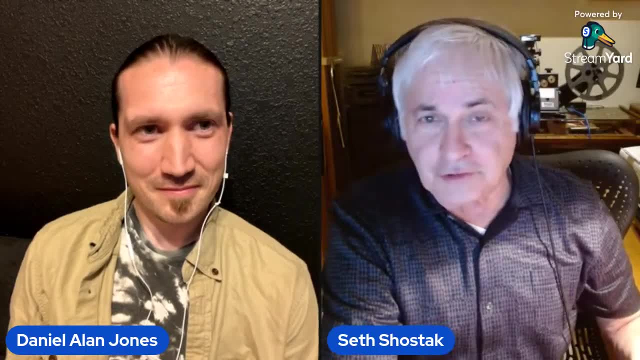 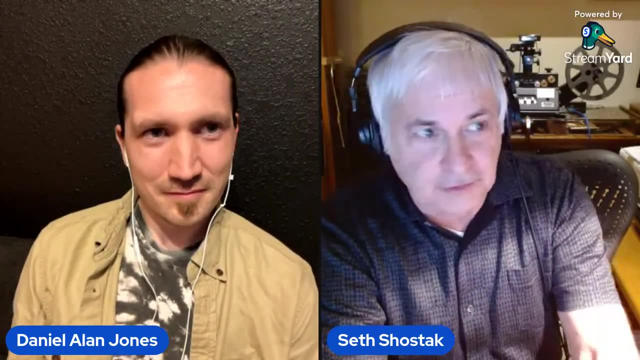 something forces you to do that, or at least encourages you to do that. And what does encourage you to do that is this rapid development of the technology here. You know these companies around here. they want to sell more chips, They want to sell more computers. 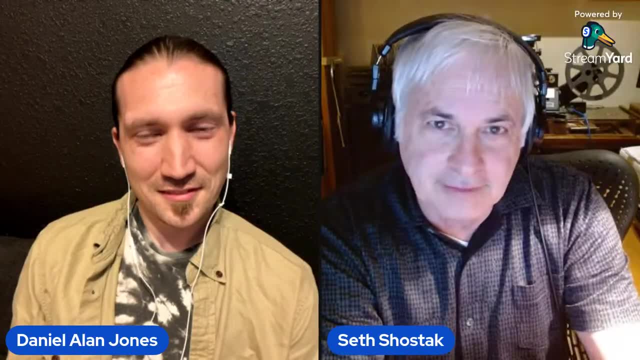 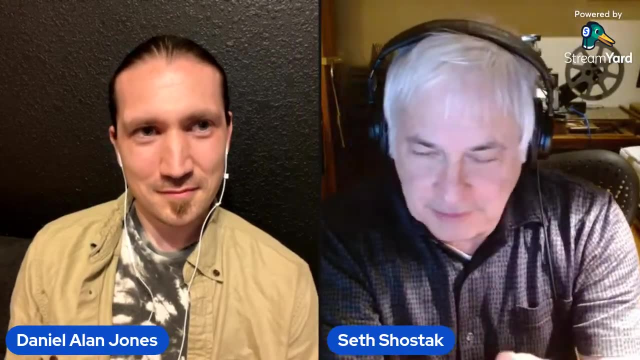 And in order to do that, they just keep speeding up the equipment the way they normally do, that It's by putting more and more transistors on the chip, right. So just more mechanism in there, if you will, And Moore's law. Gordon Moore remarked on this 30 some years ago, I think. 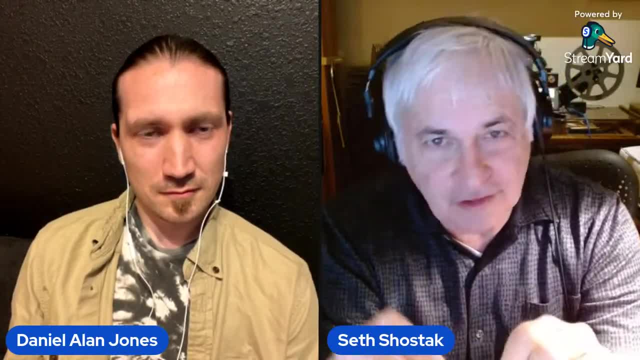 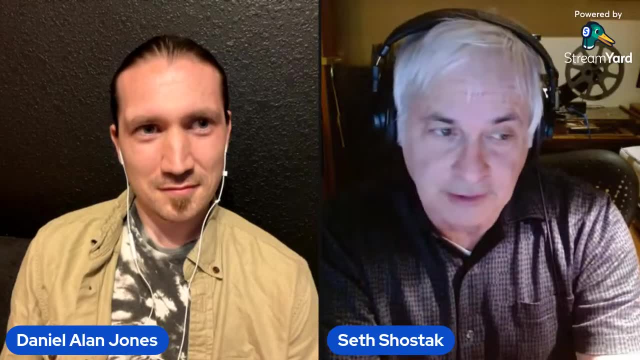 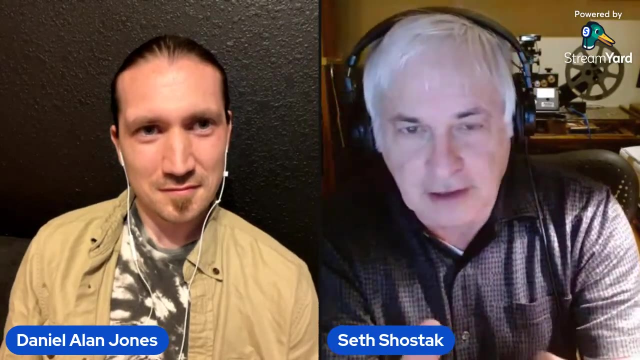 He noticed that the number of transistors on one of these chips- they're very small- was doubling about every 18 months. So that's an exponential increase, right? So every two years. say you know the speed of the computer that you can buy for any given price point, say $1,000, doubles. 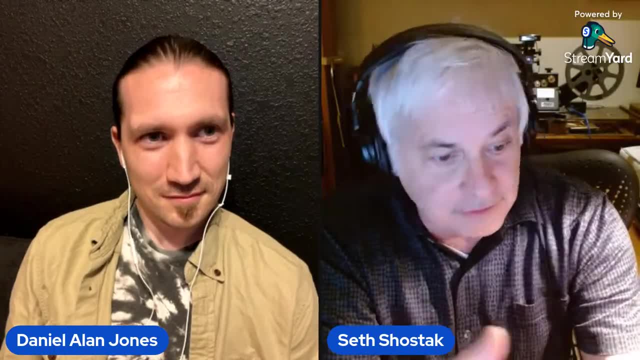 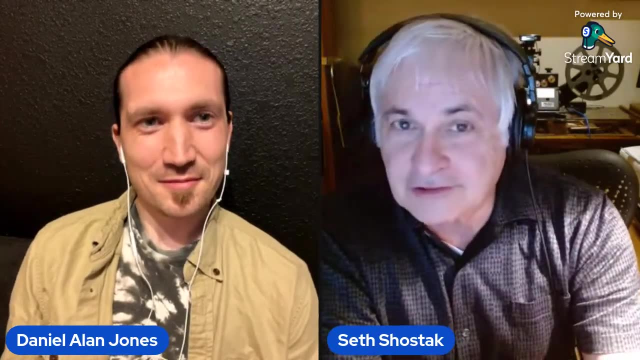 So you buy a laptop and then five years later you know it still works, You still got your software installed on it, But all the really nifty new software won't run on it because it's too slow. So you have to go out and buy a new computer. 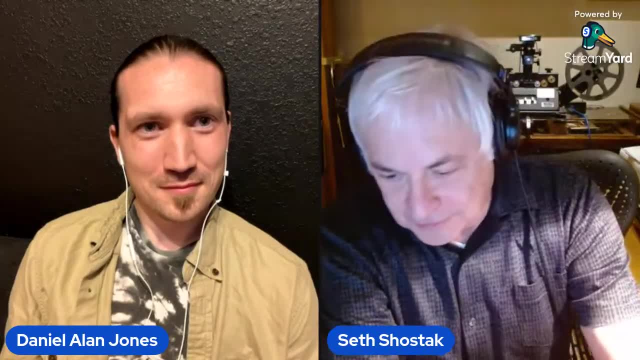 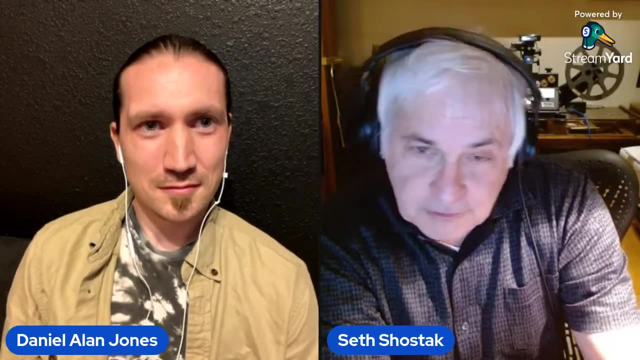 So that's the idea. That's the economic law of the Silicon Valley- Moore's law. But if you're looking for aliens, you're also using electronics and you're using a lot of computers. The consequence of all that is that about every two years, 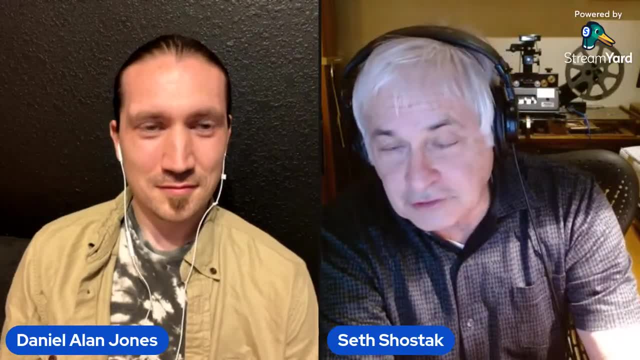 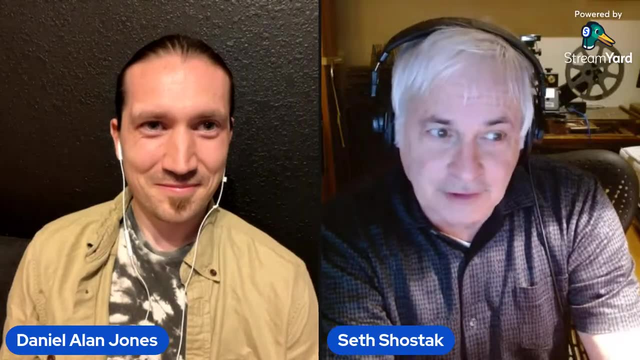 the speed of your search also doubles. So that's good news and bad news. The good news is, you know when you speed up the search you might find something a little quicker. The bad news is that you know you've got to replace a lot of the equipment. 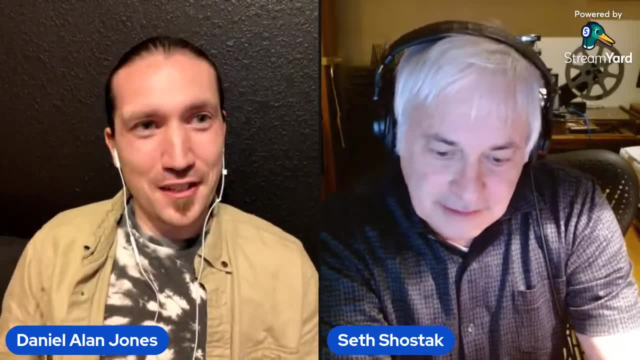 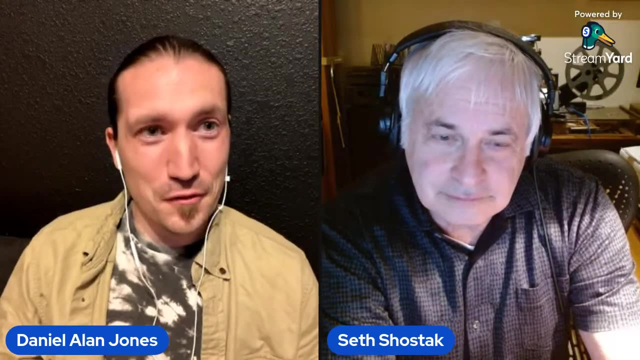 Well, it's really interesting to see how something like that can help us. You know, as you mentioned, we see that as that exponential factor might double every few months, and now that's probably changed quite a bit, with not only the timeframe. 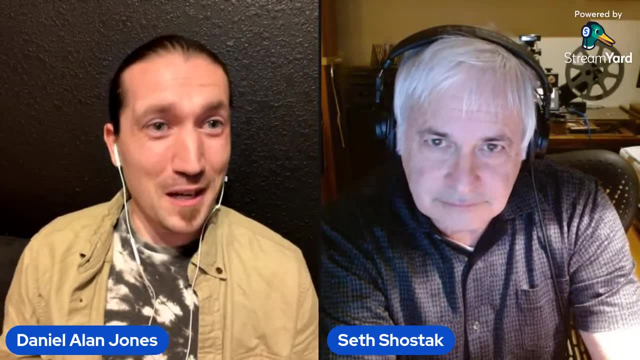 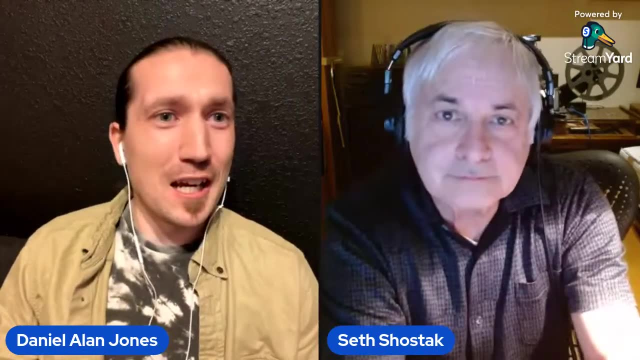 but also the materials used to produce technology and manufacture certain things as well. But when it comes to the search, it makes us wonder, and you mentioned, you know, is it a sociological type of factor when we wonder, is it safe to try to commune? 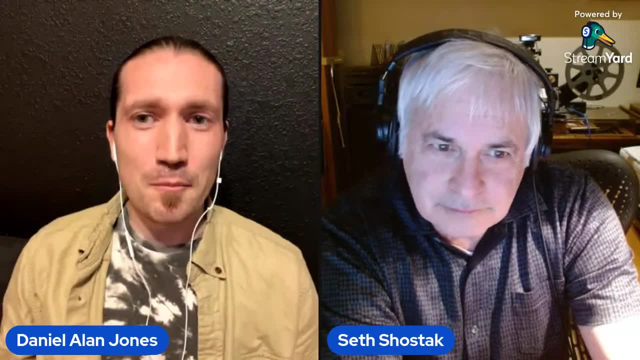 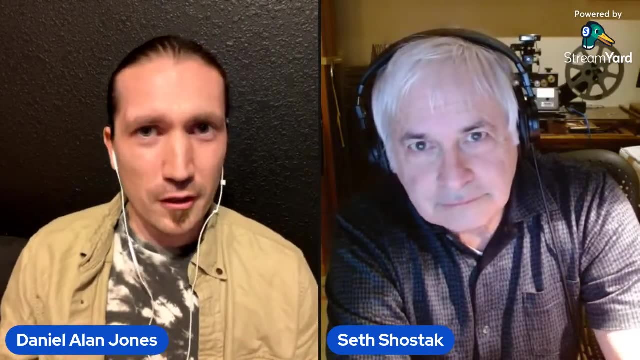 Is it safe for us to try to respond or elicit a response, And many people- various figures and those who have come forward to you know- propose various ideas. Carl Sagan was a big proponent of contact. Obviously, this is something that I think has been a big way. 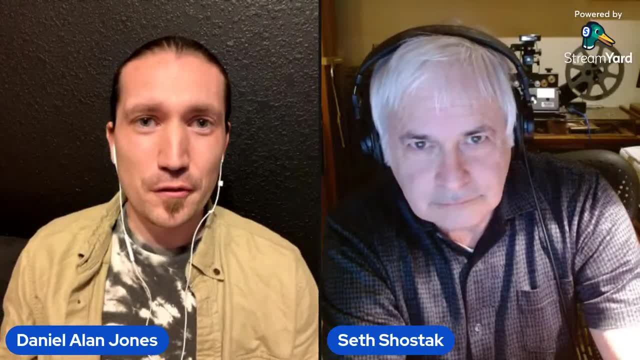 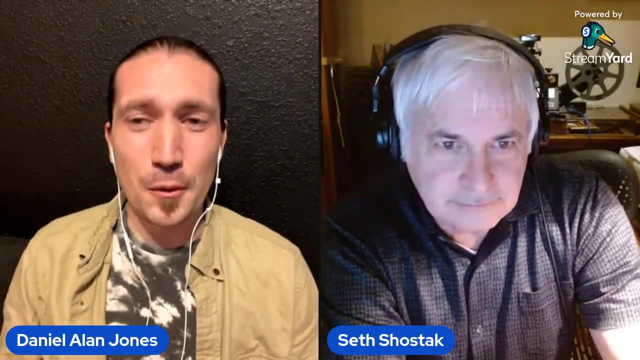 for a lot of people to know about this type of subject or this issue of connecting with other worldly civilizations. He was someone who went out there and tried to make sense of how we can find out more. But then you have other people who look at this in a different light. 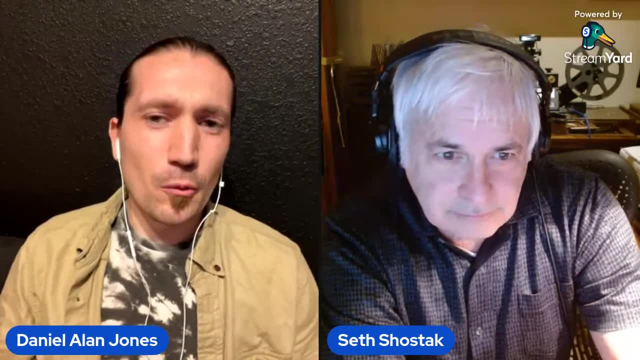 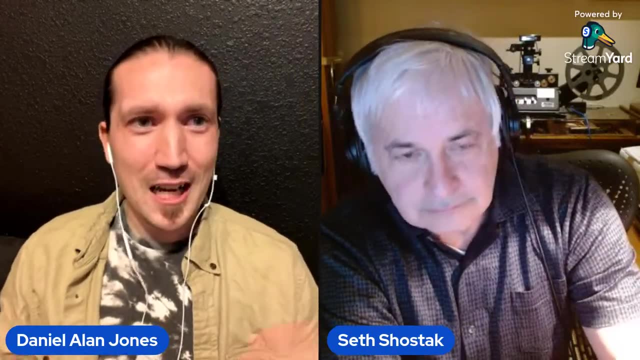 Stephen Hawking, for instance, had looked at this in a way that we probably shouldn't be trying to elicit responses that it might not turn out or bode well for us. What are your thoughts on, maybe, the dynamic between those two extremities? 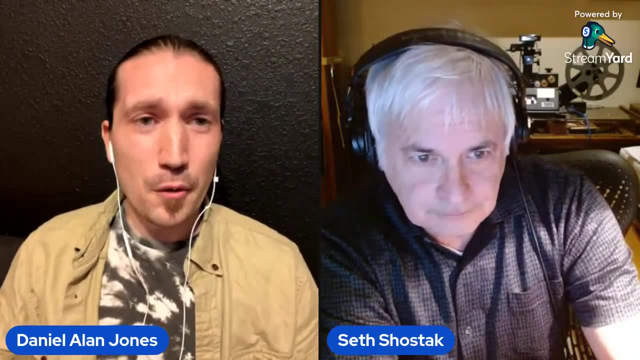 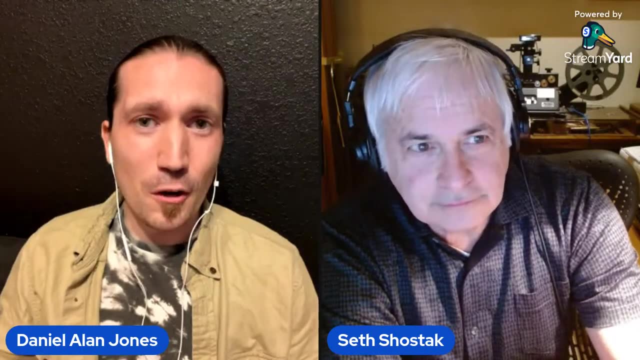 of you know, scientific figures of their caliber, both having reputable status but also having, you know, various views. maybe that are, you know, not always lining up, but help us see the real challenges that we might face in this endeavor. 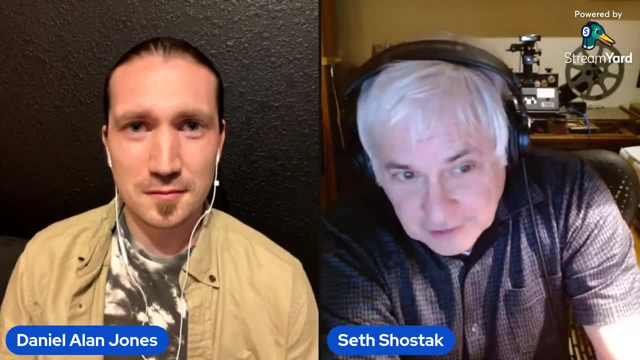 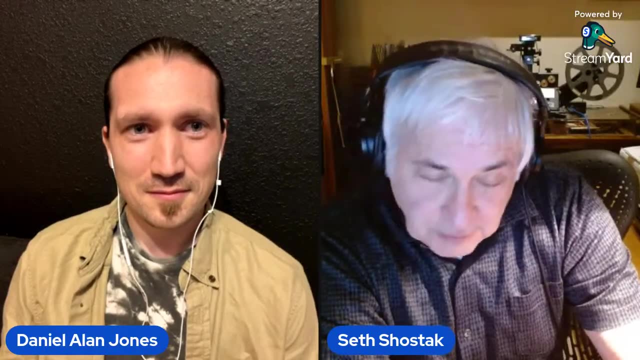 Yeah, well, look, SETI is a listening experiment, So we're only listening, We don't try to transmit anything. Now, that's primarily because if the aliens, as I mentioned earlier, if the aliens are, you know, a hundred light years or a thousand light years away, 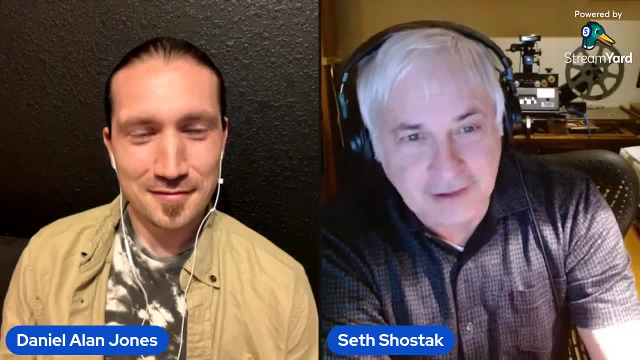 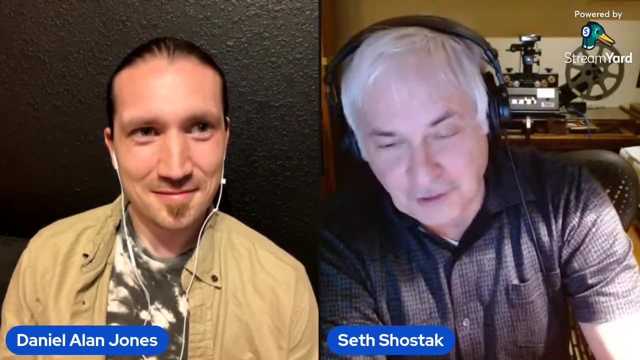 the experiment is going to take a long time before you can even hope for some sort of result, because the signal has to get to the aliens and they have to get their response to you, even assuming they're going to give you a response, right? 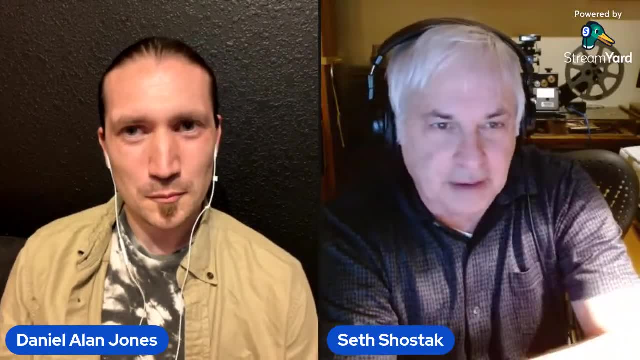 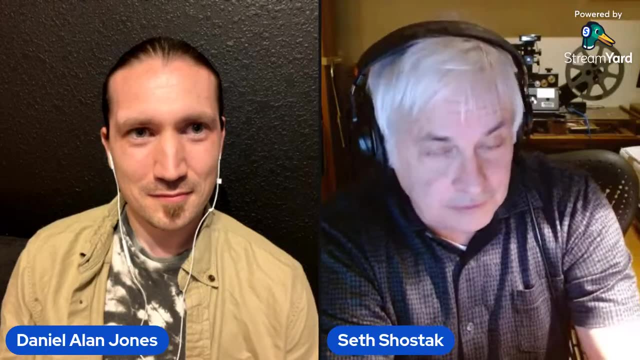 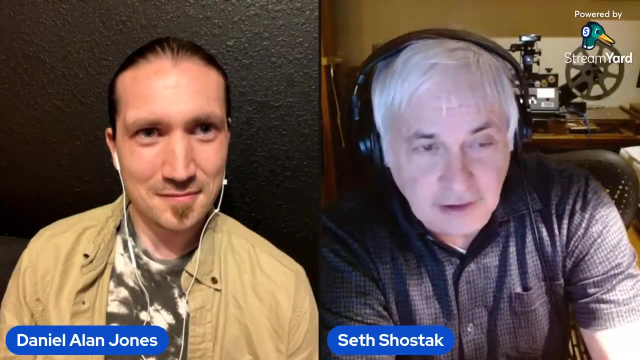 They might be on summer vacation or something, and they didn't even pick up your transmission. So I mean, there is that. But in addition to that, there are other people who say: look, just as you suggested, Daniel, that letting the aliens know where we are by sending out a signal might not be a good idea. 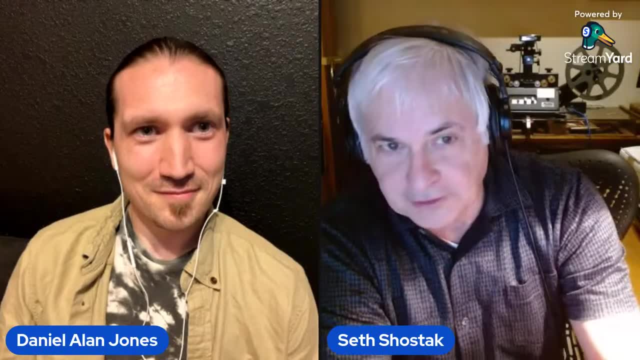 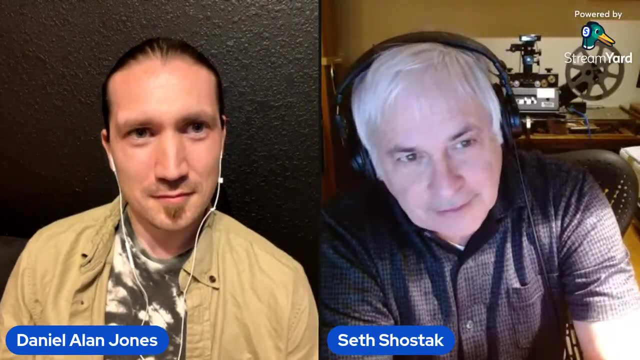 You don't know whether they're hostile or whether they just like to read poetry all day long. I mean, you don't know. So there are people who advise against broadcasting. Now you know that makes for an interesting story, sort of. 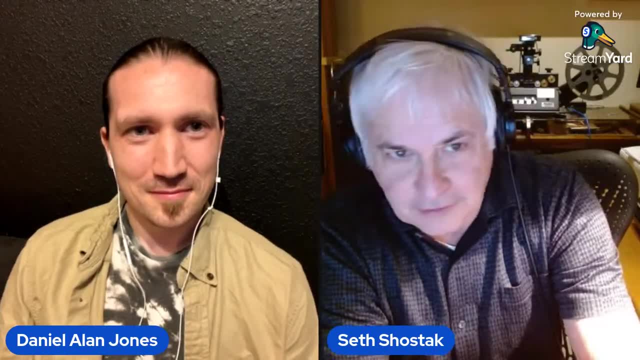 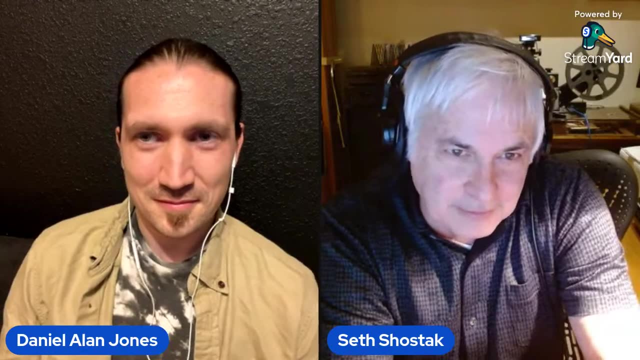 but it's kind of irrelevant because to begin with SETI doesn't transmit. But beyond that, not only not transmitting, but because because of the timescales involved it wouldn't make a whole lot of sense for us to transmit very much of anything. 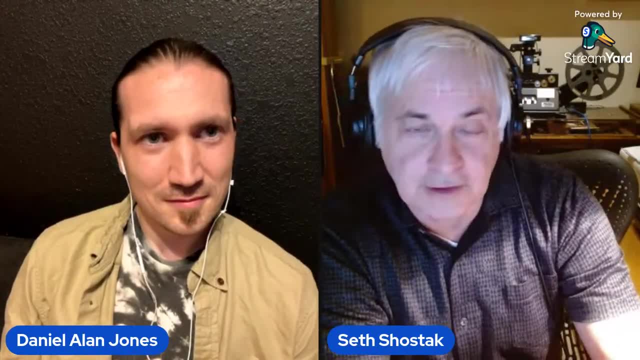 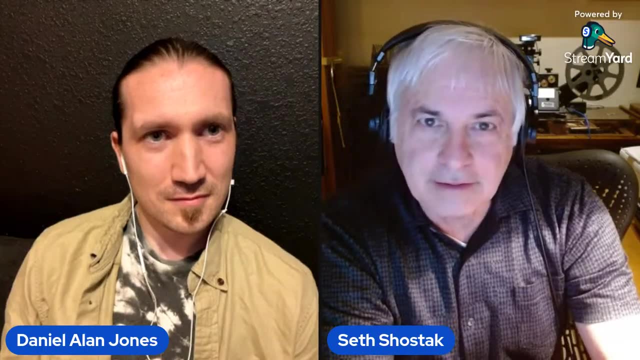 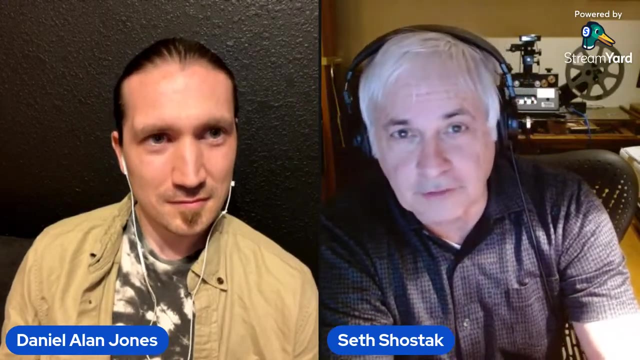 Now, not everybody agrees with that. One of the guys who used to work at the SETI Institute is actually trained in psychology, I believe, And you know he's interested in actually transmitting simply to alert the aliens that were here and maybe encourage them to try and get in touch. 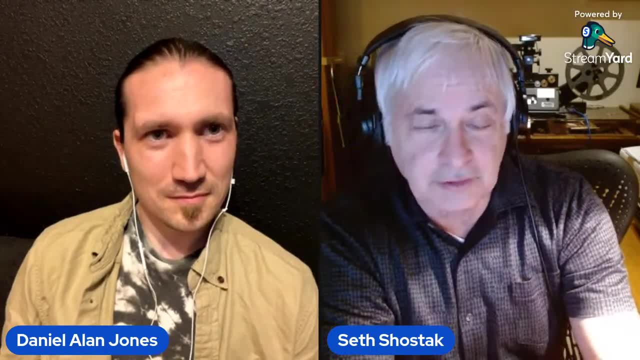 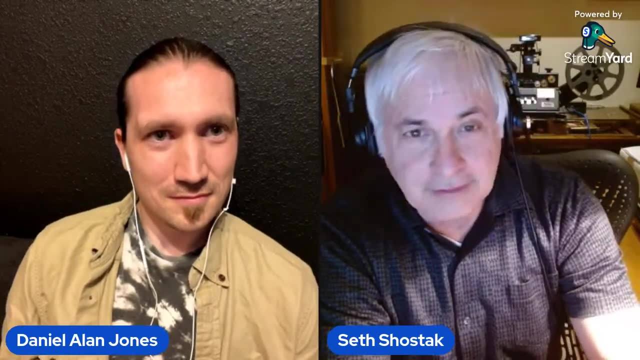 That might work. It depends on whether the aliens have any interest in doing that. But in general SETI experiments do not transmit, They're just listening And there's no danger in listening. I mean, you tune in your favorite DJ on your car radio. 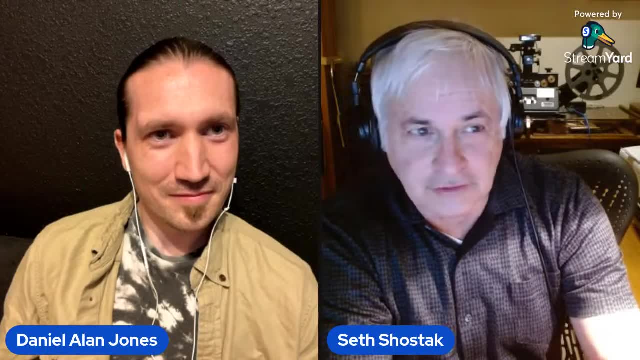 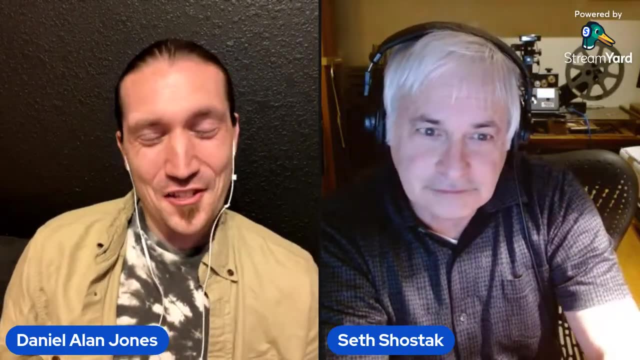 and there's very little danger that that DJ is going to jump into the car and give you a hard time, because obviously the DJ doesn't know you're listening Right? So it's one of those things where I think that it's. 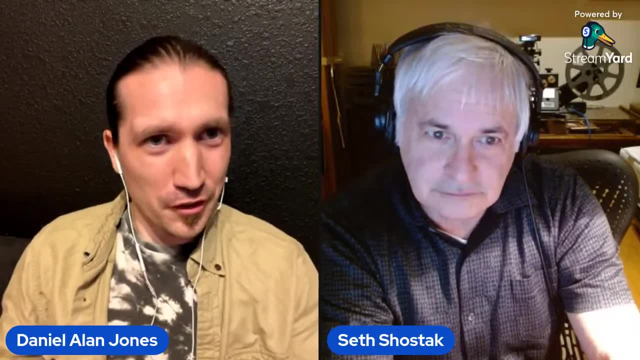 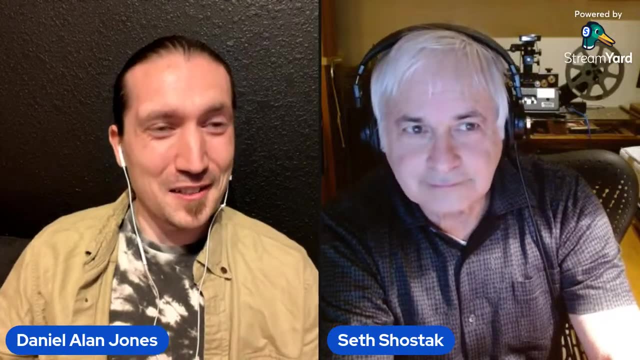 depending on the direction of the focus of a particular group organization. as you mentioned, with SETI it's not concerned as much with transmitting, you know, and receiving something that would be a communication. I think that would be fascinating to consider how that would play out. 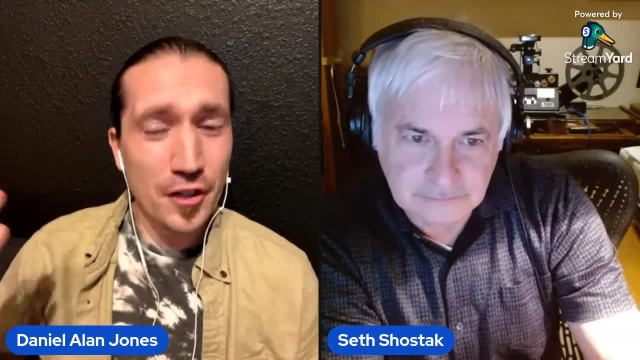 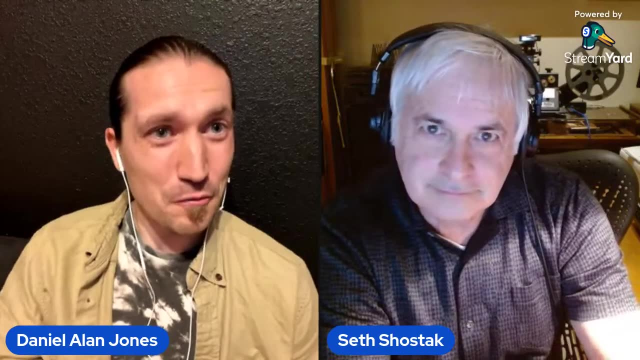 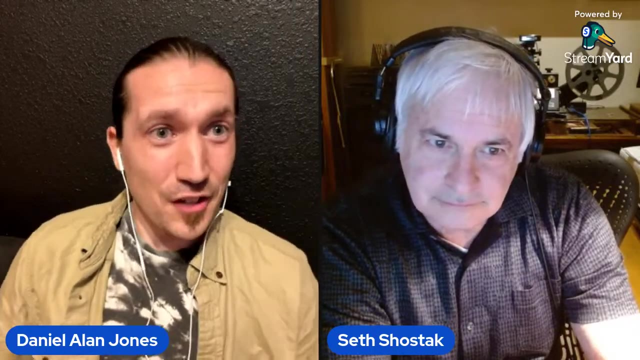 Obviously, it's something many wonder about how that would take place, But to just find signals that represent technological sophistication beyond just in many ways, as you've put and suggested in your work- microbes or something that's not really considered intelligent And with the work that you've published regarding astrobiology, 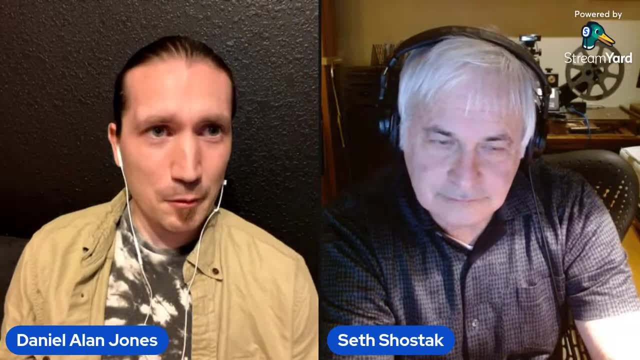 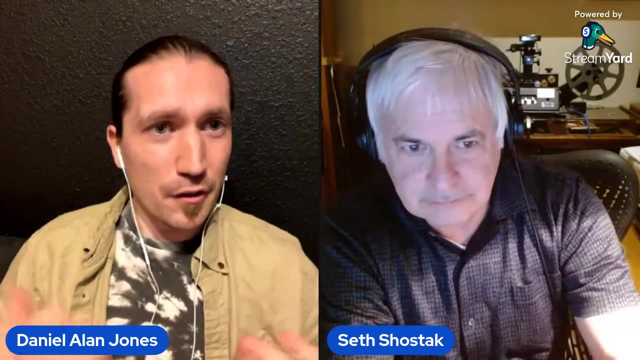 we find that there may we find that there may be many planets that are habitable but might not necessarily have intelligent life, but could be very much like what we see here with the fauna upon Earth, And that's something I think it's important for us to distinguish is that 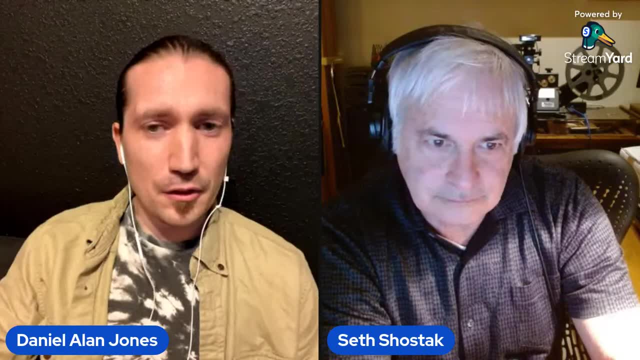 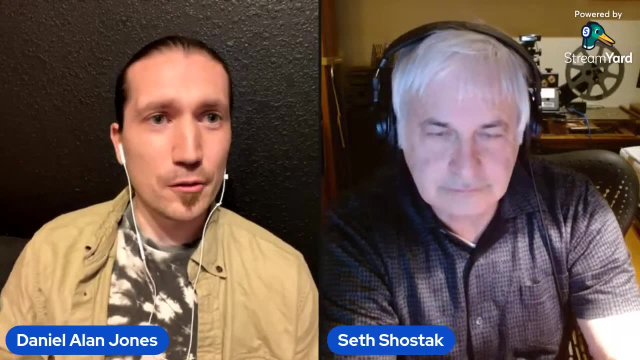 again, you're not necessarily looking for just the life itself, but if there are advances in any of those life forms that have reached the scale of being able to communicate and transmit frequencies. And so, when it comes to this, there are a lot of ways that people have. 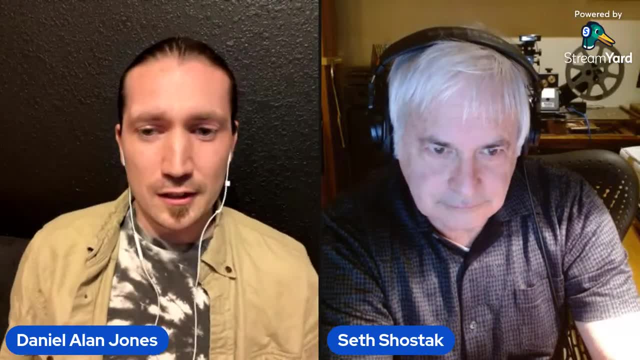 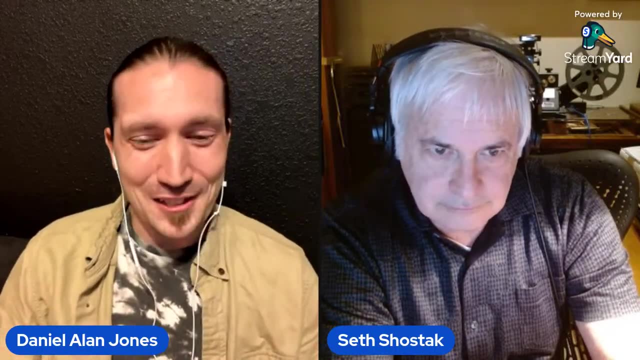 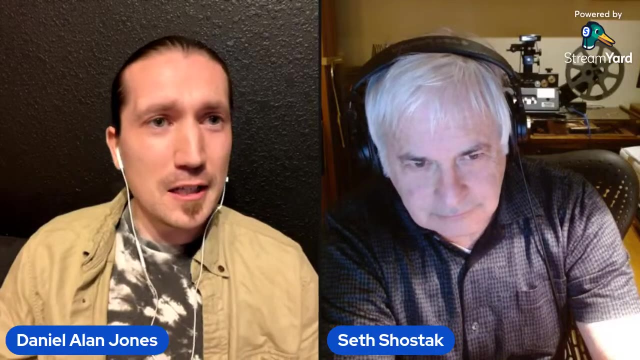 considered how to enumerate the groups out there- And you mentioned earlier Drake- And what I'd like to do now is throw some concepts at you in hopes of you sharing a little bit about your impressions on what these ideas are, how they are applied scientifically. 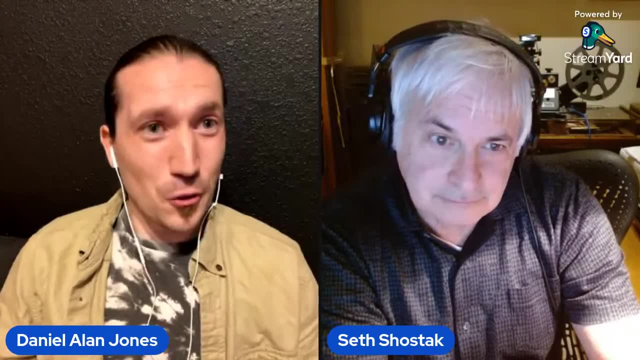 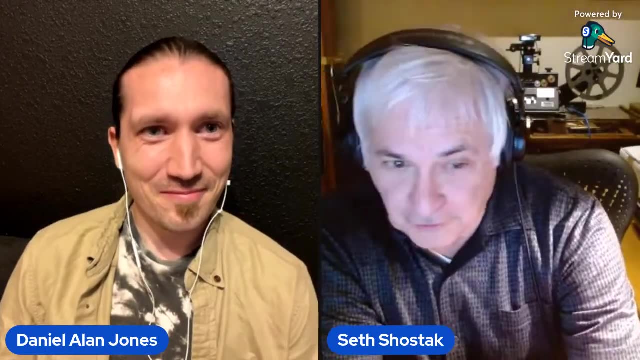 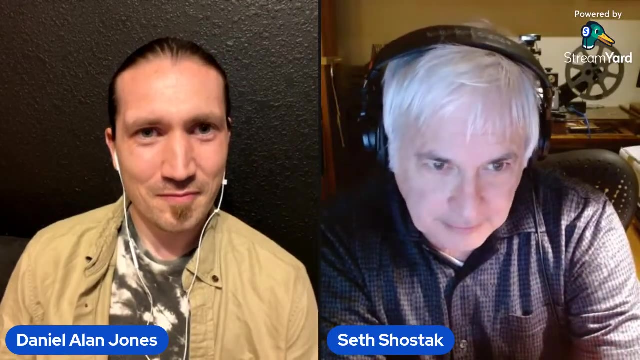 and maybe their effectiveness, The first one, of course, being Drake's equation. Yeah Well, Drake's equation, First of all. who was Drake Drake? his name is Frank Drake, Frank Donald Drake, And he actually did the first modern SETI experiment. 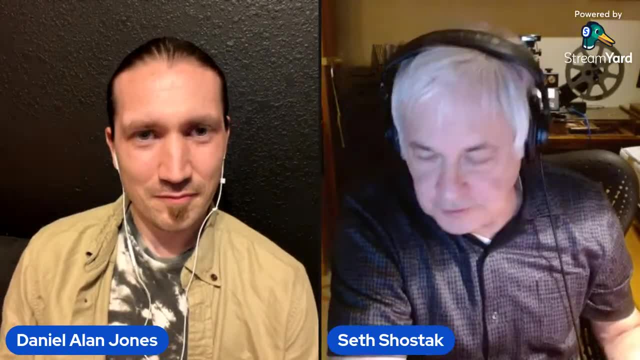 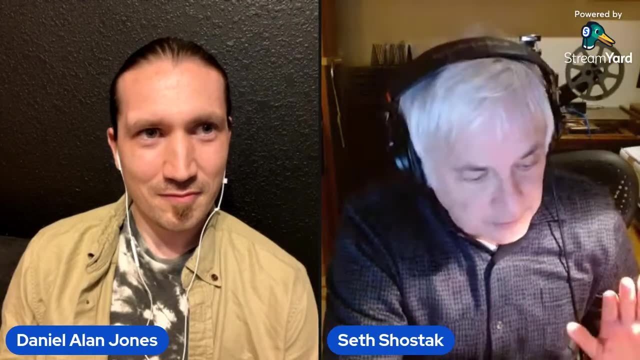 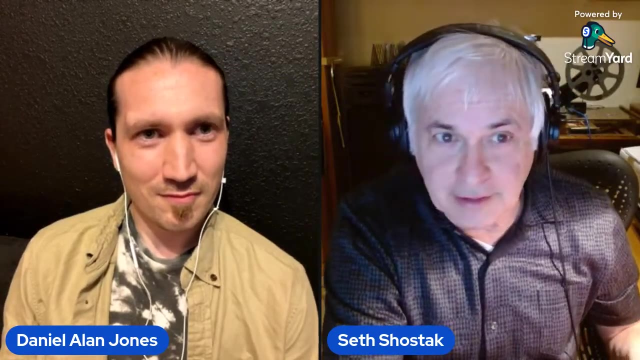 He had taken a job after getting his graduate degree from Harvard University. It was 1960. He took a job at the National Radio Astronomy Observatory, which has got its telescopes- or at least at that time had all of its radio telescopes- in a place called Green Bank. 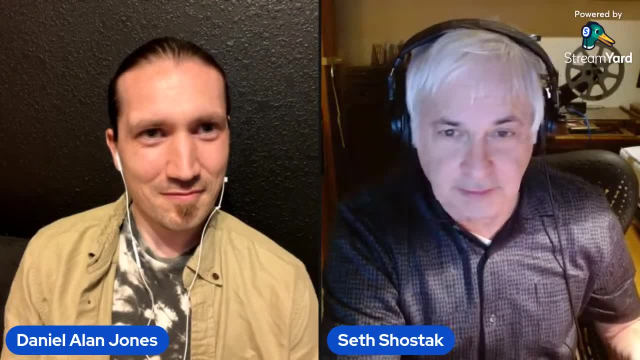 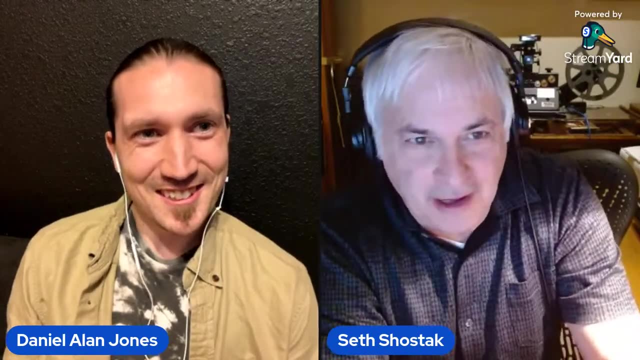 West Virginia, And it wasn't because the cuisine in Green Bank was set Exceptional, It was that not many people lived there. As a consequence, it was radio quiet. So that's what you want If you're building big antennas and trying to hear noise from the cosmos. 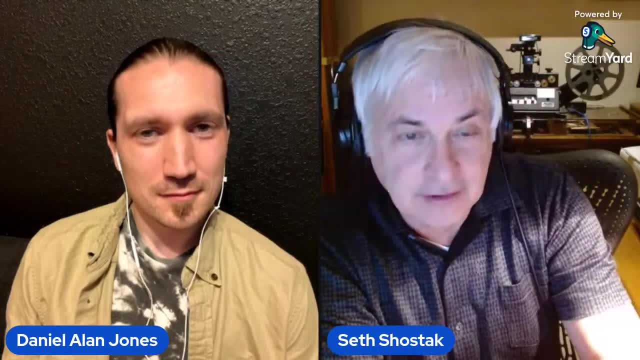 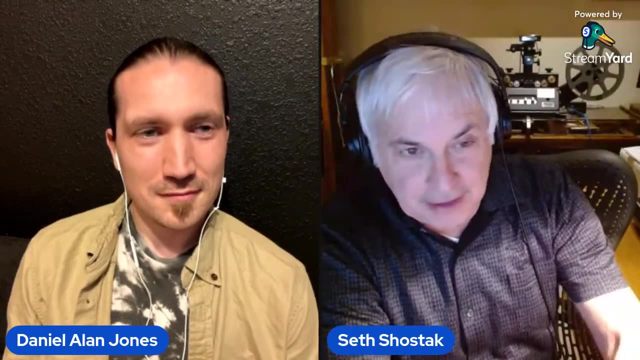 Not SETI noise. It wasn't built for that But nonetheless they had just purchased sort of an antenna kit and put that together. In 1960, there was this antenna that was well, it was like 80 feet in diameter. 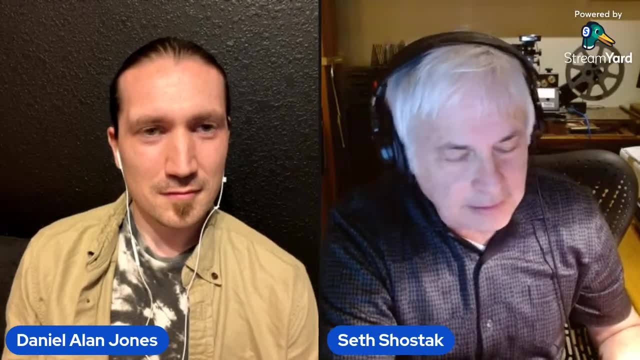 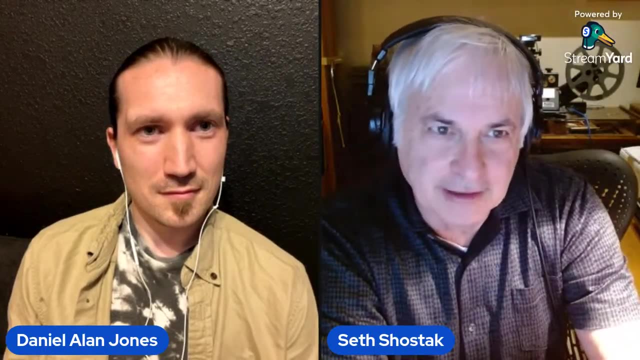 Something like that, 25 meters, I believe, And the director of the observatory, you know, had this shiny new antenna. He also had a shiny new employee, Frank Drake, And he said to Frank, look, think of something to do with this thing. 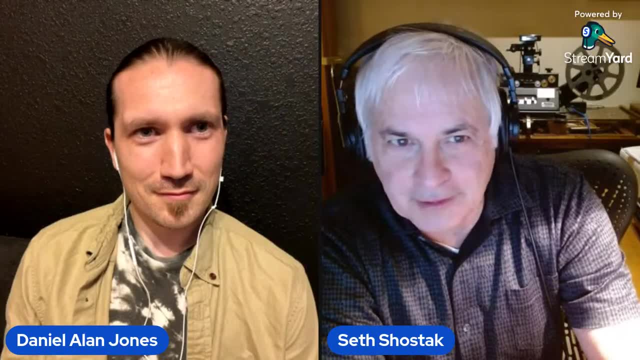 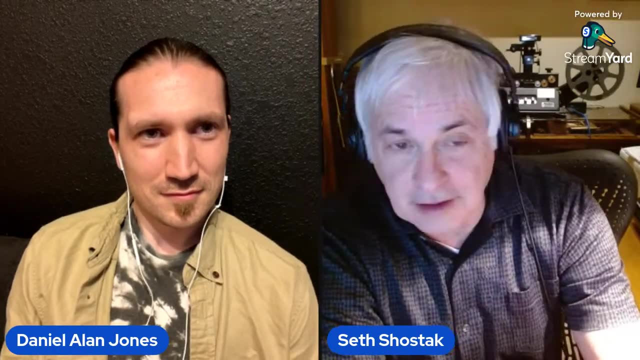 And so Drake did something that he had always wanted to try- because, you know, he was a fan of the idea of life in space and science fiction stuff like that- And he thought: well, I'm going to point this antenna at a couple of nearby stars. 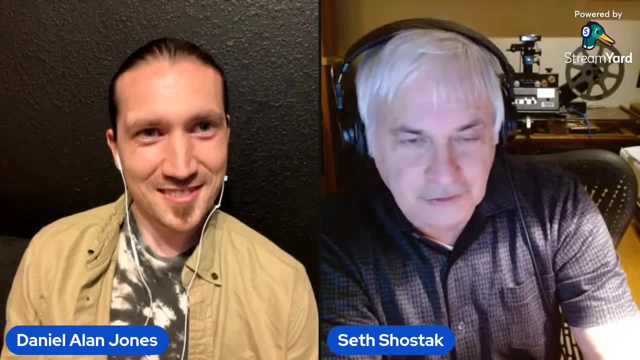 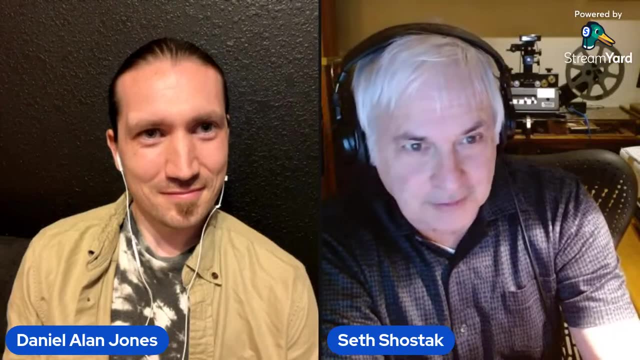 and hope that one or the other or both you know also have planets, and some planets with a Broadcasting Society on it. He called it Project Osma, based after Frank Baum's book, And he spent two weeks on this project. That's all very short. 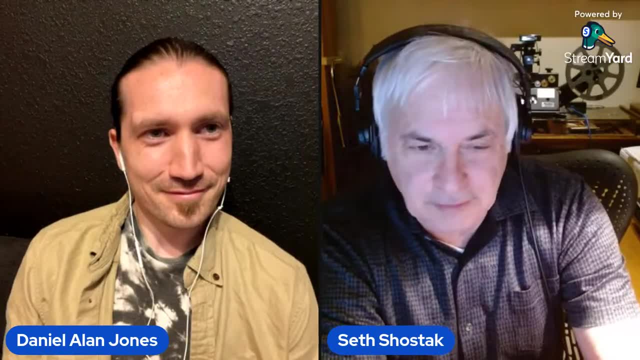 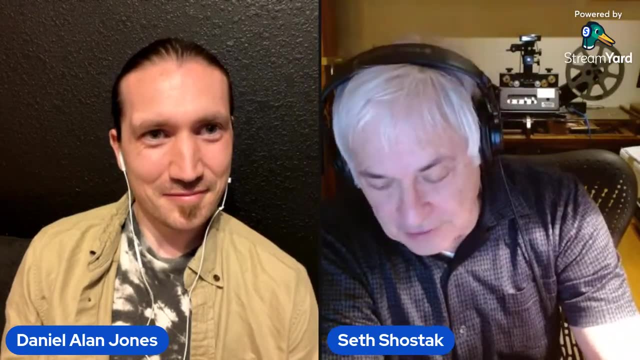 He didn't buy any equipment, didn't really have to. He tried to keep the whole project very low budget. So it's not to antagonize anybody. And he didn't find the aliens, But everybody took a tremendous interest in this and, as a consequence, 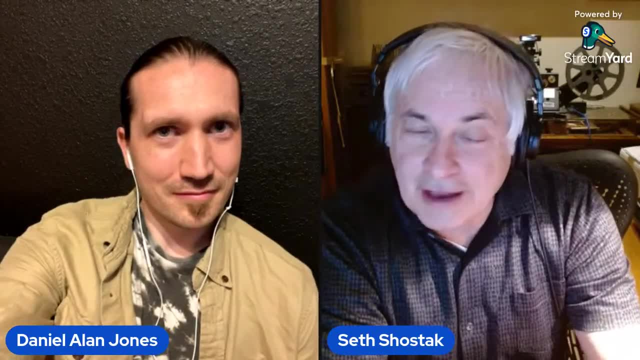 unwittingly, Frank Drake had started the whole project and, as a consequence, unwittingly Frank Drake had started the whole project, had started the whole project, whole science of SETI, by doing this first experiment And it began, as I say, in the 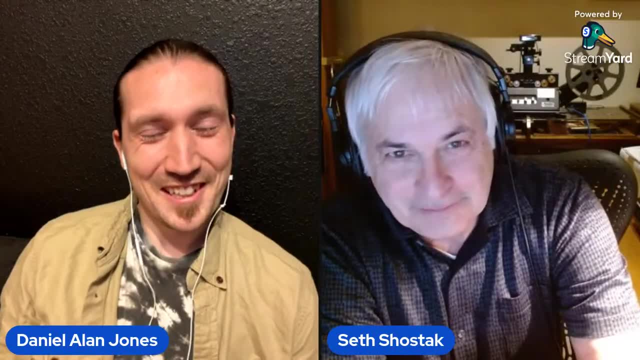 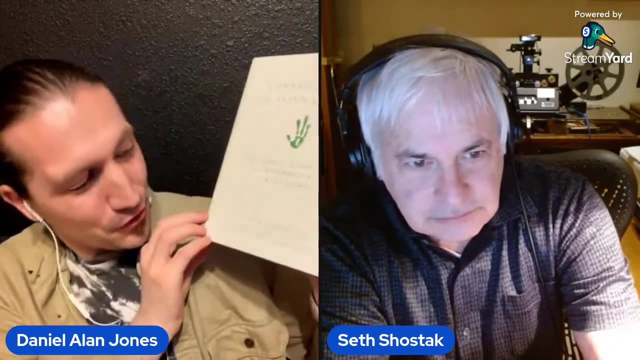 hills of West Virginia. Excellent, And I think that's something that you know. as I mentioned earlier, it's wonderful to see he wrote this forward to your book. I think it's impressive to know that he's still around- He's still considered a pioneer of this work, and that you're 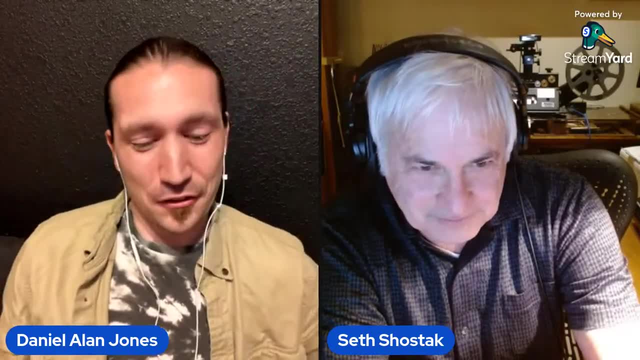 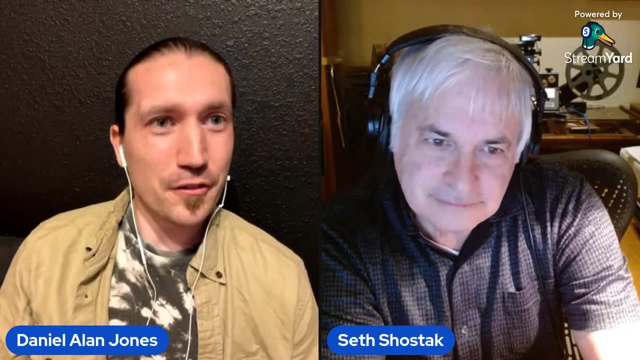 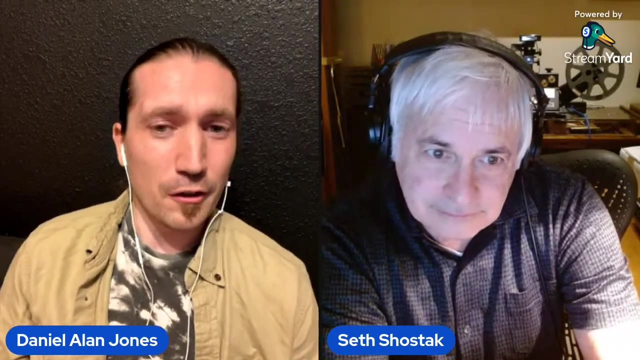 continuing that effort in many ways as well, and honoring that legacy And to precede that in some way. there was someone who came before, who this has been attributed to, but may claim that this is something that has been espoused for many years, even prior, but the Fermi paradox. 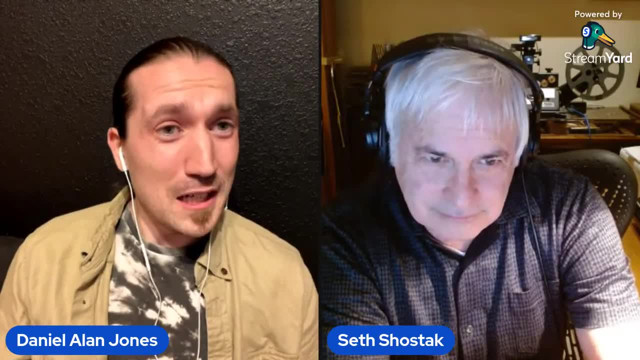 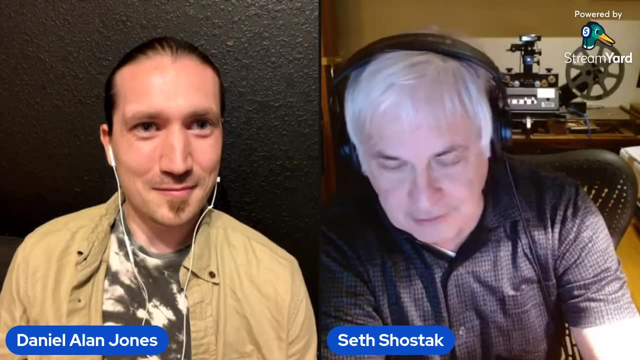 Tell us about what that implies and what that really means for us. the Fermi paradox? Yeah, Well, first off, let me mention in passing that, unfortunately, in passing, Frank Drake has passed on. Last September he died, which was 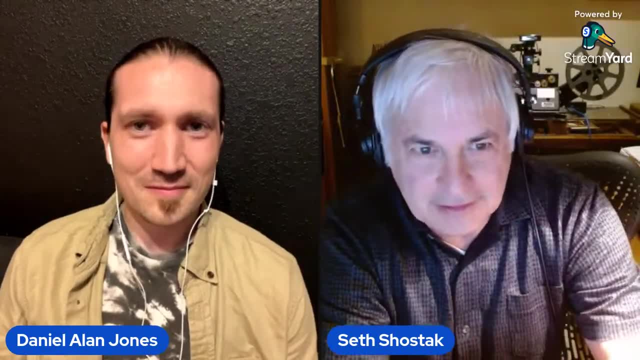 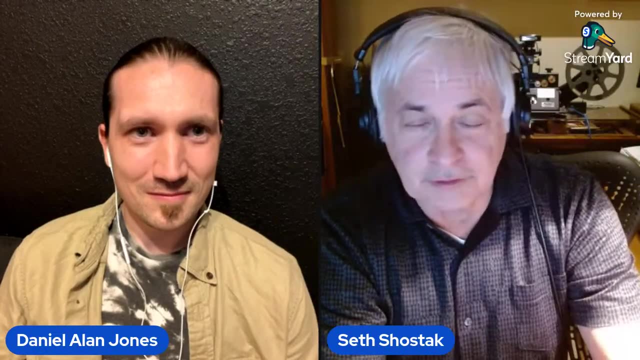 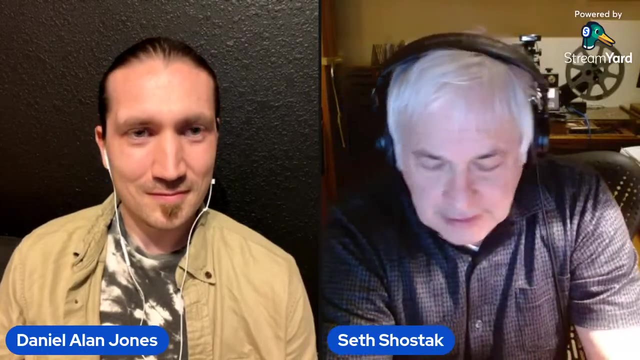 you know, very sad for all of us who knew him. He was, you know, he was a real pioneer, Actually he really was. But the Fermi paradox was named after the Italian-American physicist Enrico Fermi. And Fermi didn't do any SETI work, but he was sort of interested in it, You know. 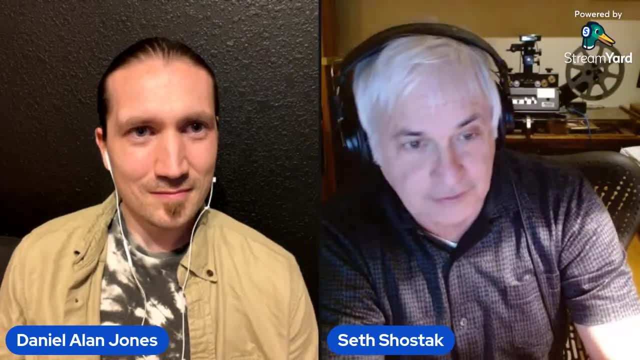 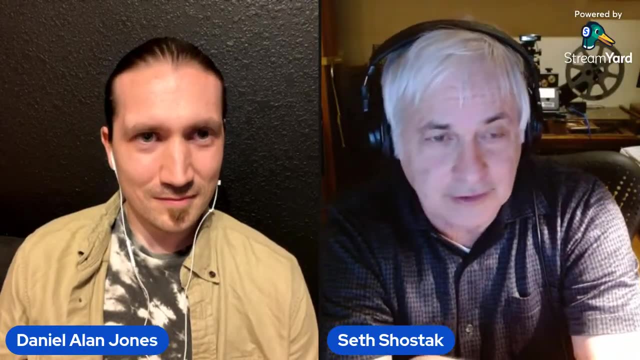 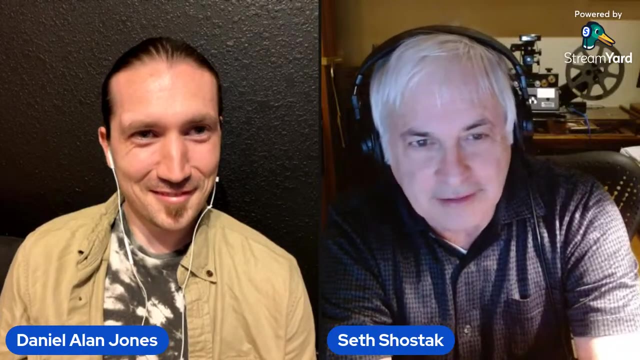 it was a novel idea at the time that he was thinking about it And he was working at the laboratories Los Alamos in New Mexico actually, And at a lunch, you know, he just he was taking some bites out of his sandwich And he was dining there with a. 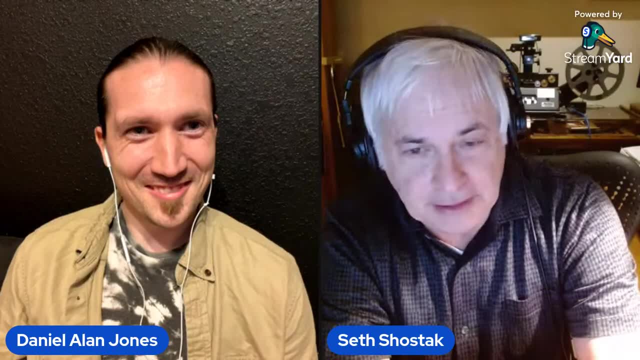 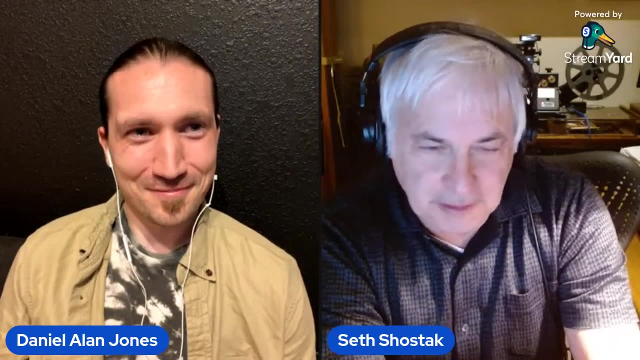 couple of other physicists from the lab, And he just said so. where is everybody? You know, Fermi is very, very bright, as were the people that were having lunch with him, And he didn't really need to explain very much what he meant by that, But what he meant was: look if the universe 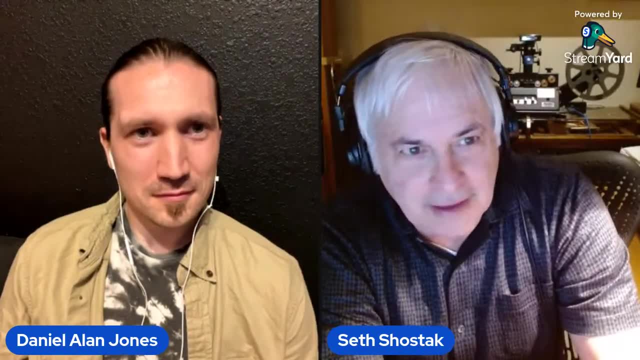 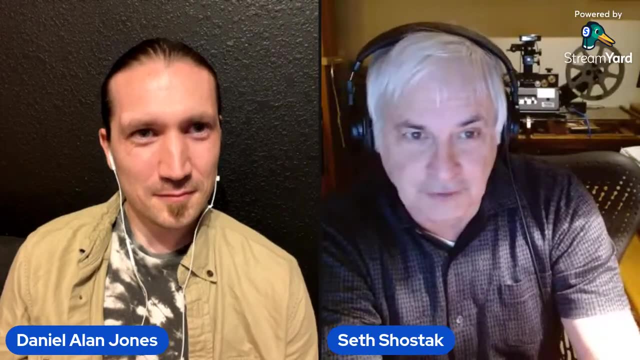 is chock-a-block with intelligent beings, why don't we have any evidence that they're there? That's what he was asking. It's a good question, even today. So the paradox that Fermi was pointing out was: well, we think that there. 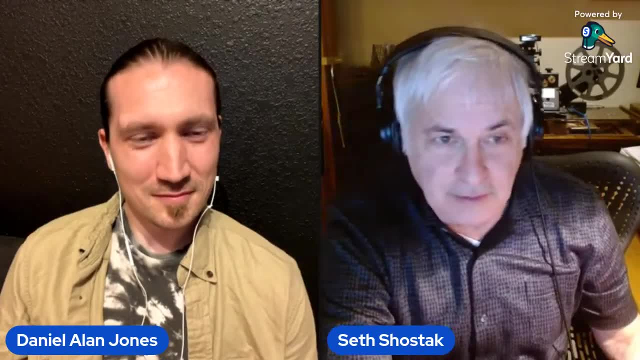 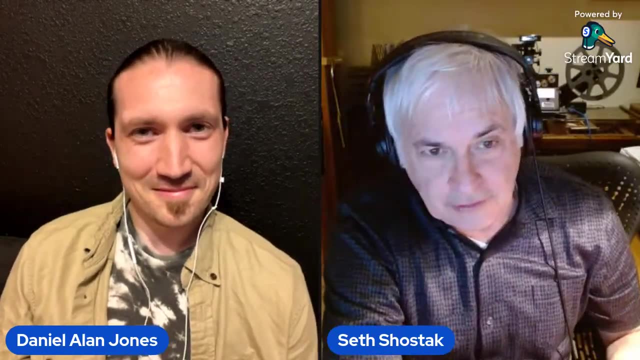 I mean, you know, there are hundreds of billions of star systems in the Milky Way galaxy. We can see a couple of hundred billion other galaxies, each with a couple of hundred billion star systems. So there's plenty of real estate, and yet we don't seem to have any evidence that anybody's 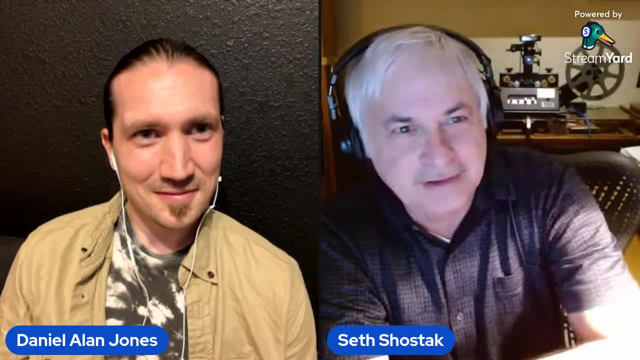 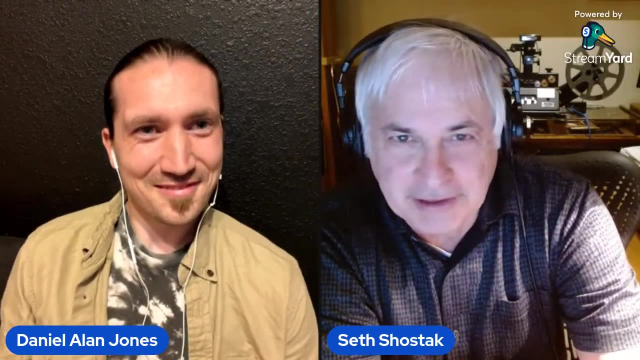 in that you know vast cosmos, And so that was his question: Where is everybody? It was just a lunchtime provocation for the people he was chowing down with, I think, And it's a really valid sentiment. As you said, even today people wonder if the 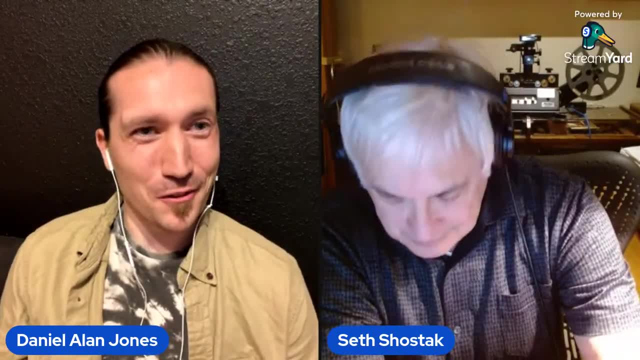 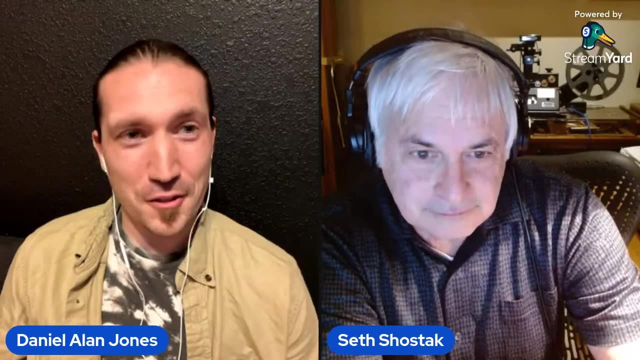 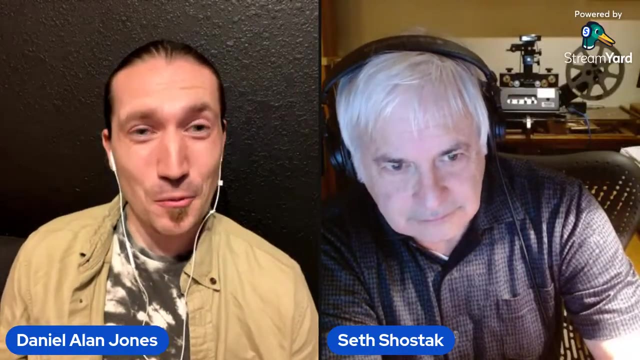 universe is teeming with life. if our scientific and cosmological models are accurate, then it seems like, if not anything else you know, a fraction of those estimations should still show that there should be plenty of it, as you put in the real estate, And I think that's curious to. 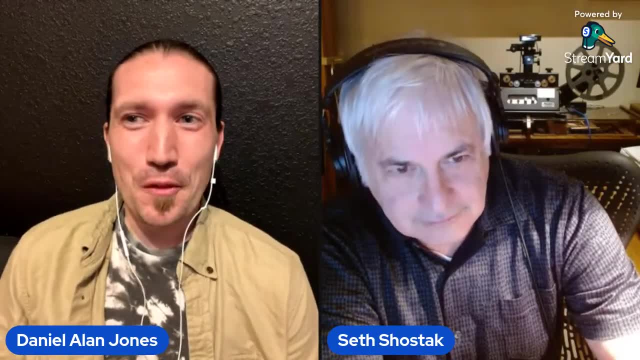 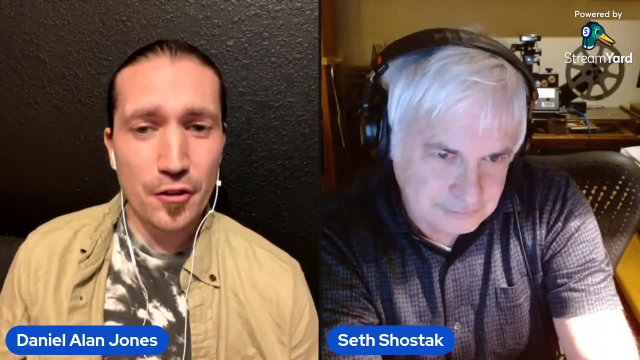 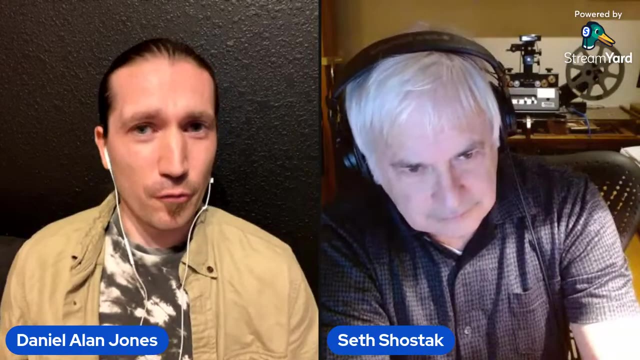 where is everybody? Where are they right? So you know. that being said, many people have also considered that maybe there are explanations for this issue When it comes to, some of those people have proposed some of the ideas pertaining to the zoo hypothesis or the dark forest. 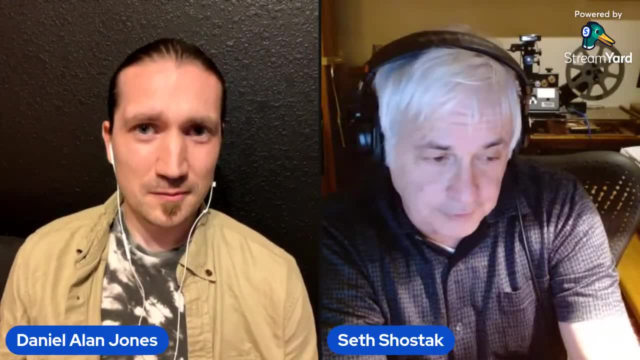 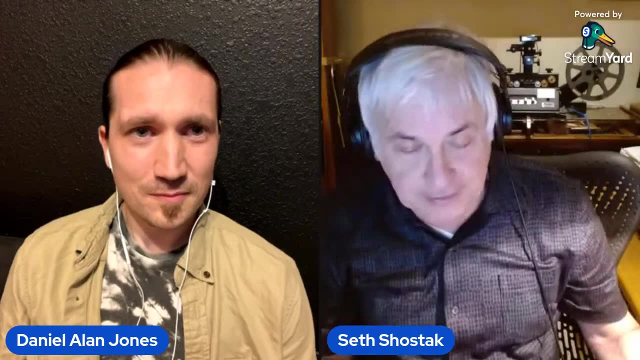 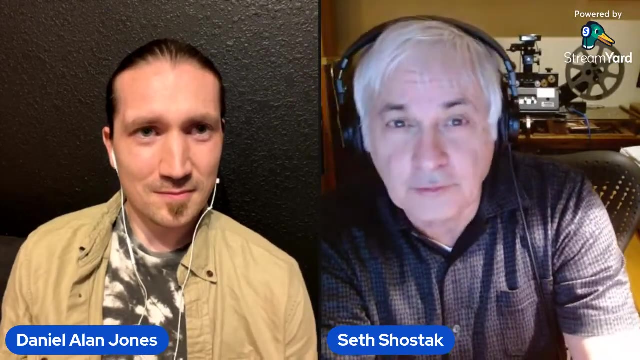 What are your thoughts on these concepts? Well, first, for those who don't know what they are, the zoo hypothesis. it tries to explain the fact that we don't see anybody, or hear from them, or get any other clues of their existence, simply because we're an exhibit in a cosmic zoo. 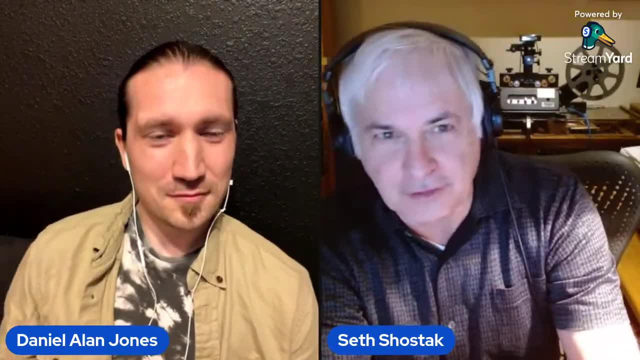 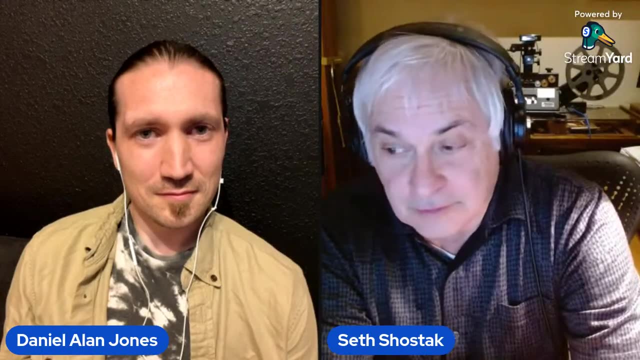 right That you know we're the new kids on the block. Homo sapiens has only been around for about 300,000 years thereabouts. There are other societies out there that could well. I mean, the universe is billions of years older than the earth, So there could be societies out there that. 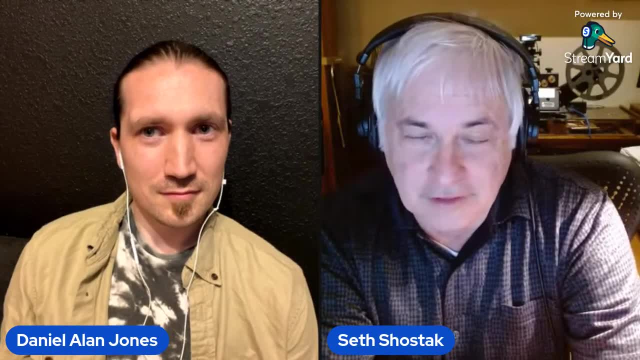 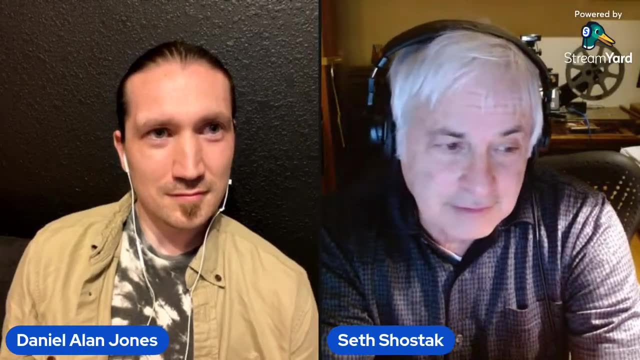 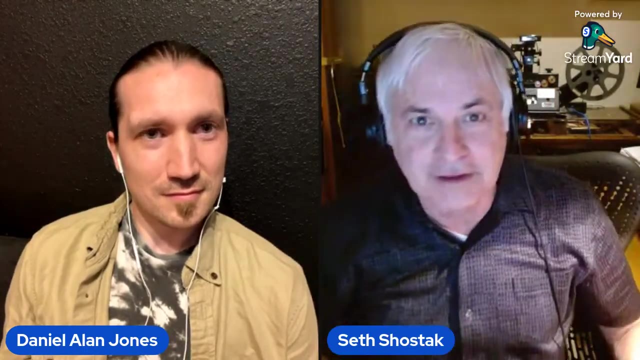 are billions of years more advanced than we are. So we're kind of the new kids And you know that thought that we're the new kids you know could lead them to keep hands off us because they don't want to. It's like the prime directive they used to have in Star Trek. 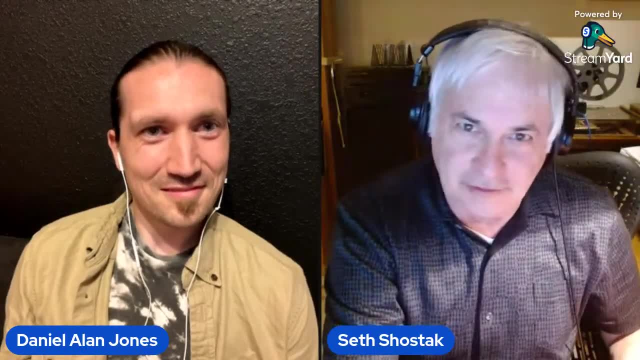 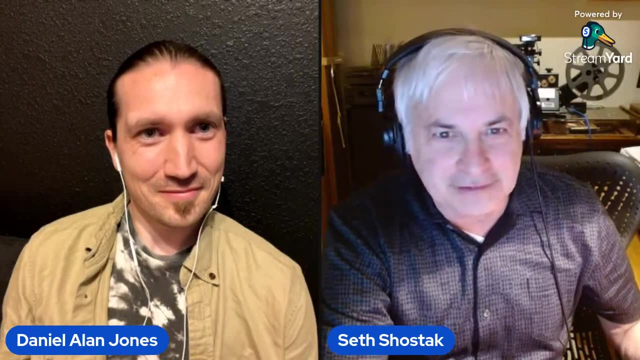 right. You just don't mess with a society that's less advanced than you, because you could trounce them if you wanted to, But that isn't a very nice thing to do. So the idea is that, yeah, they're out there and they're watching us because, well, they're just you know. 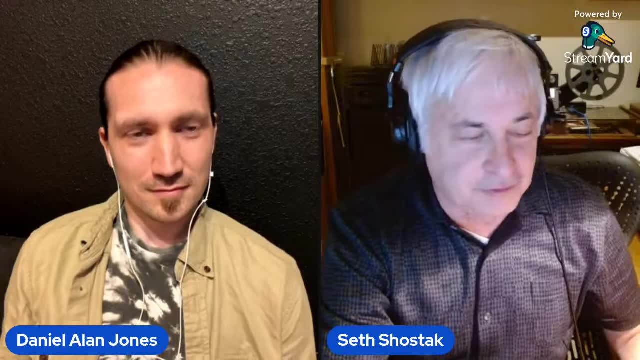 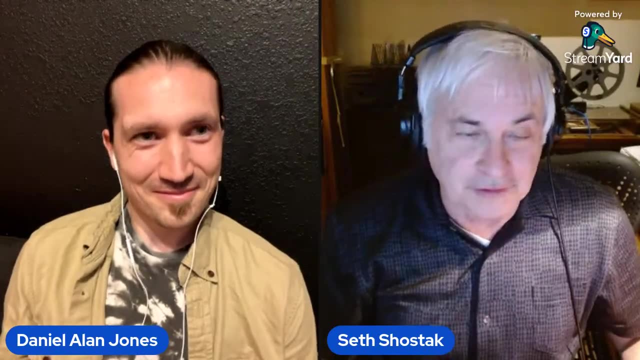 the evolutionary biologists on their planet might want to know what happens to us or something I mean, for whatever reason. So we're exhibits in a zoo, unwitting, and we don't know that we're exhibits in a zoo. So that's the zoo hypothesis. Now, the other thing you mentioned was: 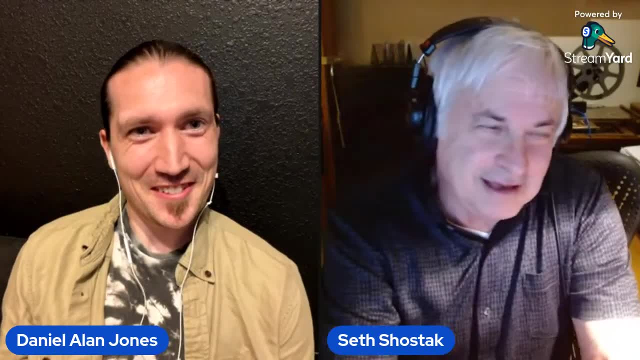 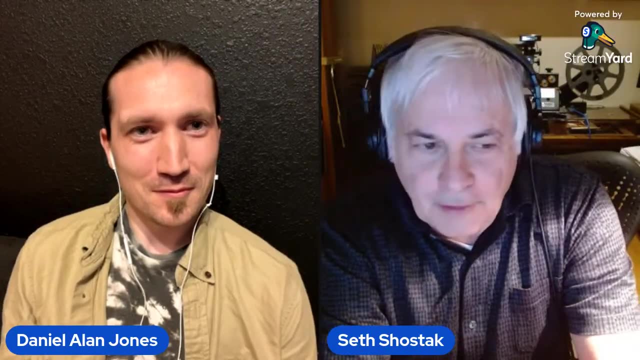 The dark forest. Oh, the dark forest. Yeah Well, the dark forest, that's a more modern term. That's why I had to think about it. The dark forest is to say that, look, you know, no matter what you. 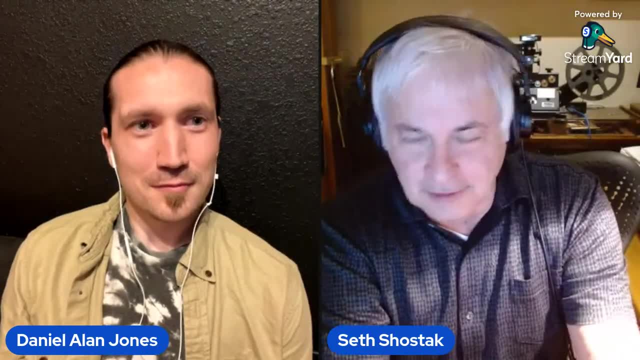 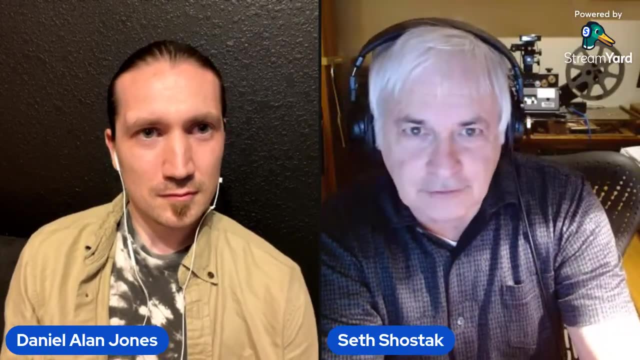 think of this whole subject. maybe it shouldn't be broadcast. I mean, as I mentioned, in the SETI world we don't broadcast anything, but there are people who do And the argument against it is: look, it's like being in a dark forest, right, You don't? 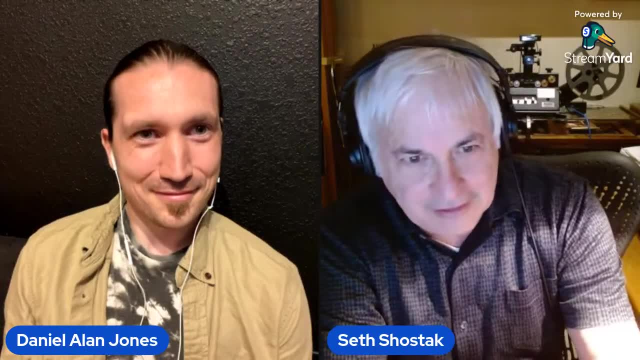 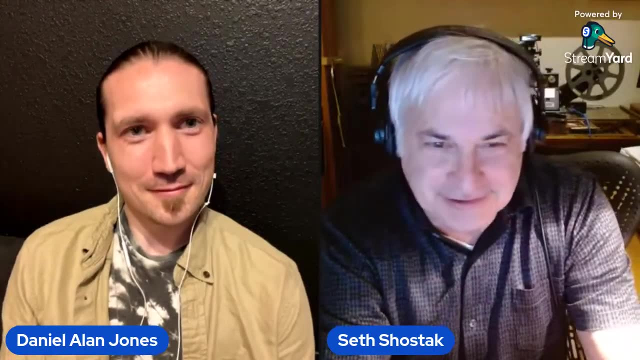 know what's out there. I mean, it could just all be squirrels and you know a few birds or who knows what, But there could be stuff out there that could eat you. So it's better not to make too much noise. right, You're in the dark forest, So you know. that point of view says all right. 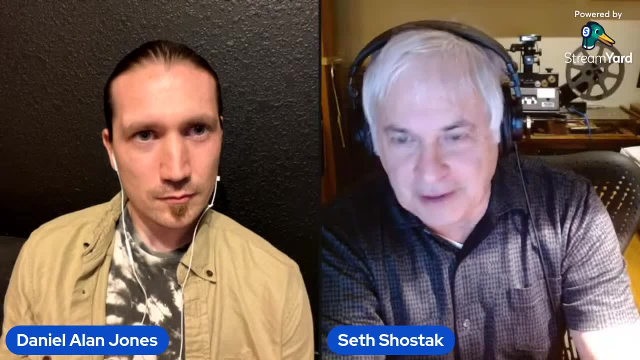 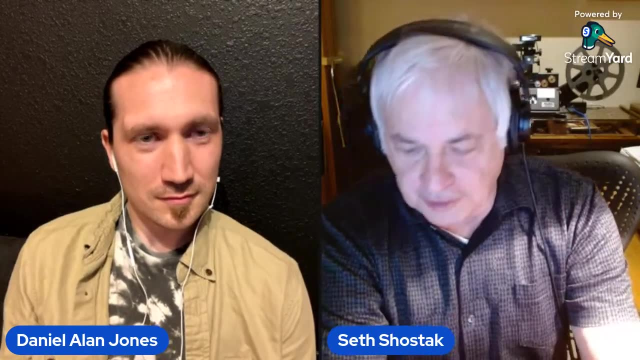 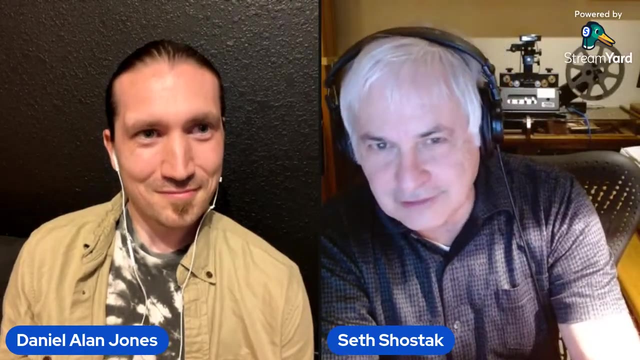 just don't betray Homo sapiens' existence by broadcasting any deliberate signals that hostile aliens may pick up and decide that we might eventually pose a threat to their export markets or whatever, and just you know, send their interstellar battle wagons to Earth and just flatten the planet And that's kind of. 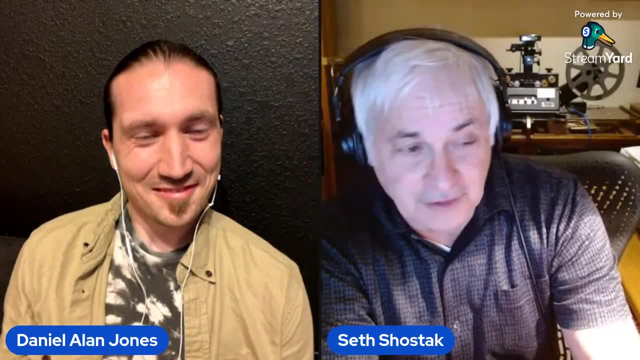 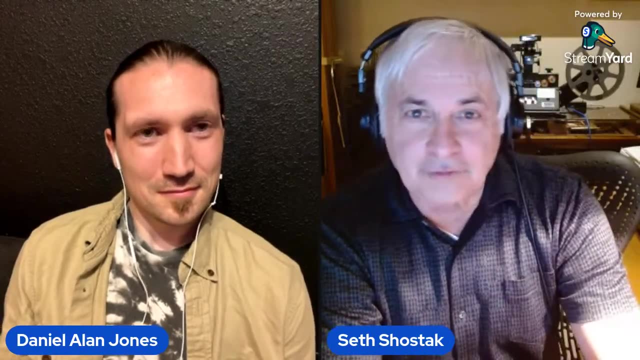 a paranoid point of view And it would be very expensive for them to do that. So I don't know that it's terribly realistic. but there are people who say that look, okay, maybe it's not very likely that if we broadcast into space, ah, we're the earthlings. 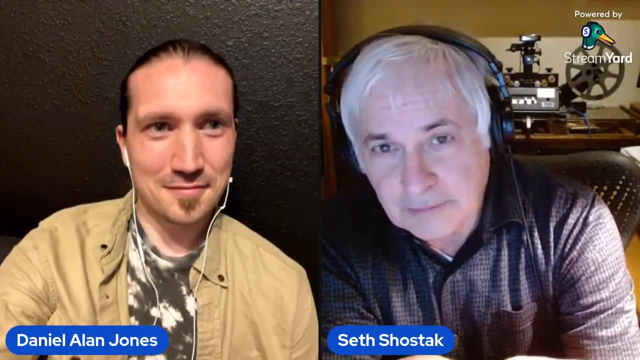 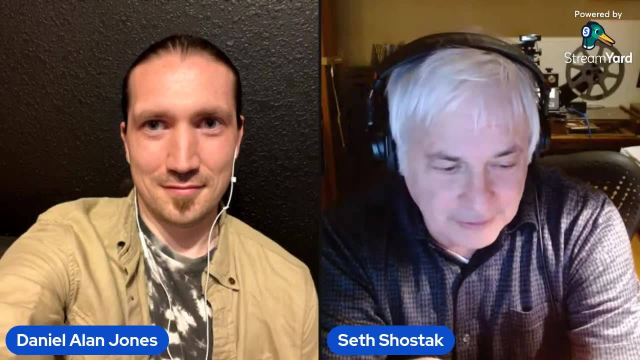 That they're going to, you know, come in and destroy us all, But on the other hand, the consequences could be so severe that you just don't want to chance it right. So that's kind of the dark forest thing, The idea that 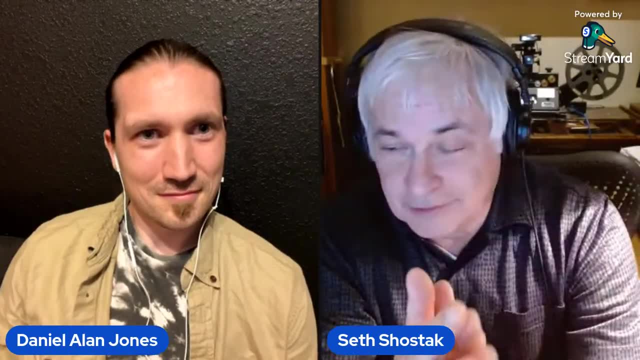 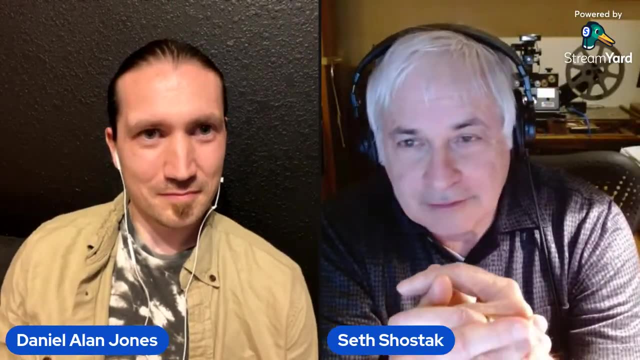 okay, we're here, but don't let them know, we're here Now. just to add one more point to all this, and that is that this whole little story about you know, not making yourself known and all isn't a very convincing 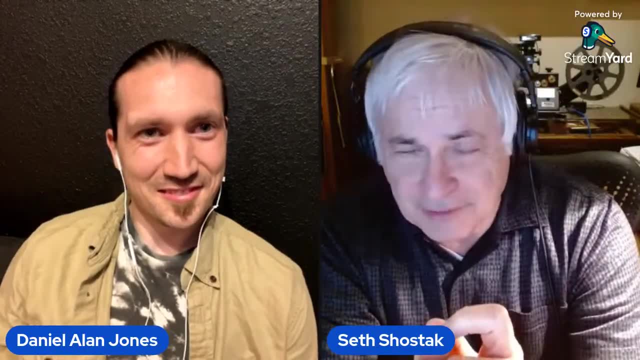 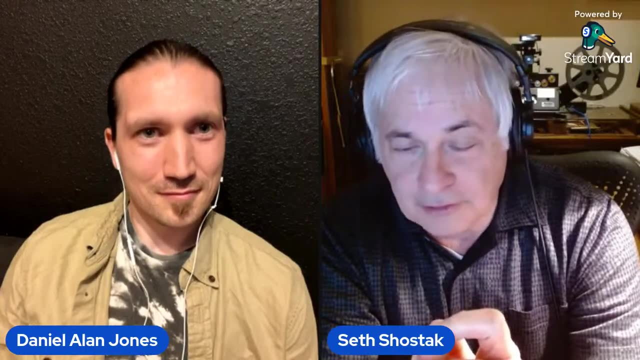 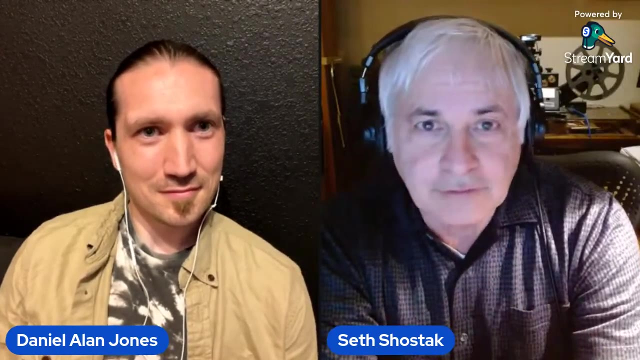 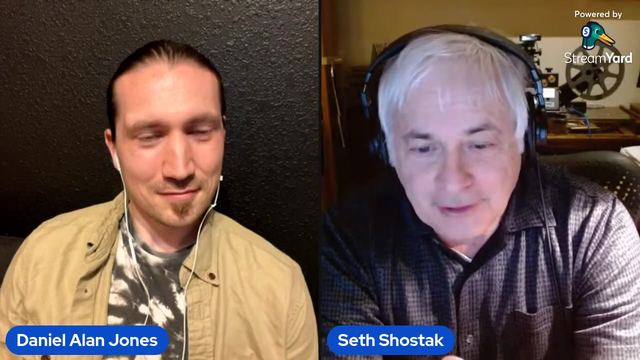 story, because we are making ourselves known, Not the SETI community, But television, radio and, in particular, radar. those are all signals that leak off Earth, you know, without us even wanting them to. They just do right, They go in straight lines, They shoot off the edge of the Earth if you will, And so any aliens with sufficiently large antennas could pick up these signals, whether we want them to or not. So you know, if you're going to worry about it, well you can worry about it, but there's not much you can do about it. 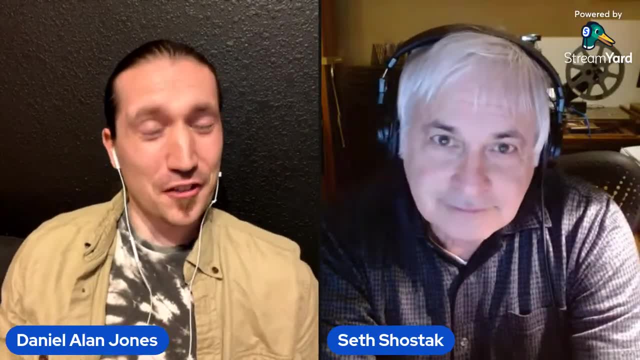 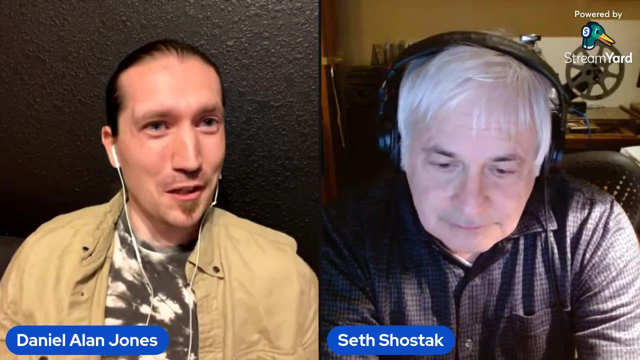 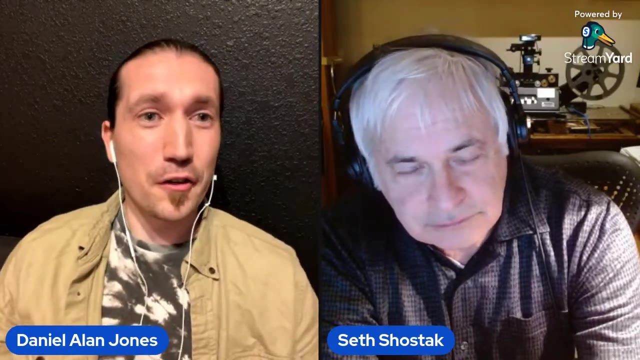 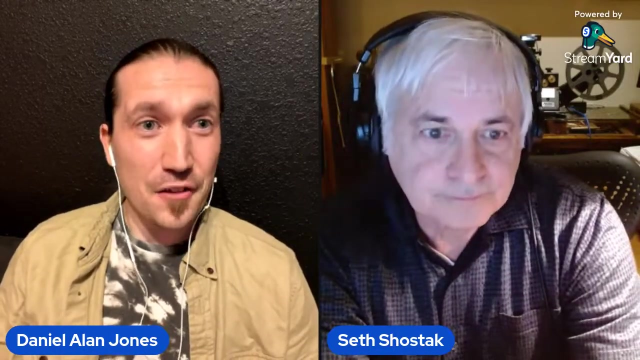 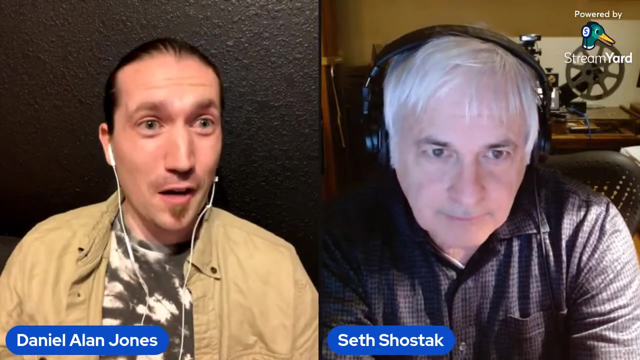 It's really fascinating to think about how much is exposed. It's really fascinating to think about how much is exposed And there are some ideas thrown around about. if there may be beacons- so-called- you know what we can think of as beacons- out there. that would be very obvious. Now, what are your thoughts on the possibility that others looking in, at least toward us, might see Earth in such a way? Would Earth be observed as a type of beacon, in the sense that it's spewing emissions and things that show signs of obvious manufacturing? Would that be something that? 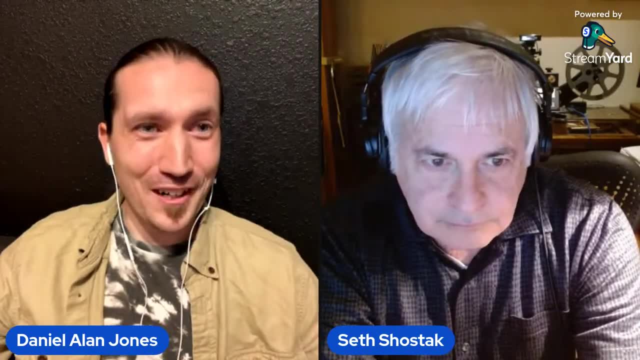 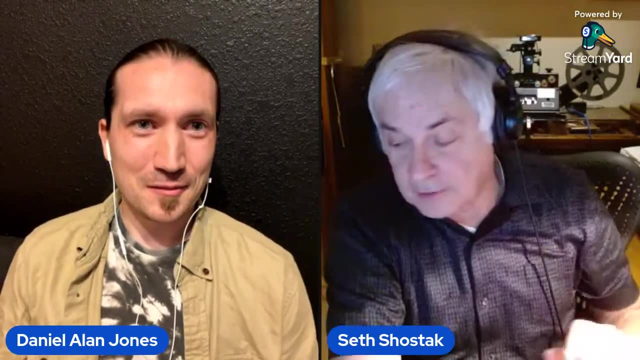 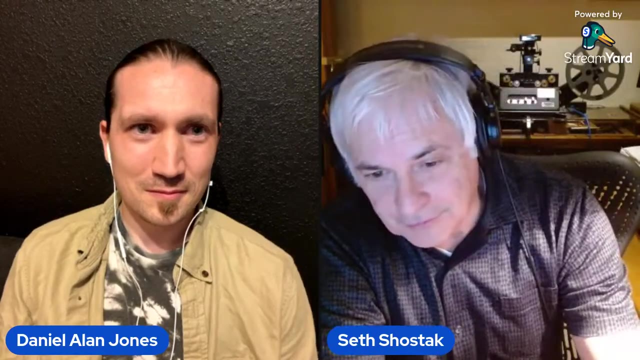 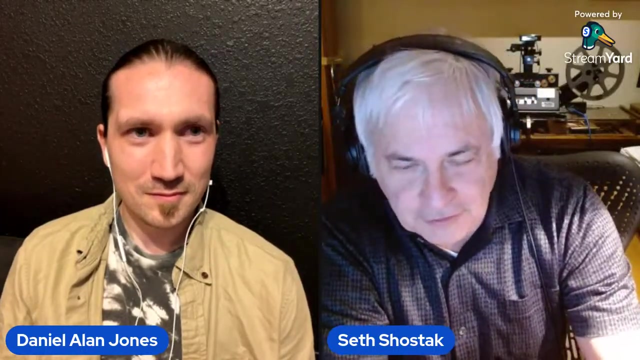 you know, we we look for out there, but that other people, whoever else is out there, would see that might be obvious here on Earth. Well, depending on their level of technological development, yeah, they could very well pick up something from the Earth. Now a couple of caveats To begin with. you know, if the aliens are 50 light years away, that's pretty close actually. But let's say they're 50 light years away, The signal's taken 50 years to get to them. Okay, that's neither here nor there, But the facts are that at 50 light years the signals from Earth, they're not going to be able to pick up anything from the Earth. 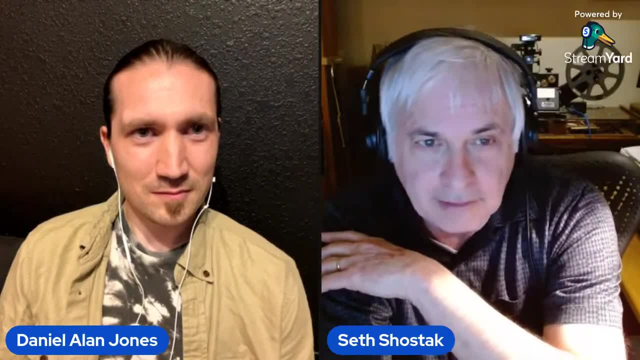 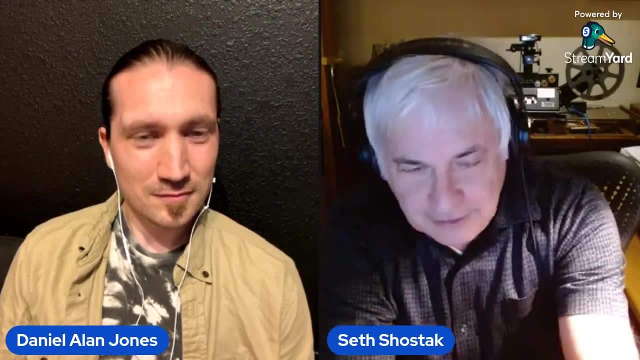 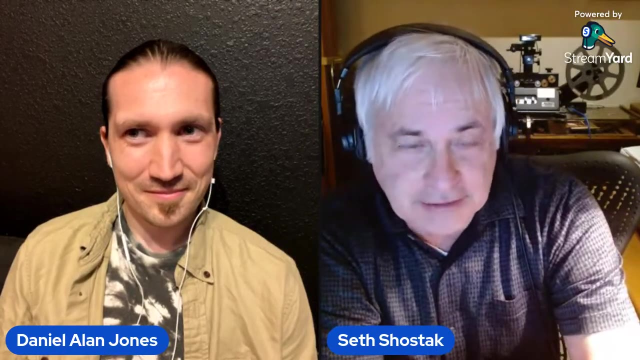 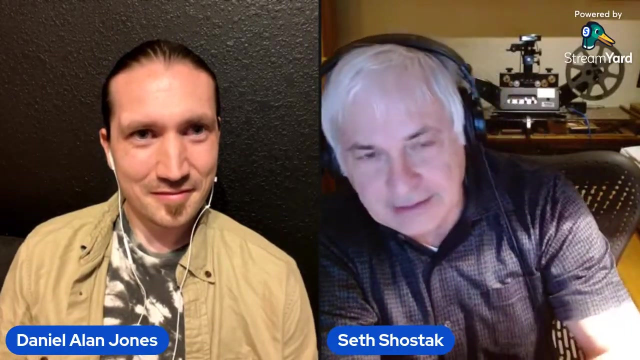 Even the most powerful signals that we make radar right, those are the most powerful signals to me. They get weaker with distance, of course, as your flashlight right. You go out in the evening and aim the flashlight at your neighbor's house and it'll light up the house a little bit. But if you aim the flashlight at the moon right, you're not going to see the reflected light, even though it's getting to the moon. You know it's so weak by the time it gets there and back that you don't even see it. So you know this idea. 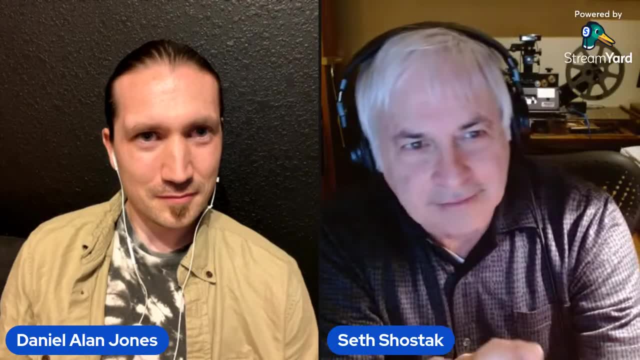 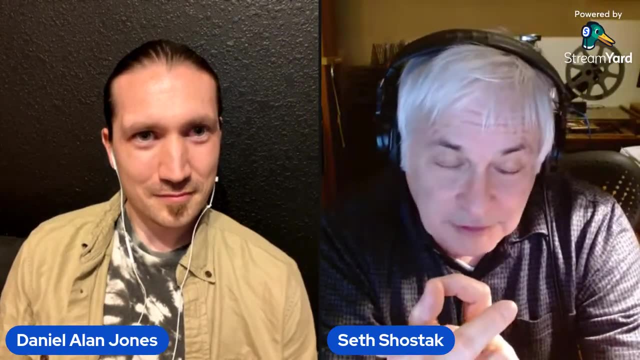 that it's, you know, dangerous and that you know we're betraying ourselves. well, all of that is true, But you know it doesn't have much to do with SETI, because SETI isn't doing that. 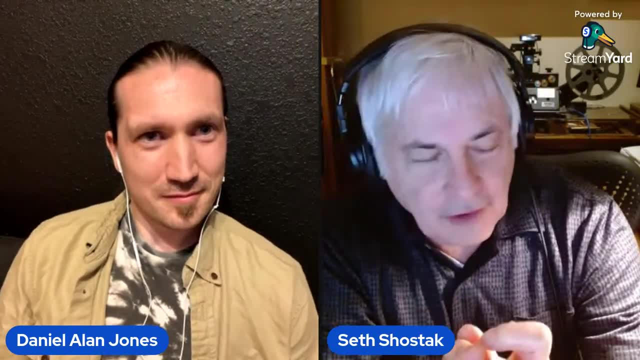 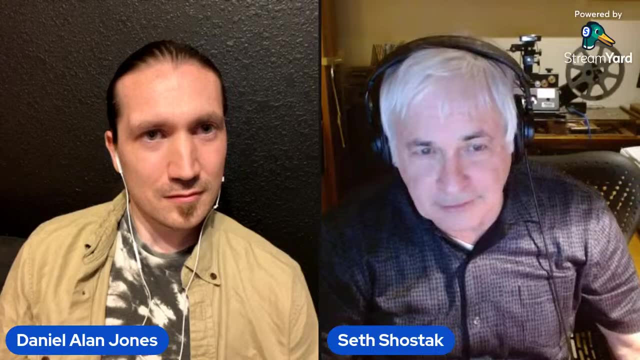 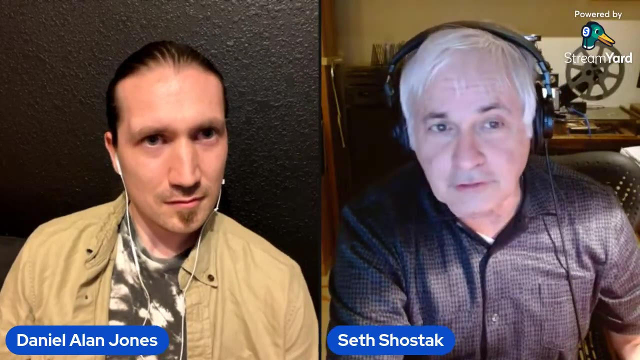 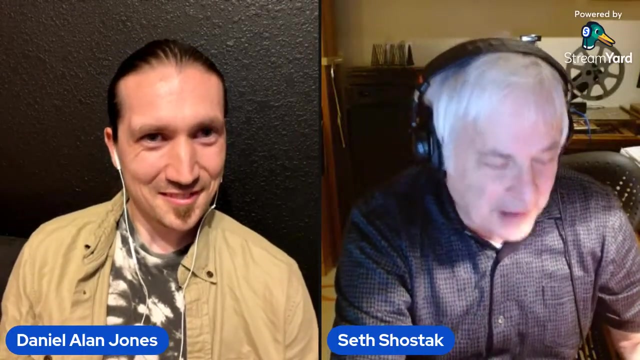 So I think these things are interesting stories, but there's, you know, they don't affect the experiment very much because the experiment is a passive one. We're just trying to eavesdrop, We're trying to pick up signals And you know, there's, as I said before, there's no danger in listening for signals. right, You can sit at home all day long and tune the dial of your radio and it just doesn't have much potential for a bad outcome. 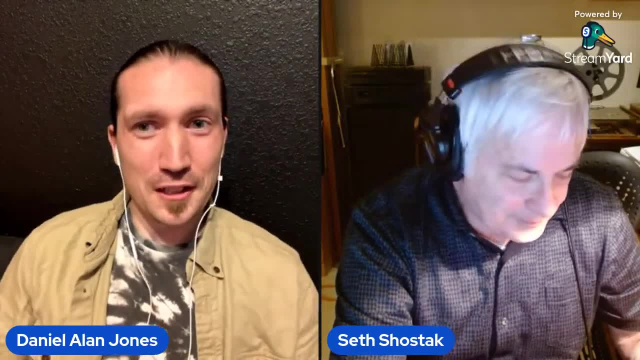 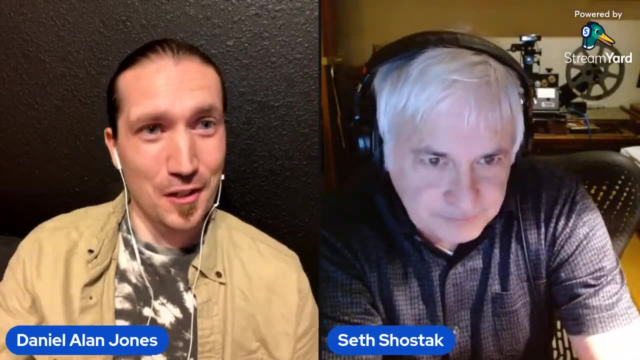 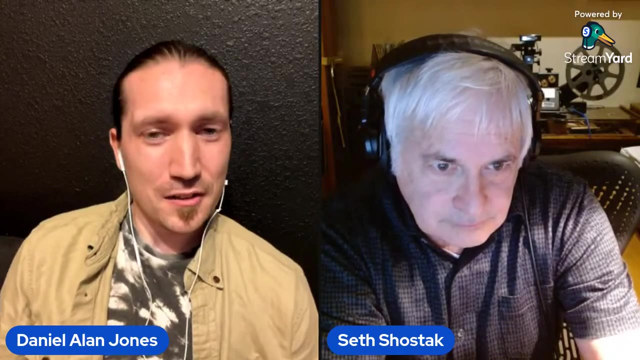 well, it's something that i think you know. when people wonder about these ideas and and the reality behind it, it helps to have light shed upon them in such a way that it's good to know that you know we have people such as yourself who are working on- uh, doing what we can to try. 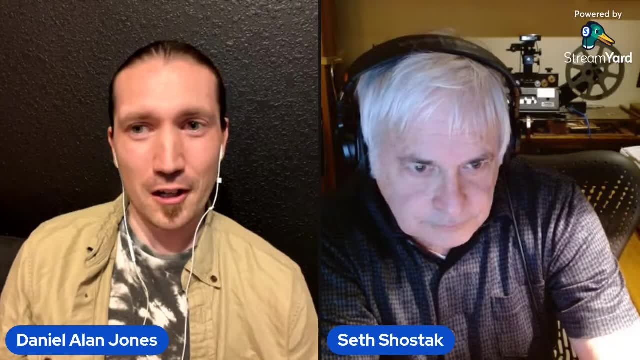 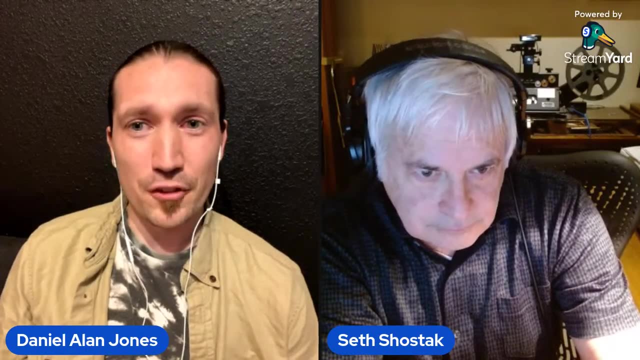 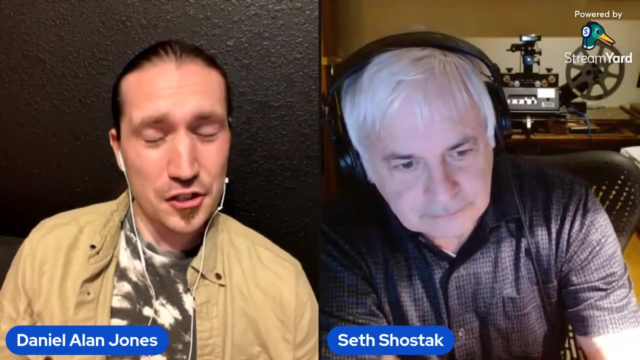 to understand signals and see what frequencies are out there, um knowing that we're emitting them. um it's possible that there could be something else that we might notice as well. um, some people have considered there are ways to uh, classify or categorize types of civilizations that could. 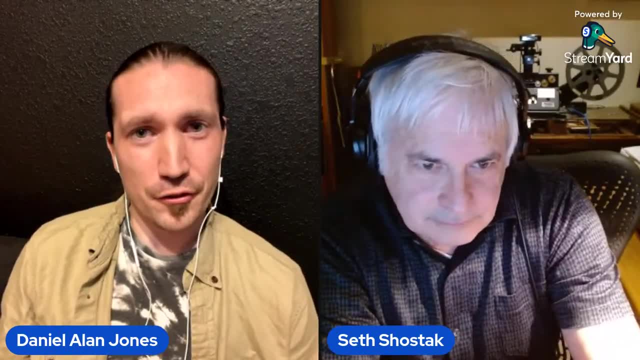 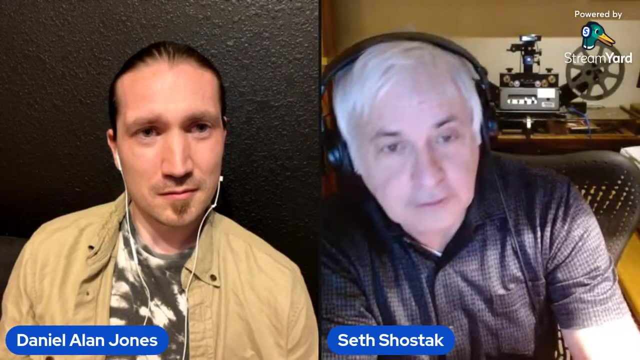 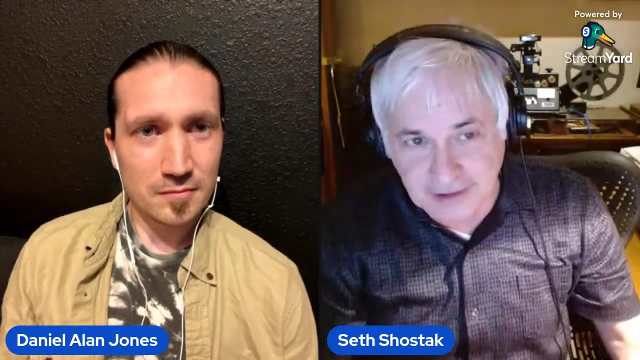 potentially exist in the universe. what are your thoughts on the kardashev scale and the type one through three civilizations? yeah well, kardashev was a soviet physicist. he's- he's gone now. but nikolai kardashev, and what he said was: well, he just he had a taxonomy scheme for for societies. 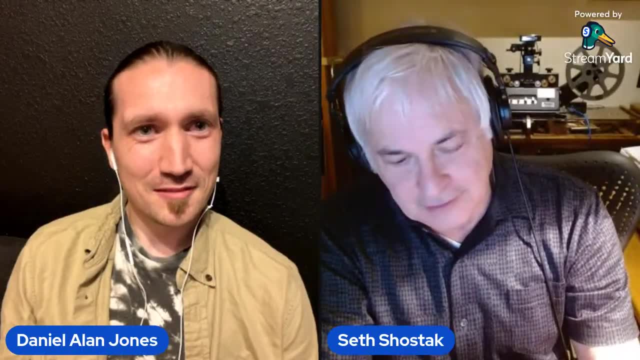 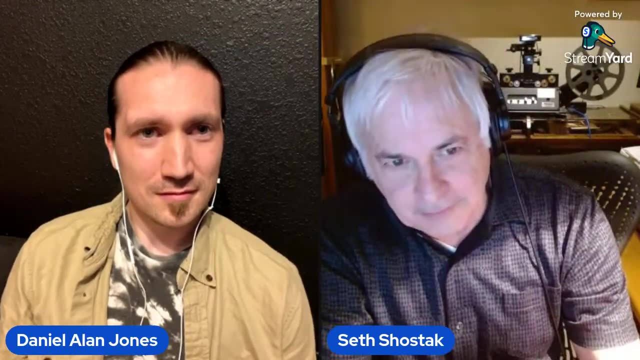 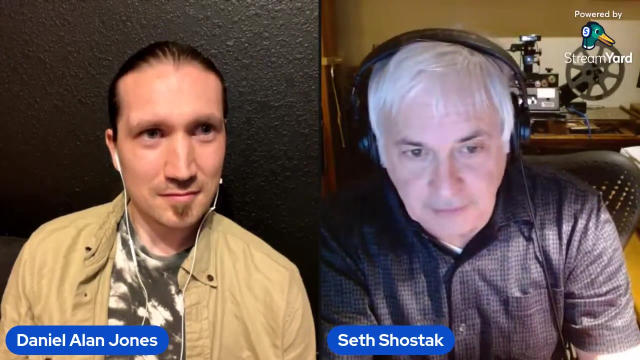 he said: look, you've got three categories of societies. type one societies use the energy available on their home planet right. type two will use the energy not only on their home planet, but the energy of their star right, their sun. and type three would use the energy available from all the stars in the galaxy. 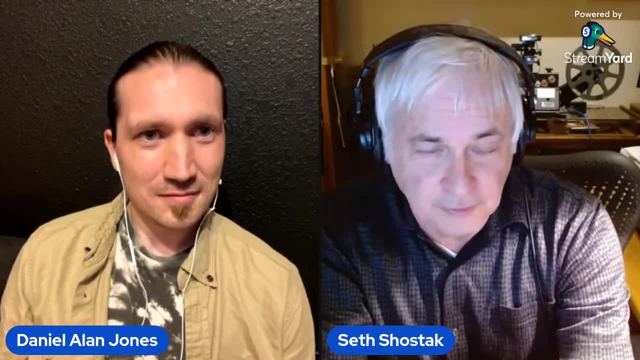 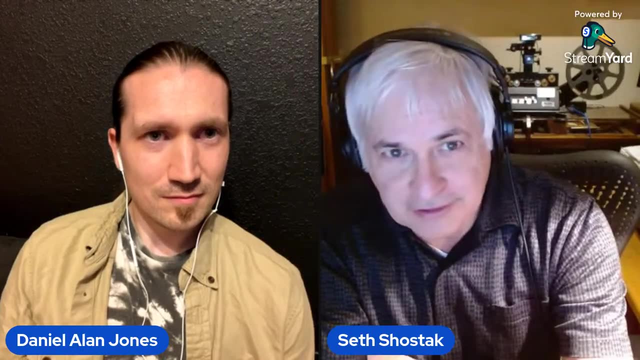 right. so that's a couple of hundred billion times more than available from their own sun. so you know, if you categorize societies on the basis of their energy usage, it's just called events and states stay as it is. but um in in in these days, of course it's, it's. 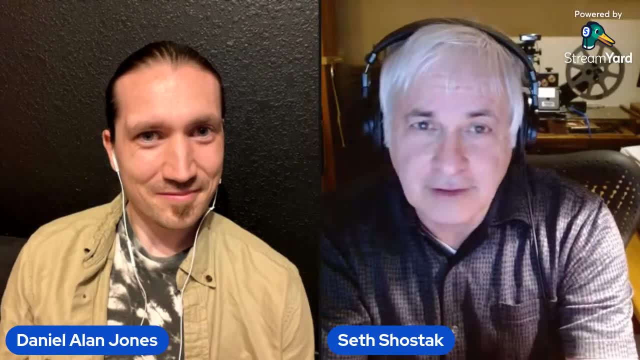 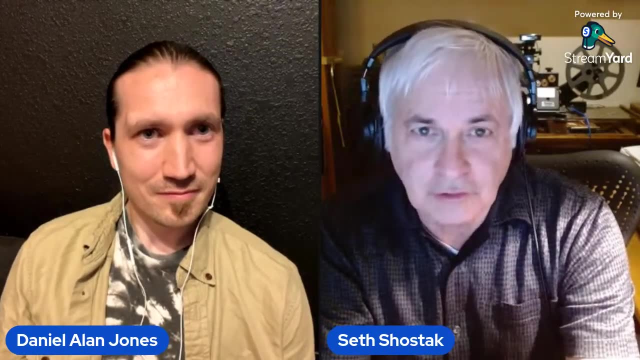 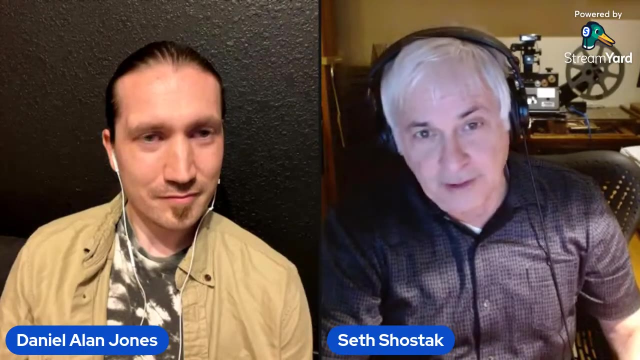 preferable to use less energy for various reasons that are obvious to all the listeners. but you know, uh, it's also the case that if you want to measure a country's economy or a planet's economy, how much energy they use for inhabitant is a good measure, the more energy they use for inhabitants. 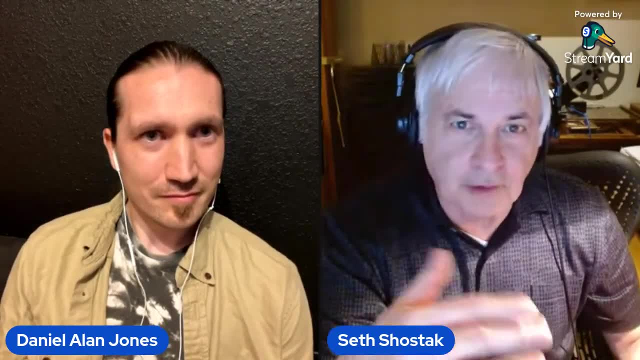 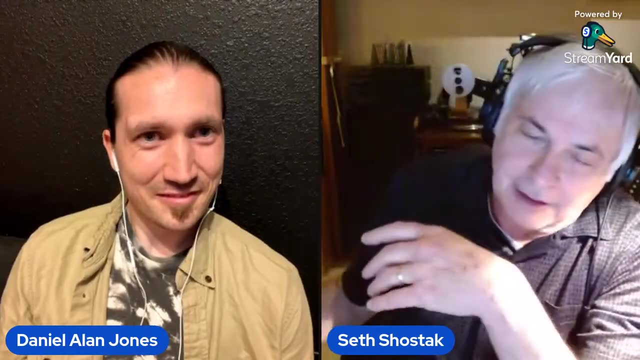 you know, the more advanced a society is, we we use quite a bit. i mean about 10 kilowatts. That's the amount of energy usage, right? So I mean that's adding up, you know, the car and all the lights in the home and the TV set in the corner and all this stuff. 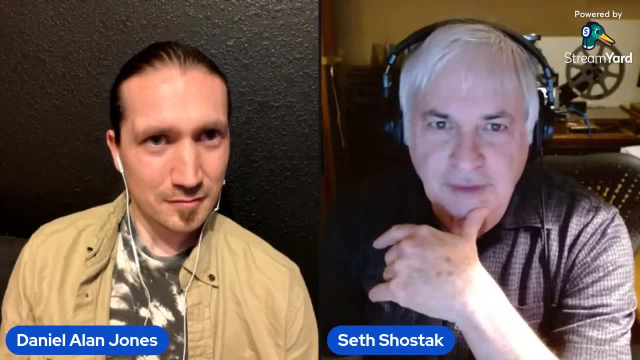 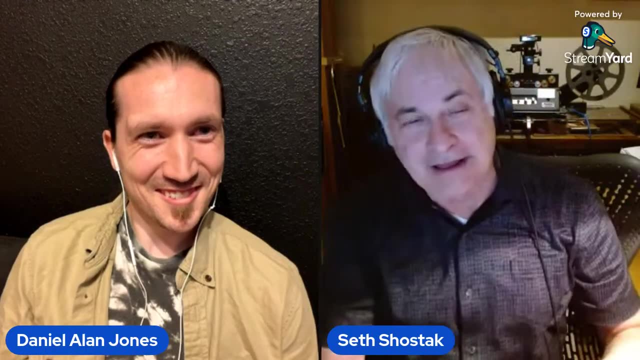 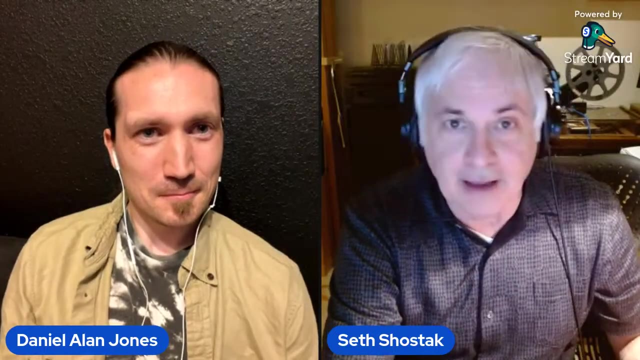 Everything that you use that consumes energy more or less adds up to 10,000 watts. How much did Julius Caesar use? Well, a lot less than that. He didn't have electric service there in Rome, right. So it is a measure of, if you will, economic success to use more energy, But 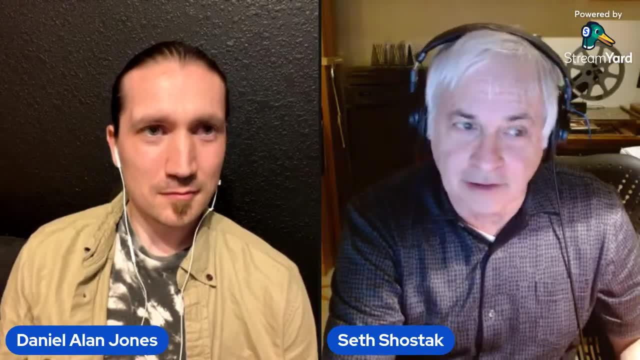 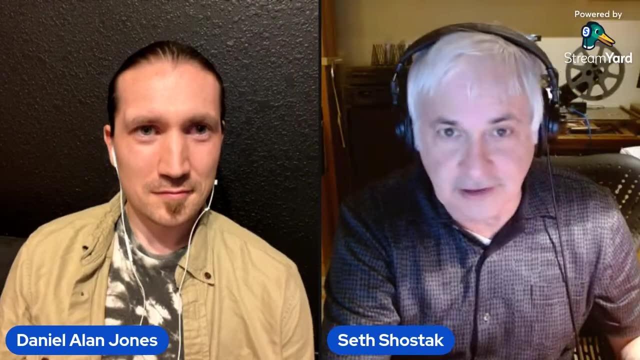 Kardashev was just extending that a little bit by saying: look, you know, if you have technology that allows you to capture all the energy of your home star, in our case the sun, you know you're pretty advanced. And that would be true. I mean, the earth intercepts only a couple of 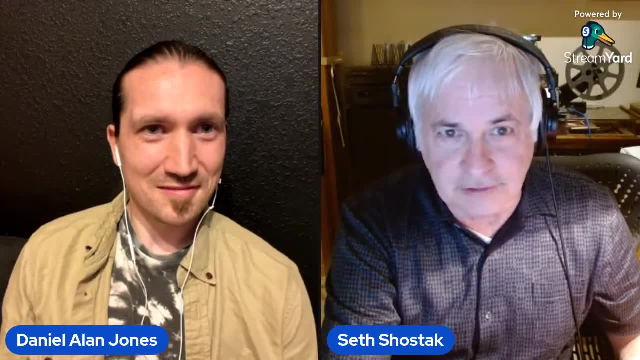 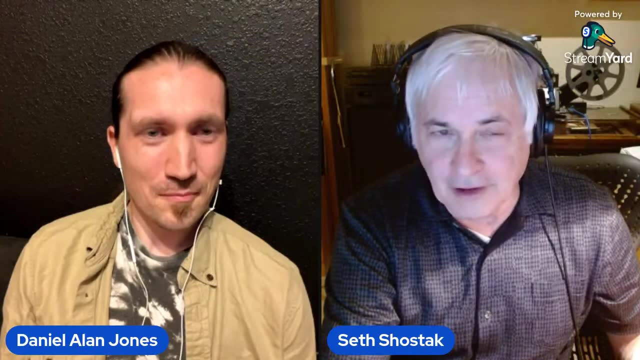 percent of all the energy emitted by the sun, And most of that just gets reflected into space by the clouds or the ocean or even the land. We don't use very much of it, So we're really not a Kardashev type three society. 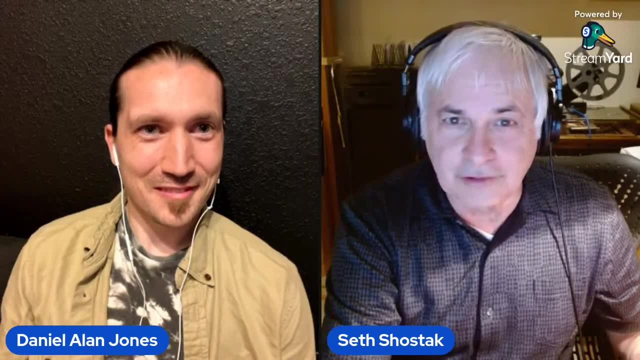 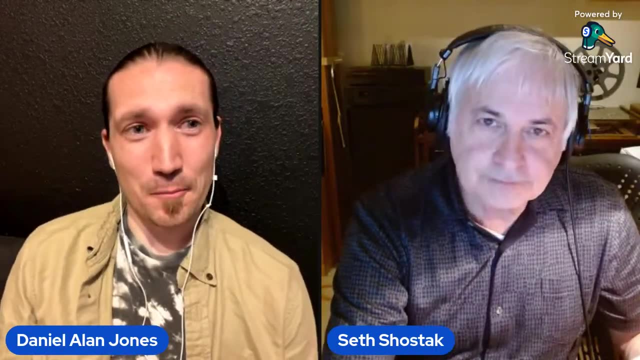 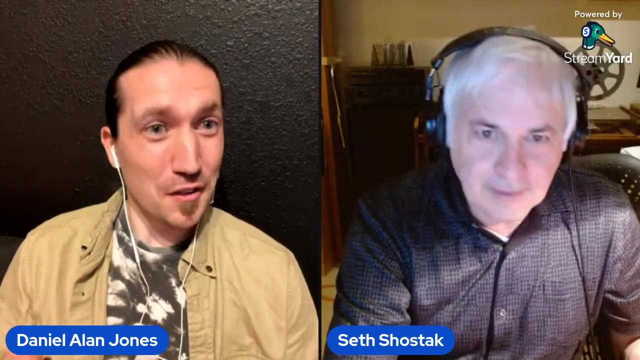 or even, for that matter, a Kardashev type two society. We're just still doing baby steps, Yeah, And it seems like we're maybe not even you know, type one. It seems like, maybe until we unify as a collective civilization and we, you know, work in equilibrium with the planet. 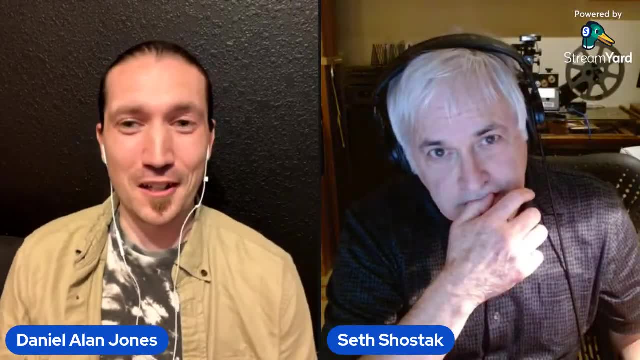 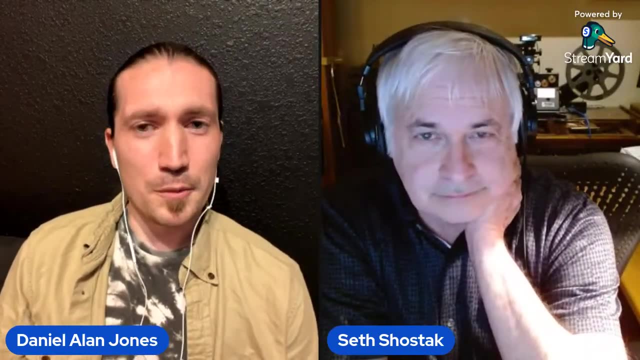 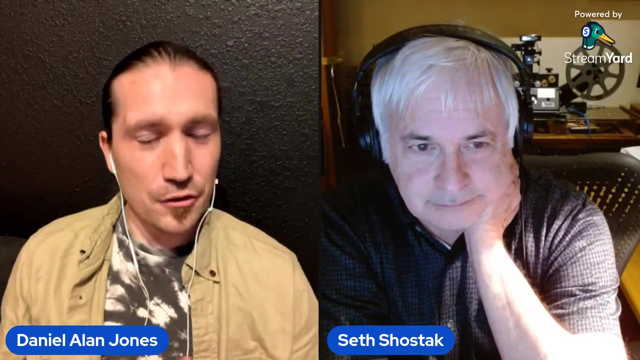 that we might be able to get to that point. Hopefully so. I'm at least thinking now that That's something that's possibly within our future. Some have speculated that a type two would be capable of producing and manufacturing structures that could be utilized, as you just 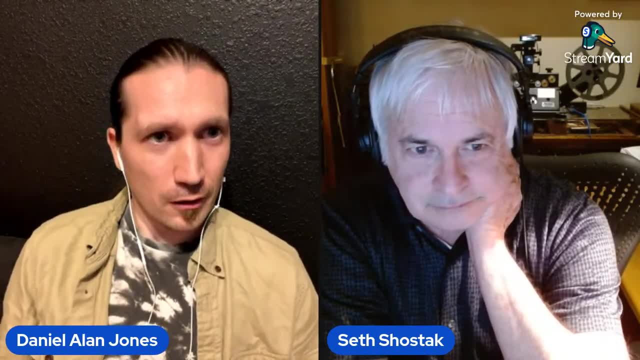 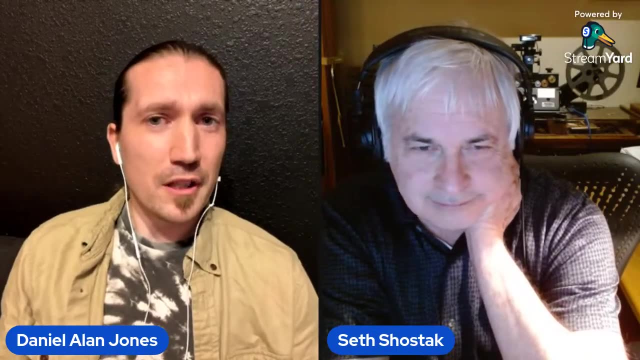 mentioned, to harness the energy output of a star, or maybe several stars. There's the notion of the Dyson sphere. What are your thoughts on something that's a construct like the Dyson sphere? Is this a practical notion, or are we maybe looking at it from a different perspective? 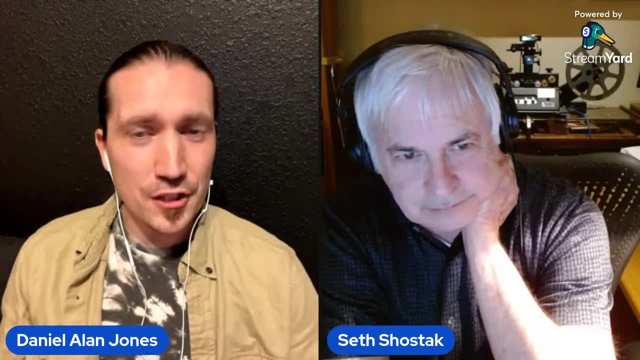 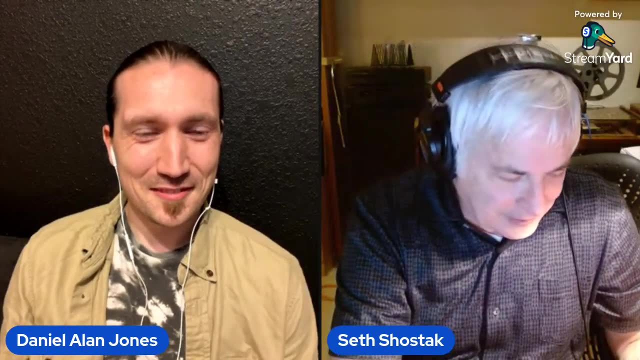 Are we looking at this in a similar vein of our technology? What are your thoughts on the Dyson sphere? Well, for those who are not into Dyson spheres, this was just an idea by the physicist Freeman Dyson, British, but he also worked in the United States, worked at Princeton. 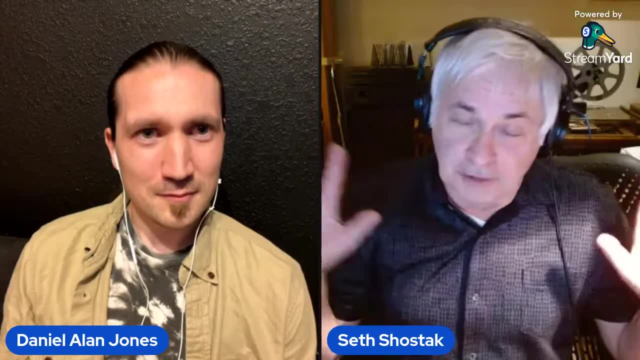 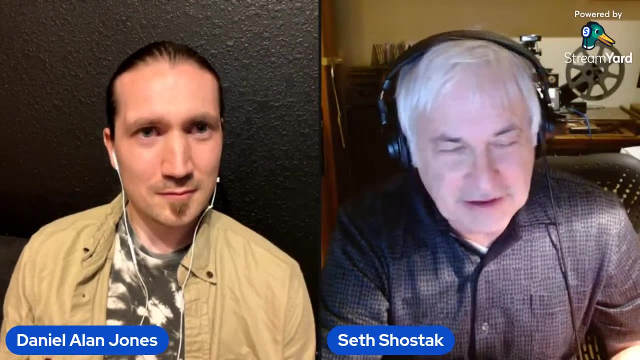 for quite a while actually. And Freeman Dyson, you know he was looking always at big picture things And he said: look, if you're an advanced society, you don't let 99% of all the energy output by the sun go to waste. 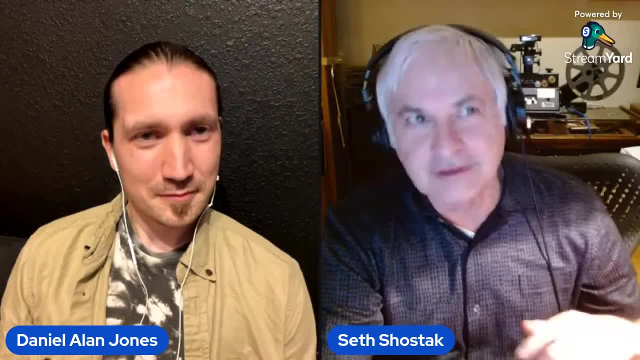 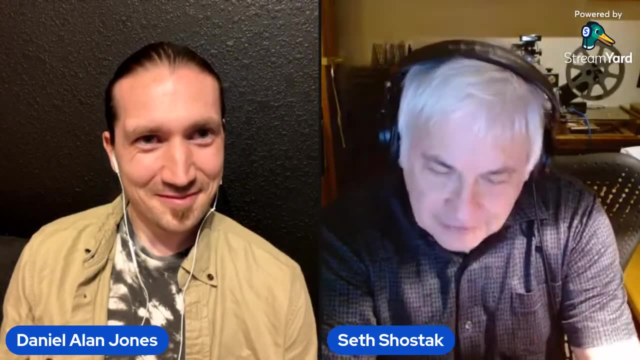 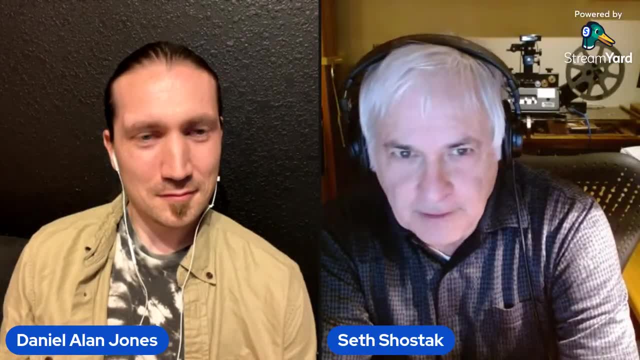 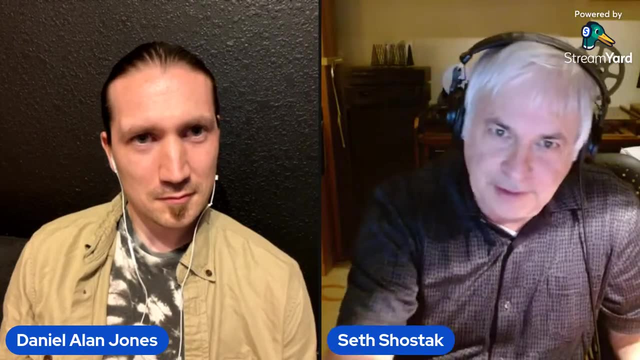 big, you know, if you will, a sphere. Well, it's not a sphere, It's just the shell of a sphere around the solar system, so that the earth is orbiting inside that shell. All right, They cover the inside of the shell with solar cells, So now you're collecting all the energy radiated. 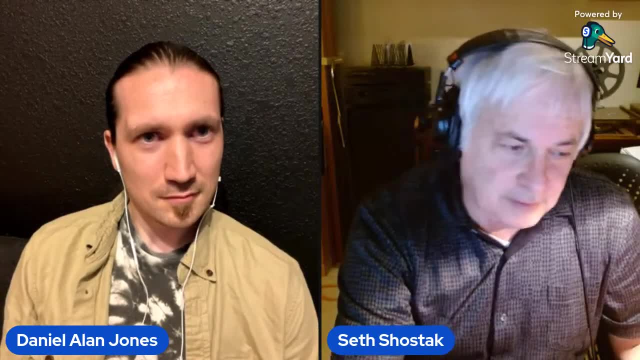 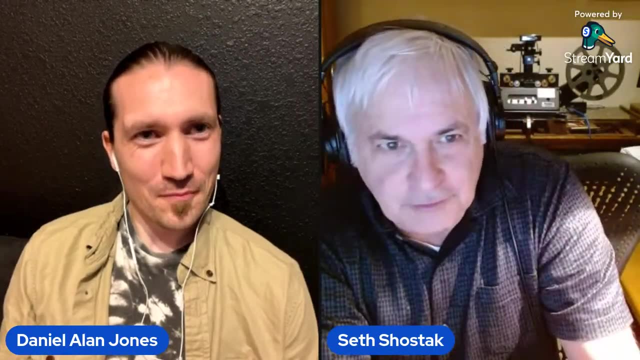 by the sun, You convert it into electricity and then you beam it down to earth so we can use it for, you know, video gaming or whatever we're going to use it for Now. that would give us billions of times more available energy, And that would give us billions of times more available. 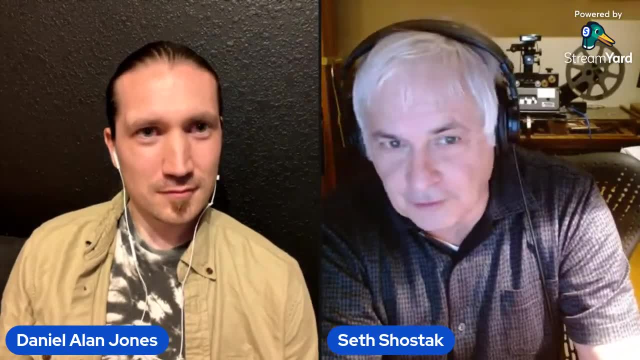 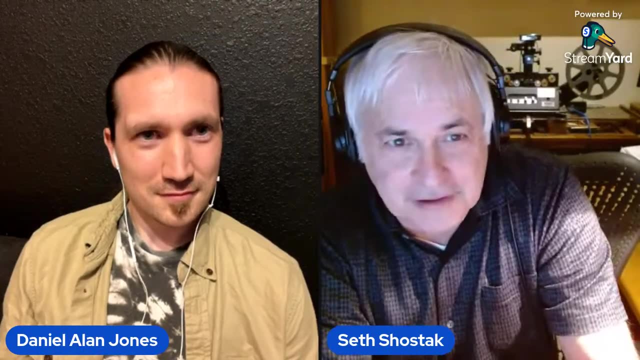 energy than we have now, with all our fossil fuels and our nuclear fuels and, you know, the windmills and the solar panels and all that stuff, We'd have, you know, billions of times more energy and maybe we could do more interesting things. Maybe we could. I'm probably, I'm fairly certain. 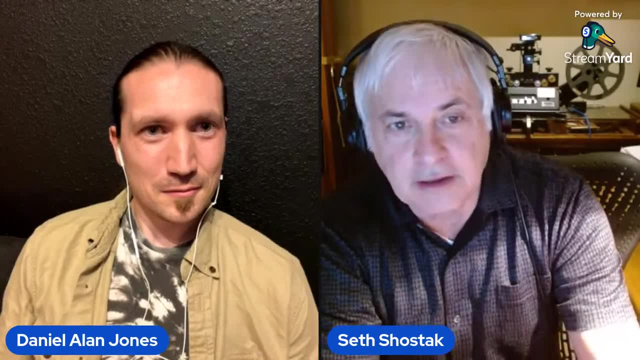 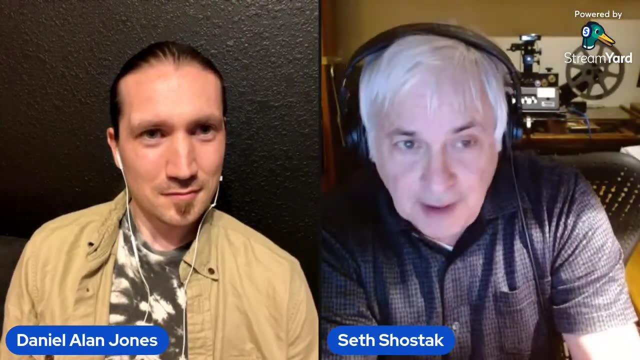 we could do more interesting things, But the idea was only to say: look, if you're a society that's millions of years more advanced, or even thousands of years more advanced than ours, you might be able to do this. So we should look. 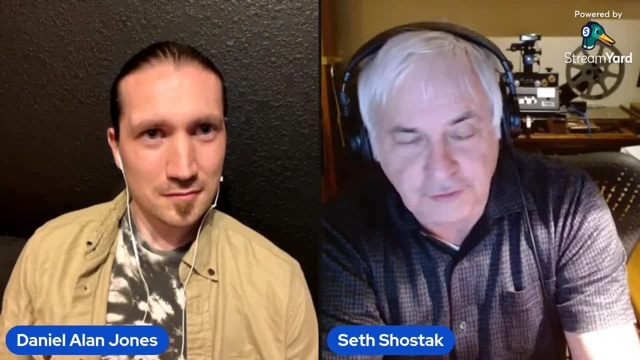 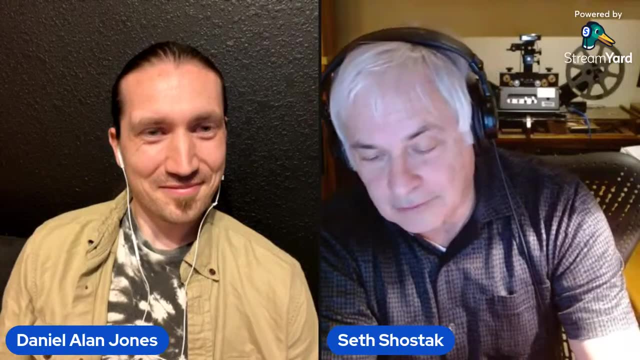 Look for these Dyson spheres or partial spheres out in space, because really advanced societies may have done this. It's one way for them to get a lot more energy than you know: digging up the landscape, looking for things they can burn. It's very interesting And, speaking of video, 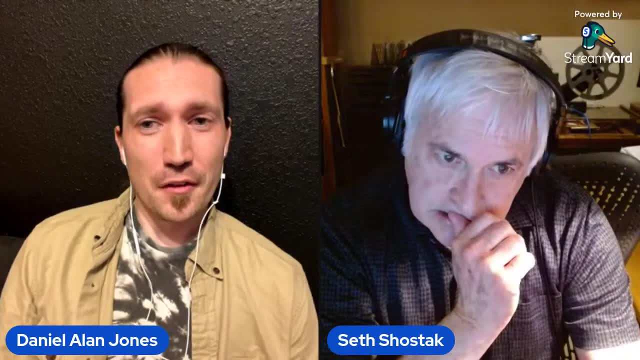 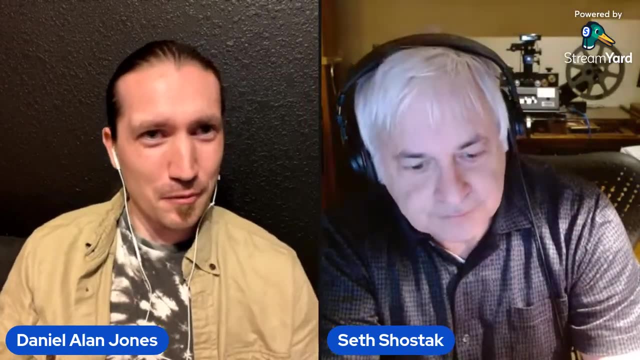 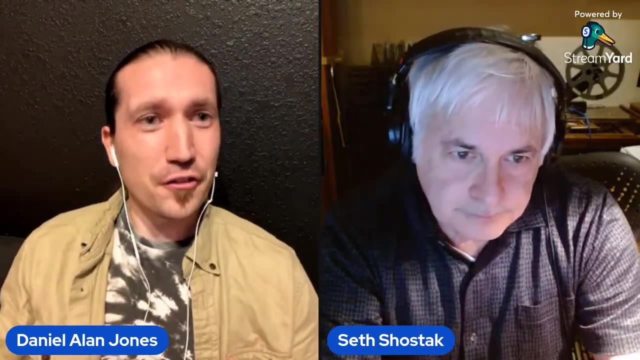 games. another and very similar thought is that of the Jupiter brain, or Boltzmann brain, or even, considered, the Matryoshka brain. Are you familiar with this idea and how? it's supposed to be? something very similar to the Dyson sphere, but its function is that it simulates realities. 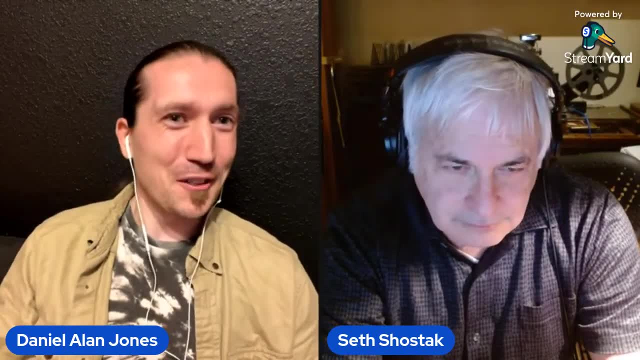 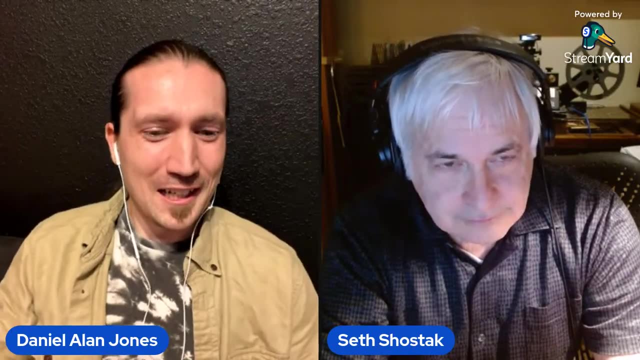 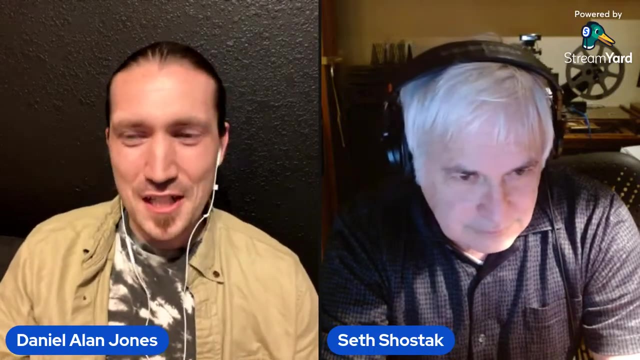 And in doing so might propose another completely tangential issue of if we exist within one of those many simulated realities. essentially sounds like a very challenging issue to undertake, and more of a philosophical one. But what are your thoughts on the idea of a Matryoshka brain? 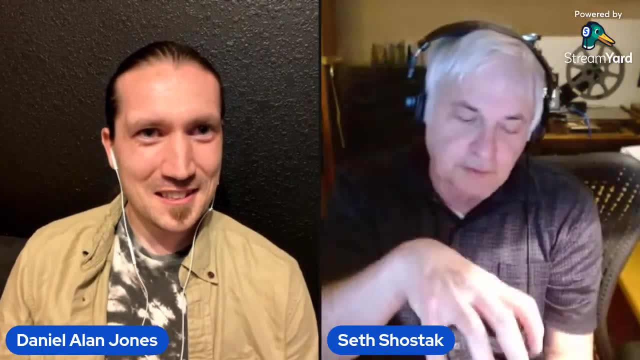 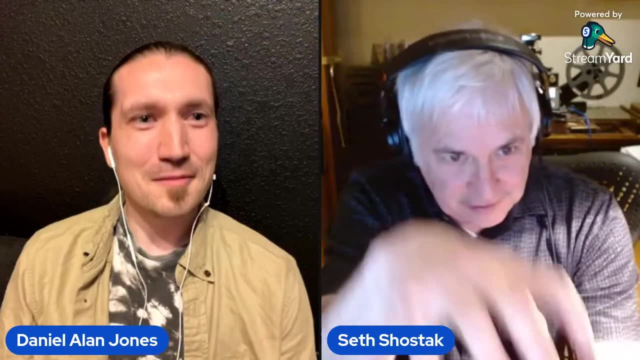 Now these Matryoshka brains. I mean, you know the Matryoshka dolls, Russian dolls. anybody who's been to Russia knows about these dolls. You can buy them all the shops and they nest one into another. You know, here's a small one in the middle and then a bigger one. 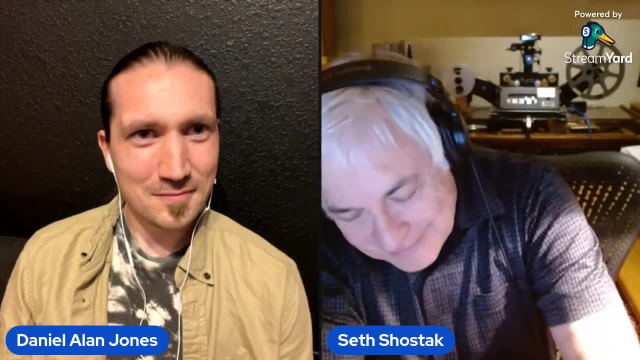 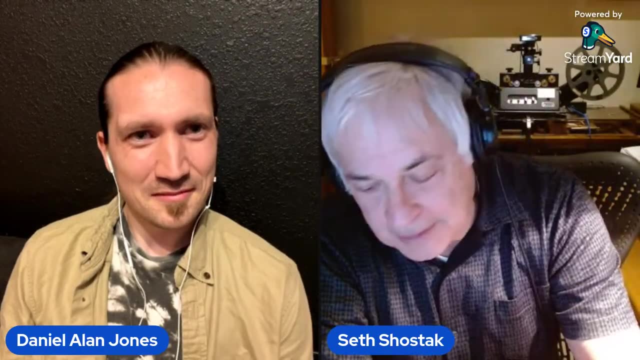 and a bigger one. So you know, I mean, what are you going to say about it? I mean, they may exist, that kind of thing. It may be that I don't know. I mean, I guess, what I'm trying to, struggling to. 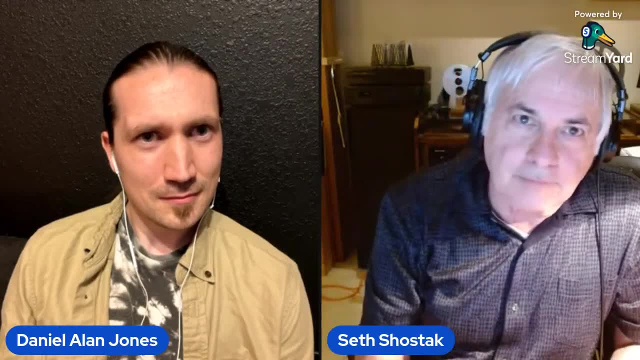 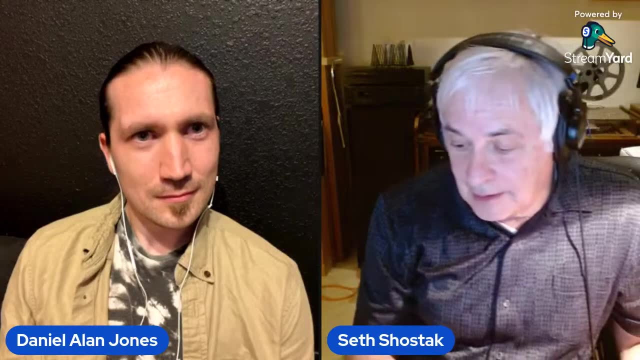 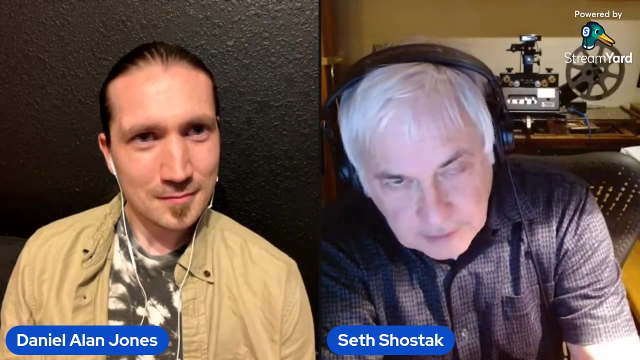 get to is how this is relevant. Does this say anything, Anything about what the aliens might be like or what they might be interested in doing? And I'm not sure that it does on neither case, But it is, you know. I mean it pertains to the 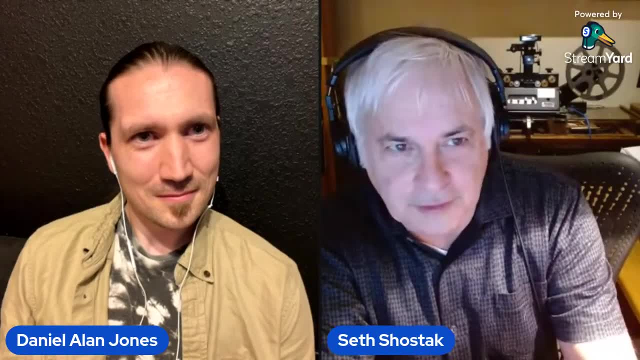 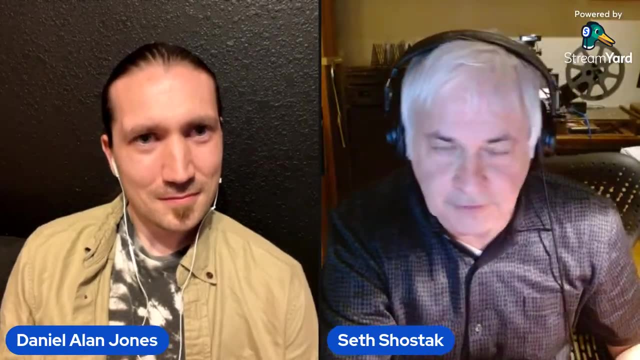 aliens in this sense, because you're talking about brains within brains or brains in general. Will the aliens have brains that are bigger than ours? Well, some of them will, of course. Will they be smarter than we are? Well, probably a lot. 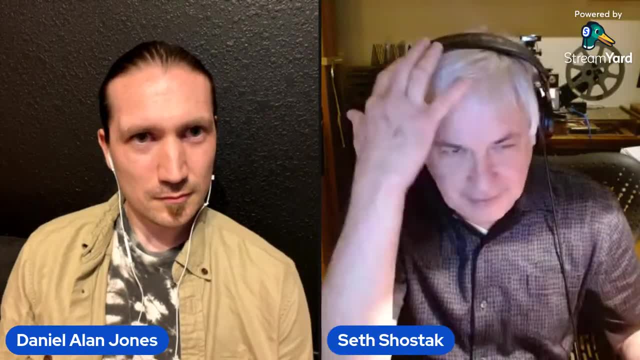 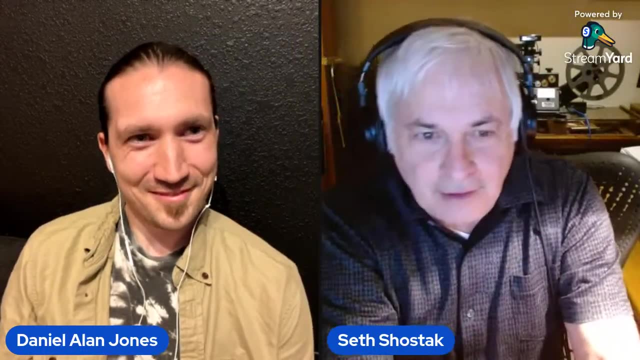 smarter than we are right. More technically advanced- I mean our brains- are. you know they're one and a half pounds or three pounds or two pounds. a couple of pounds depends on whether you're a fathead or not, But you know, it's just a couple of pounds And we do everything that we do. 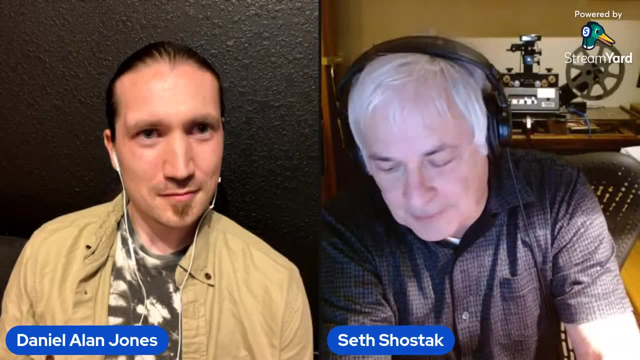 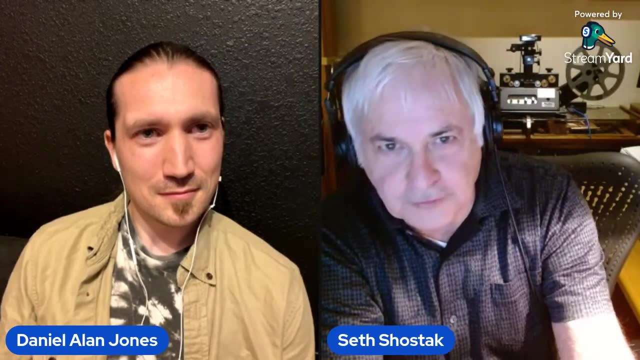 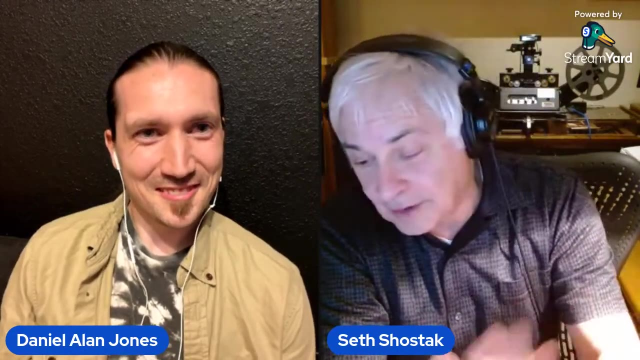 with, you know, essentially a machine that's only a couple of pounds right. So you know there's no reason that you should stop there. It's just that nobody can give birth to babies that are going to have 500 pound brains. So that's where we're limited by that. But you know you can beat. 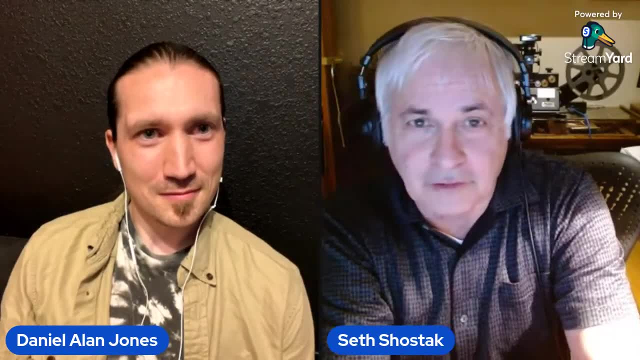 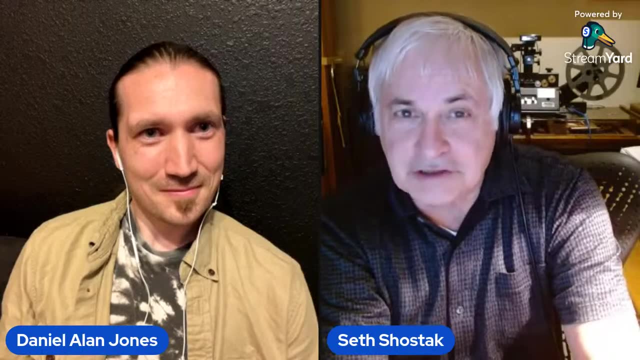 all this by inventing artificial intelligence. We seem to be doing that as well- And then you can build the brain as big as you want, consuming essentially as much power as you want, And in fact you could imagine combining these two ideas that we've been talking about. that you, you know. 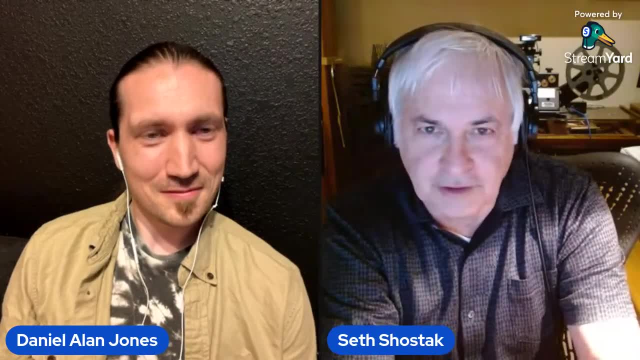 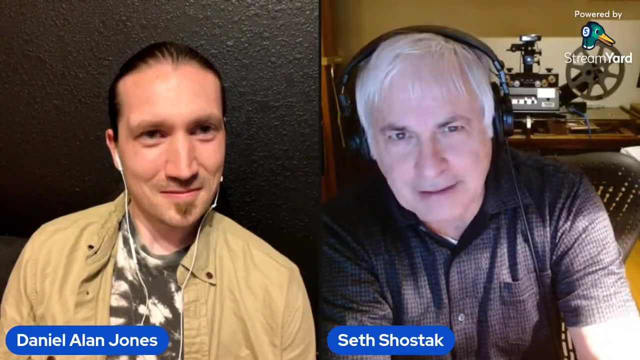 you build a Dyson sphere or a partial Dyson sphere and you use it to power. you know an artificial brain. And now you can. you know, not only can you play a lot of games of chess, you can also, you know, probably work out all of. 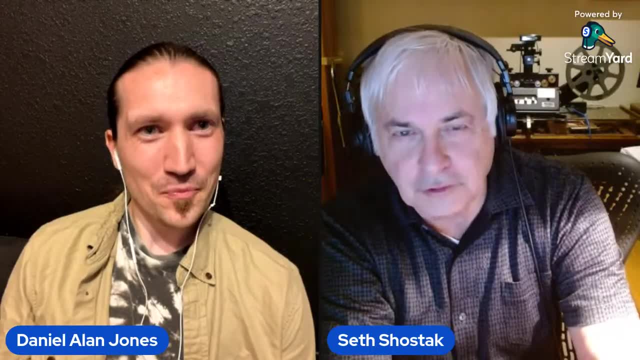 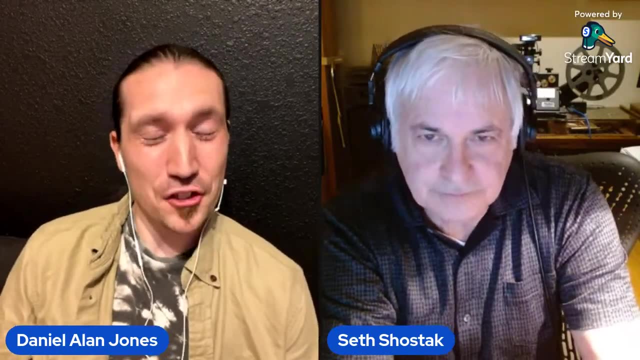 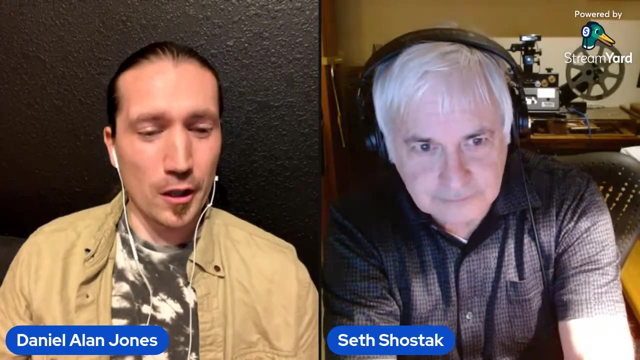 science too. I mean, you know and probably write a few good short stories as well. Awesome, So you know. on the thought of video games and simulations, SETI just published this article about the work that's currently going on, that's simulating. 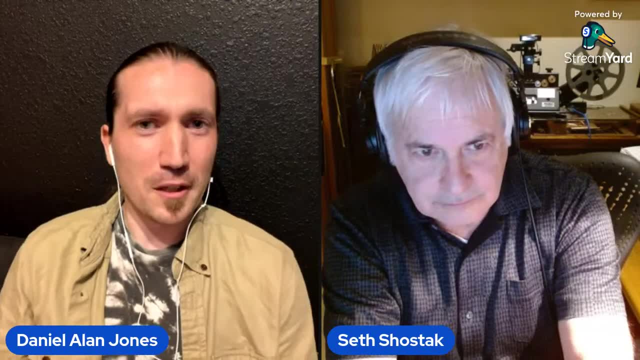 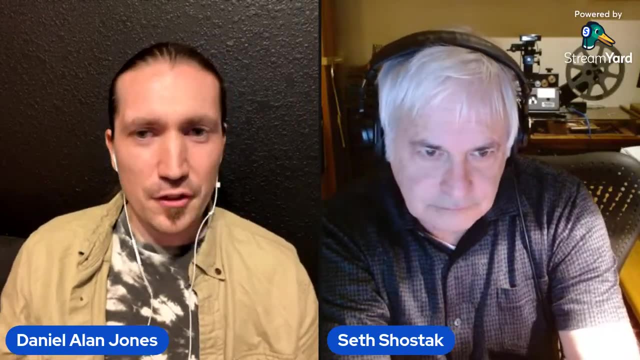 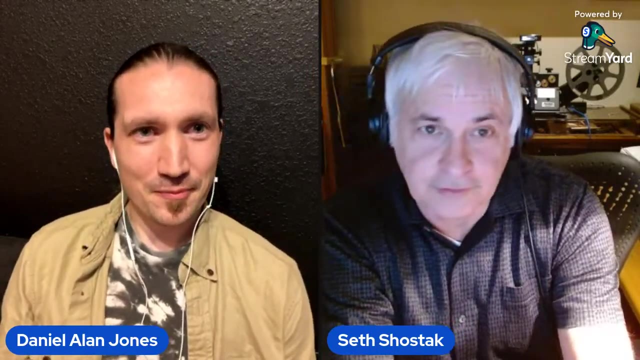 signals. So this seems like a really exciting type of experiment. How is this uh taking place And and what do you imagine the the effectiveness of this type of simulation to to enable for for future work to be done? Well, we only simulate signals, you know. 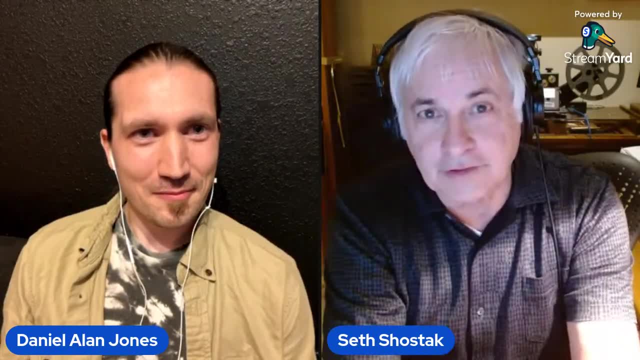 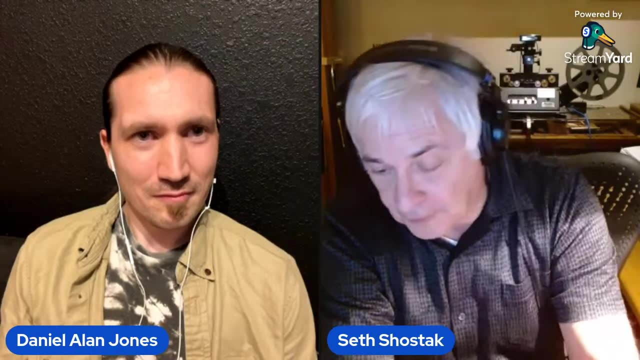 not that you've. I mean, we do it simply because it's a good way to test your system. You're trying to pick up signals, right, And we haven't found any signals so far from the aliens, So we'll just build this box over here that produces signals that we think would be typical. 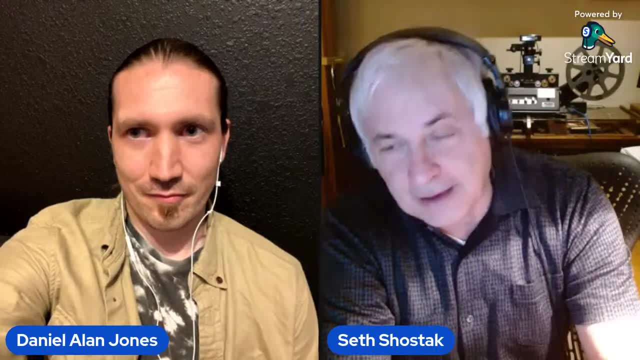 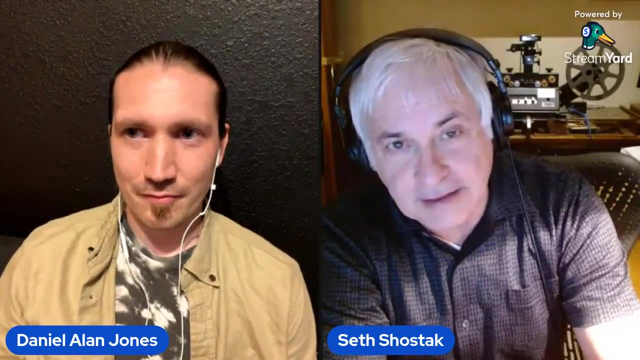 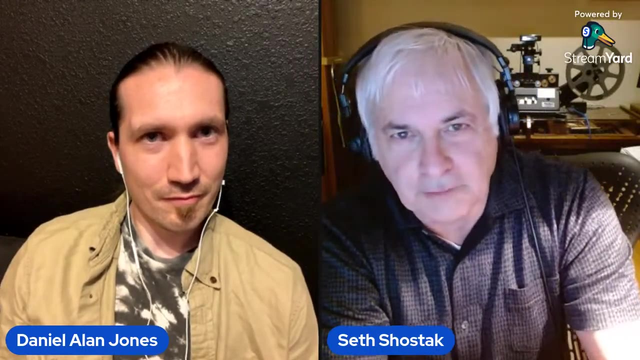 for another society to send into space, to transmit, And that allows us to test our equipment to make sure that we could find the kind of signals that our device makes. So it's like any other sort of testing that you might do. you know, you essentially build a model of what you're. 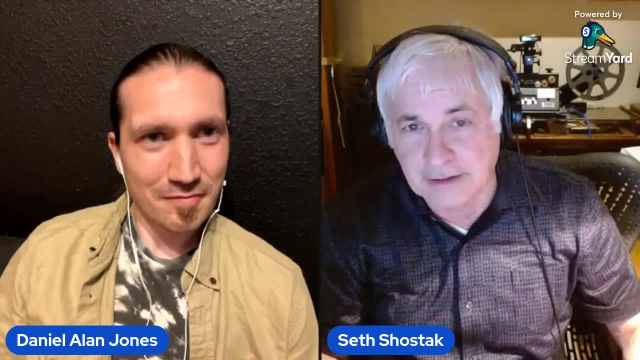 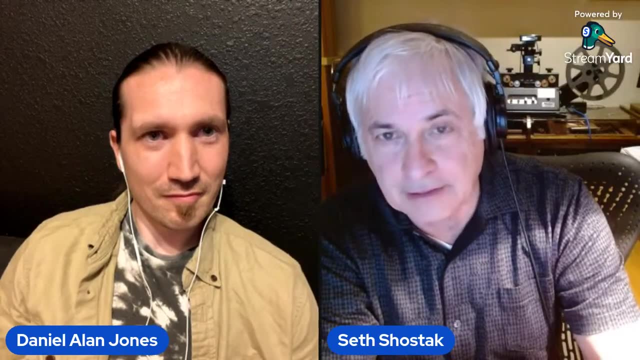 looking for and you run that against your equipment to see if you can find it. That's the way it works. We actually are applying artificial intelligence, AI modeling, some of the searches, in fact, all the searches now that we do, But you know that's a technical. 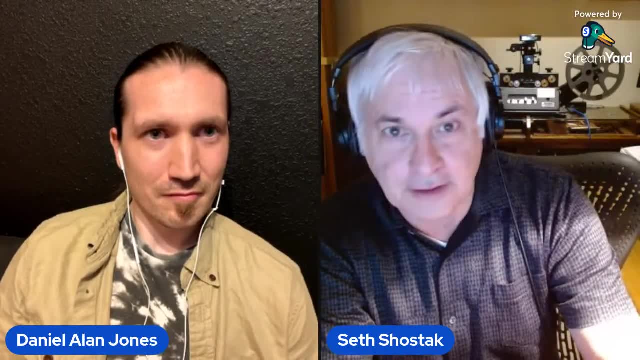 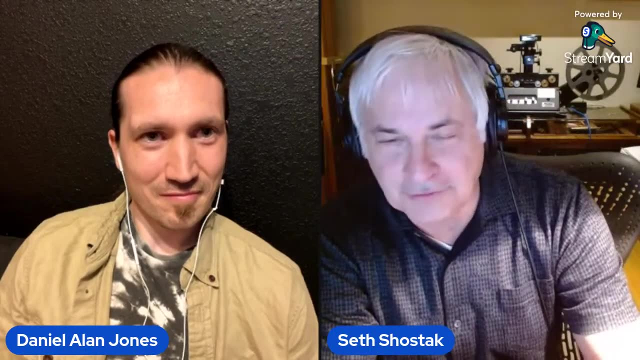 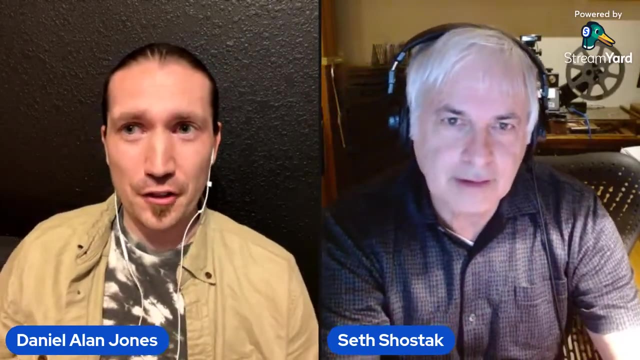 aspect that improves the ability to find weak signals on a planet where there are an awful lot of transmitters trying to, you know, getting in your way if you will, But that's a technical thing, Right? Well, when it comes to the technical aspects- and there's a lot of the techniques- 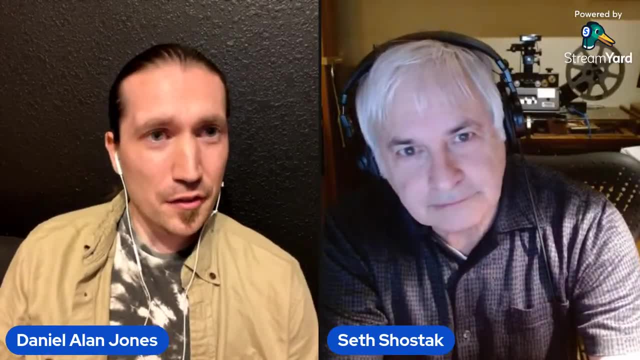 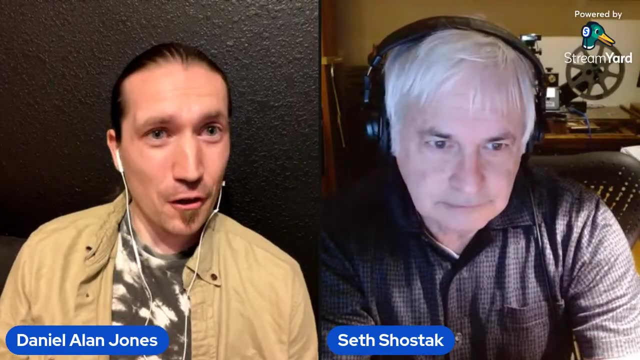 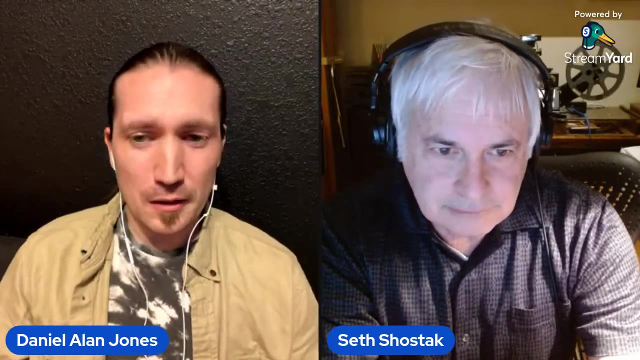 the methodology to utilizing the various equipments that are at work. it looks like with the Very Large Array in New Mexico there's a lot of, you know, potentially promising results And with that underway, what are your aspirations on how something like the Very Large Array there? 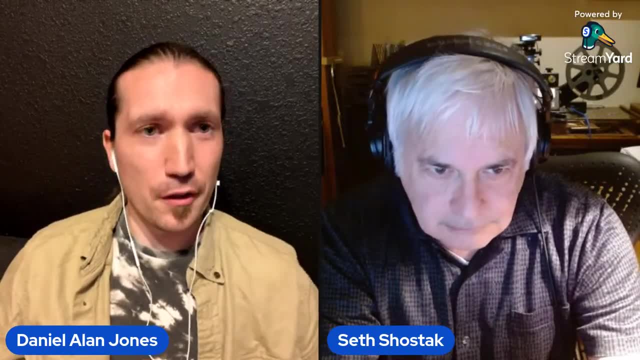 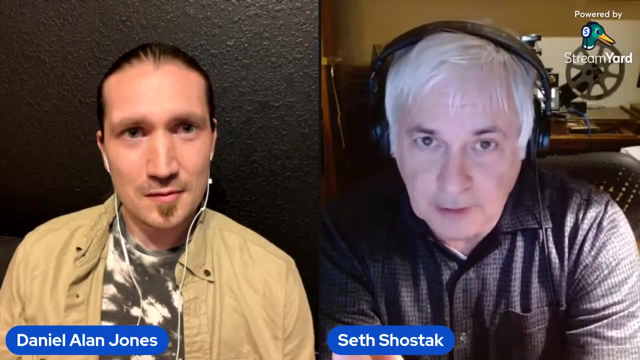 in New Mexico can come into play and serve some use with SETI's work. Well again, the idea here is: we're trying to eavesdrop On signals from others, And if you have a bigger antenna then you can, you know, respond to weaker. 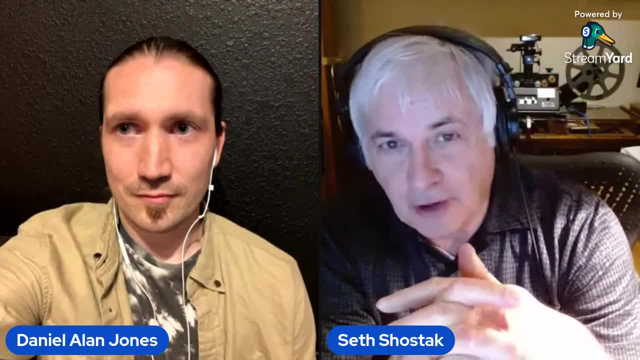 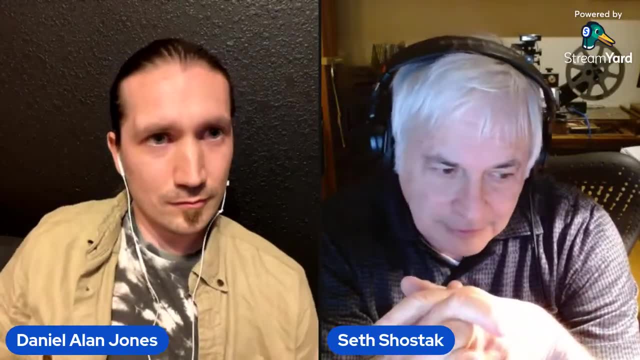 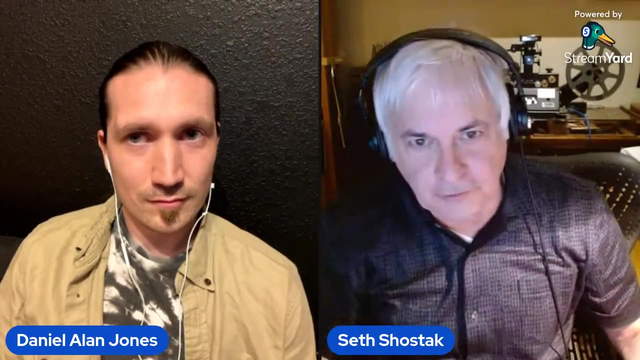 signals, You can find them right. If your antenna is small, you won't find the weakest signals. You just won't have enough sensitivity to do that. So the idea here is that, okay, you know you want to increase the chances that you'll find something. The Very Large Array in New Mexico, it's 27. 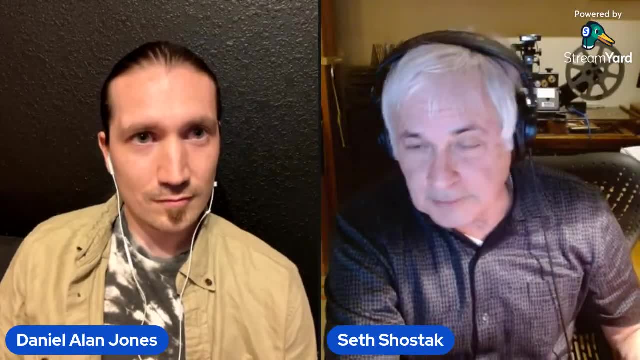 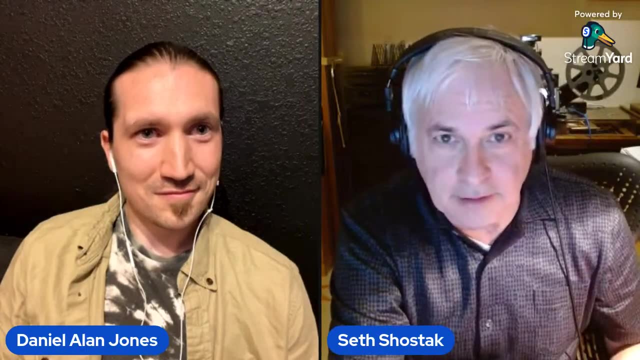 antennas. Each of those antennas is as big, if not bigger- Slightly bigger, I think- than the antenna that Frank Drake used for the first SETI experiment. But there are 27 of them. So you gang them together, work them as a team and that gives you. 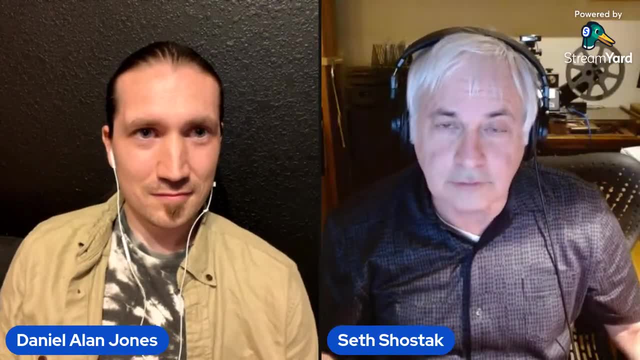 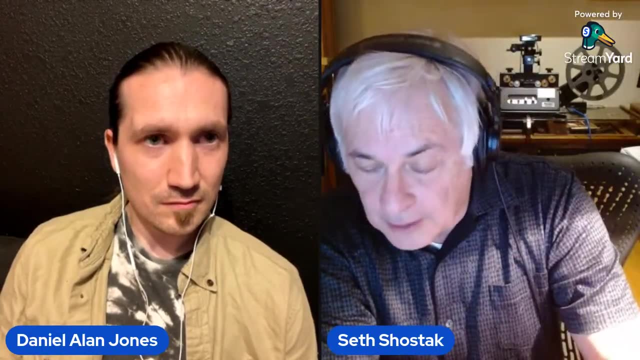 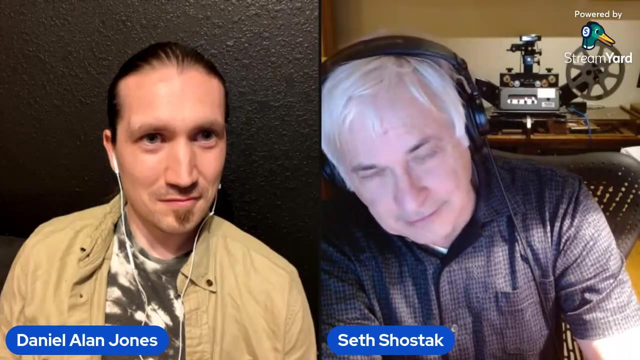 additional sensitivity. So these are again are schemes that you use to try and maximize the chances that you'll find something. What's worth pointing out here is that when I joined the SETI Institute, that was 19,. it was about 1989. It was still a NASCAR. 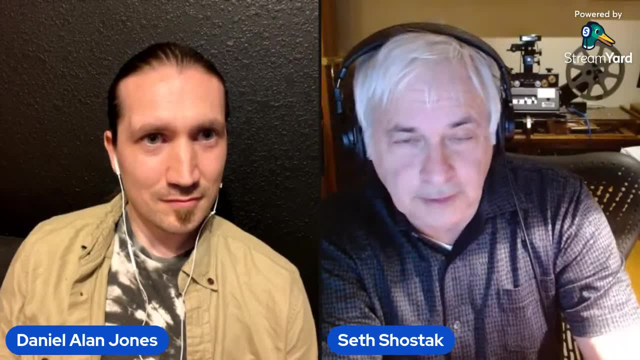 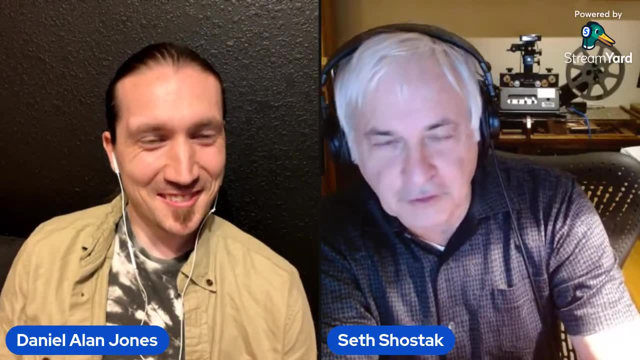 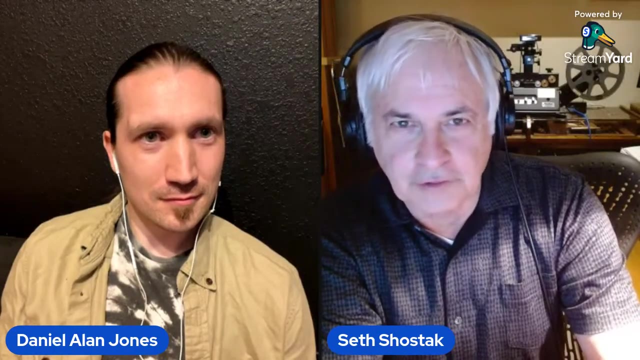 It's a project, But a congressman from Nevada. kind of curiously enough, about two years after I arrived in California, this congressman decided that he needed an issue to prove to the voters of Nevada that he was trying to save them money. So he introduced a bill late at night that killed 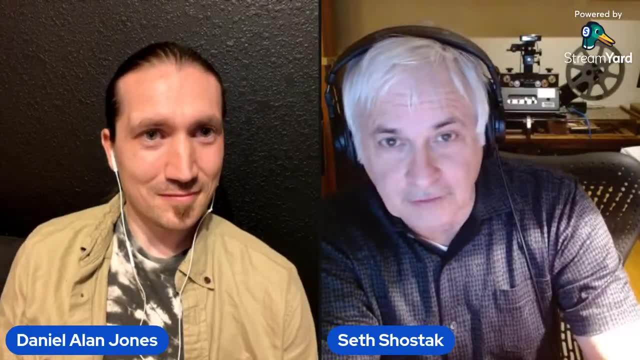 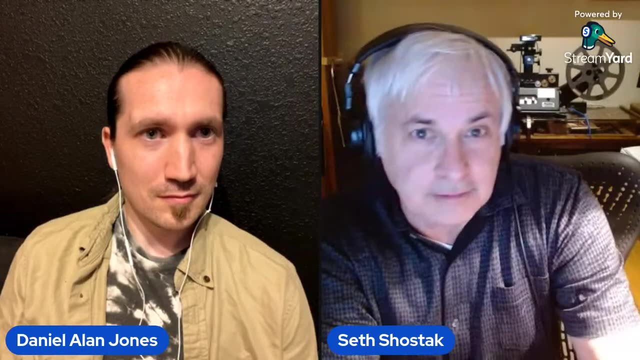 the NASA SETI program. So that was the end of that, actually, And you know that ended NASA's participation in the program. But we could just, you know, keep going as long as we could find enough money to pay the people that were involved And one of the projects that we're working on. 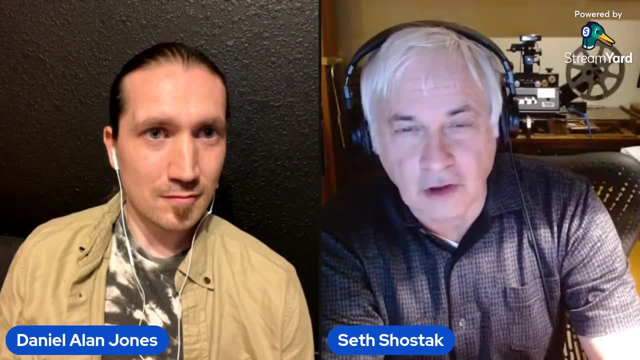 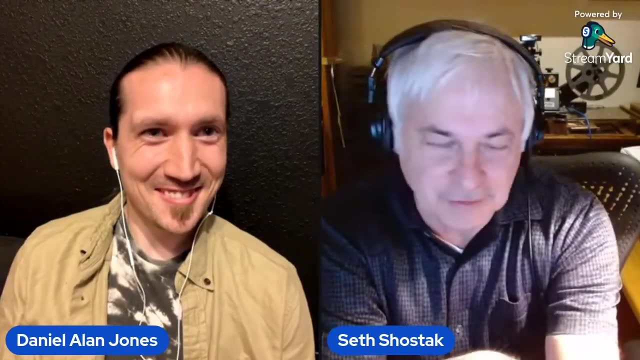 this year it's already begun- actually is called COSMIC. That's a very tortured acronym that stands for well, you can look it up But I don't ever remember what it stands for. But the idea there is to sort of piggyback on experiments running on the very large array. 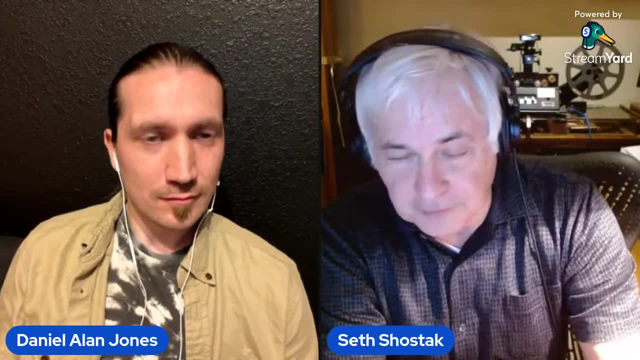 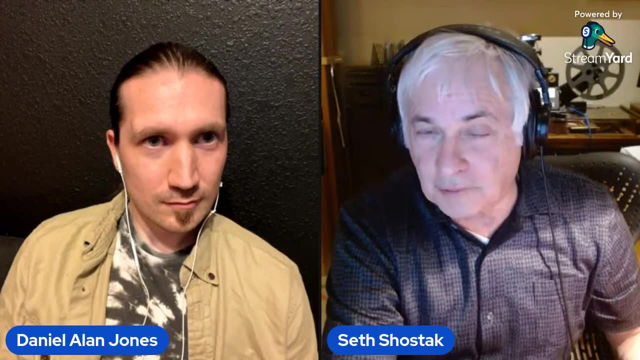 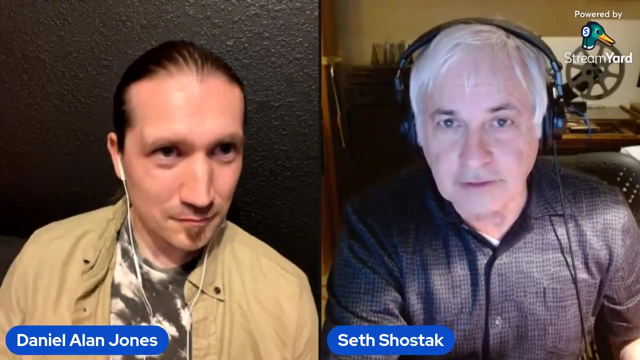 in New Mexico right Not to look for quasars or pulsars or anything like that, But just to piggyback on the receiving system of that 27-element array in the New Mexico desert and pass it through the kind of equipment that would allow us to find a signal that could be. 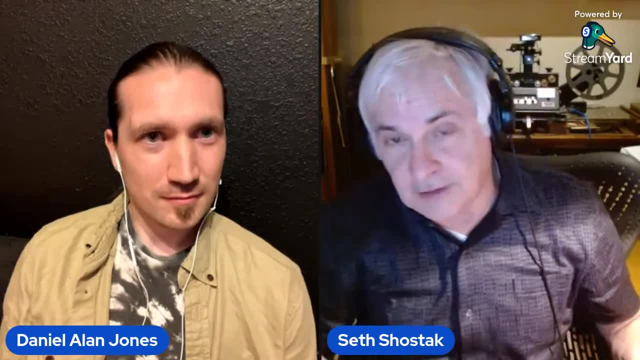 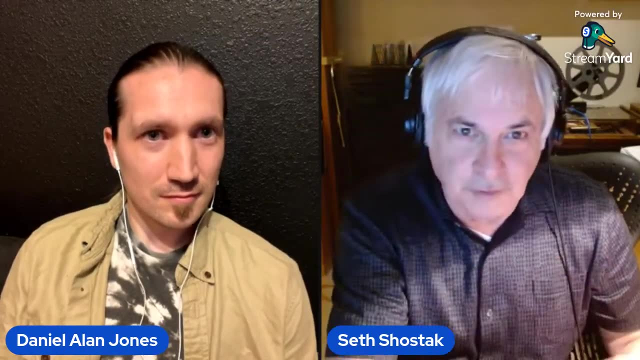 due to a deliberate transmission from elsewhere. So that saves you the expense of having to build and maintain- you know, a very, very large instrument. if you can, you know if you will share that instrument with somebody who's already using it for other purposes. 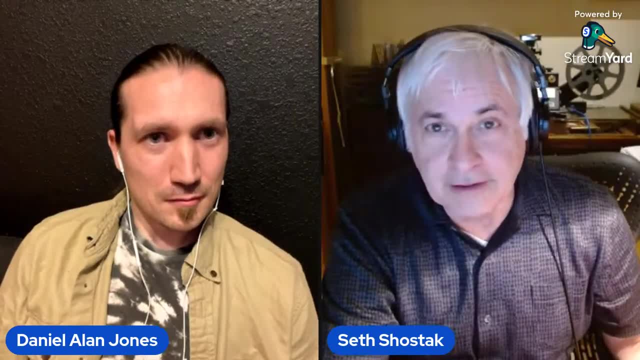 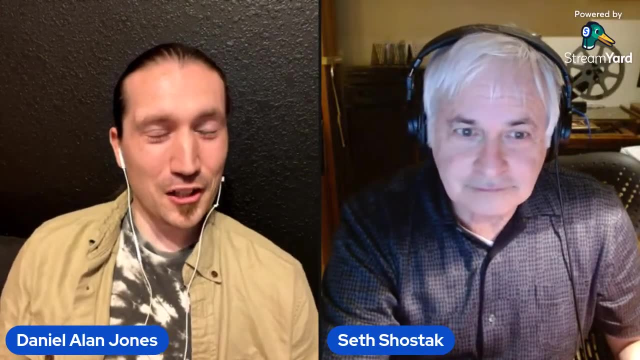 It doesn't mean you can't choose where you're going to point the antennas, But on the other end we don't know where ET is hanging out anyway. So maybe that's not such a big loss. Sounds like a fascinating collaborative effort. And when it comes to the deserts of New Mexico, 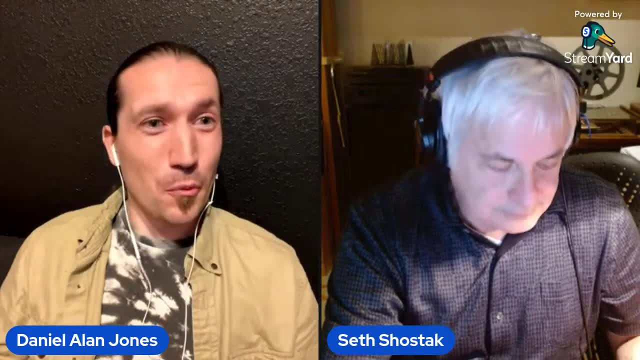 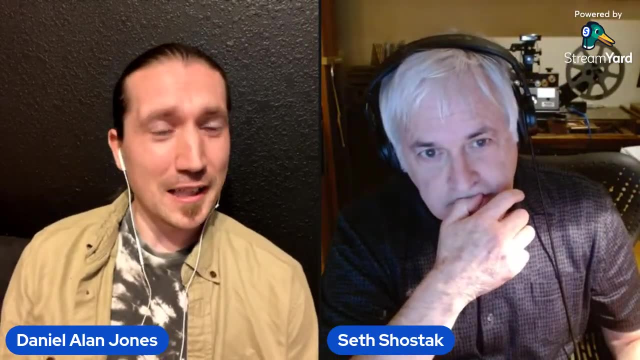 people often wonder: have aliens visited here at some point in our recent or distant past? And when we see things as you just mentioned, with NASA jumping into the game of investigating what is now referred to as UAP- Unidentified Aerial- 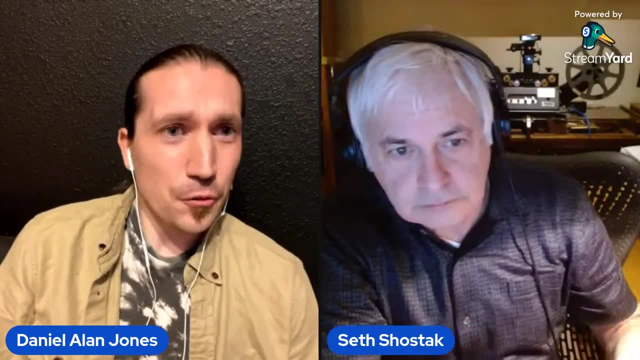 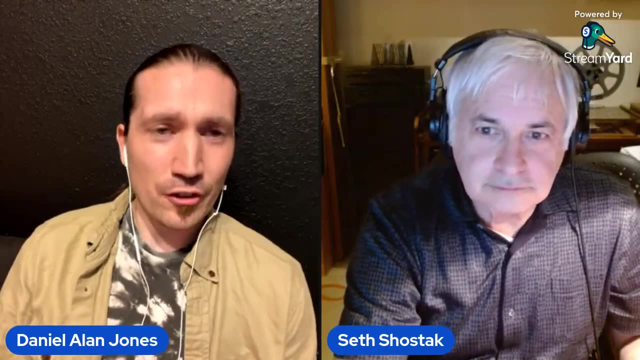 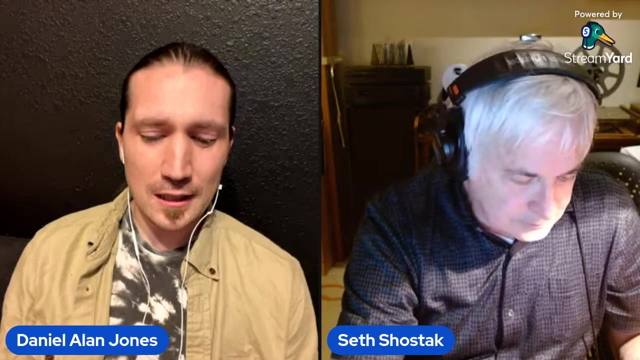 And now anomalous phenomena And, of course, with the history and mythos of ufology, the study of UFO reports and people who investigate these claims. do you or does SETI in any way give credence to the history of this type of phenomenon Or does it seem to be complementary to the work? 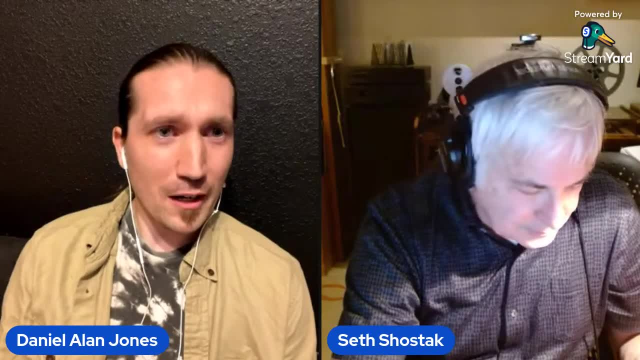 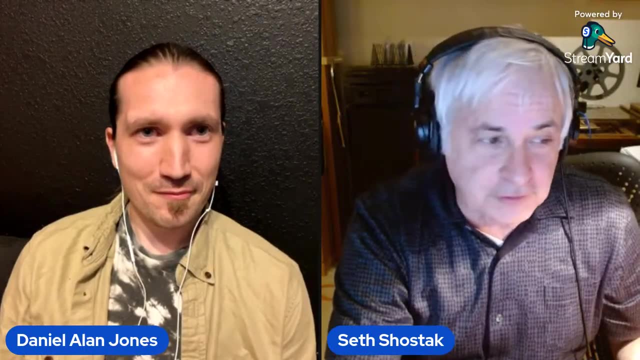 being done in an attempt to find out more about extraterrestrial intelligence. Well, this is an unpopular viewpoint, but I don't think it's a popular viewpoint. I think it's a good one. I don't think that there's any good evidence that Earth is being visited, or actually 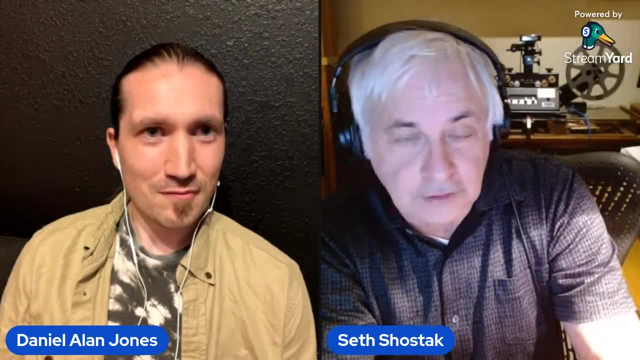 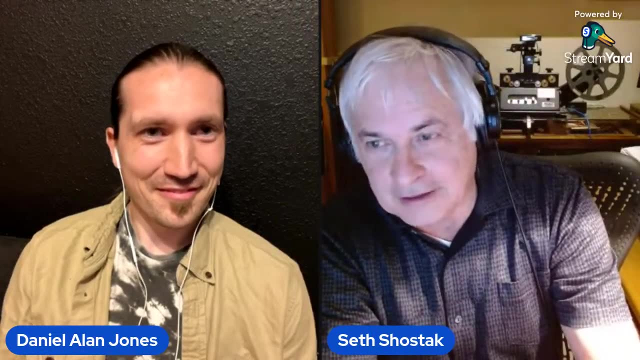 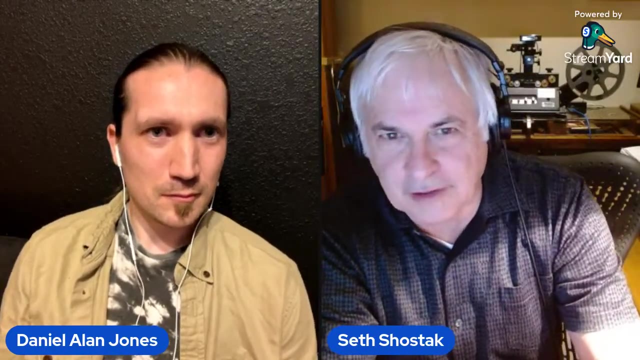 has visited Earth in the historic past. I mean, I don't know, maybe in the Mesozoic era some aliens landed here to make photos of the dinosaurs. I mean, how are you going to know? The dinosaurs didn't leave any notes behind. But as far as anything in modern times, say the last. 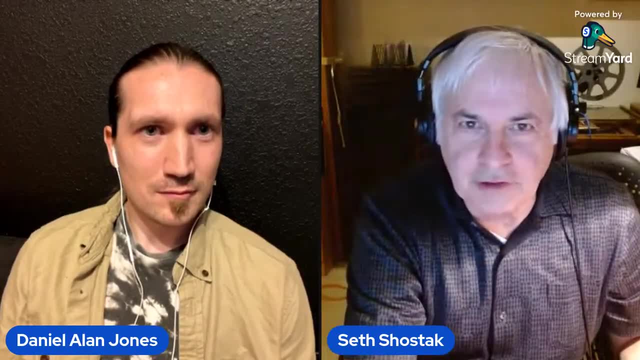 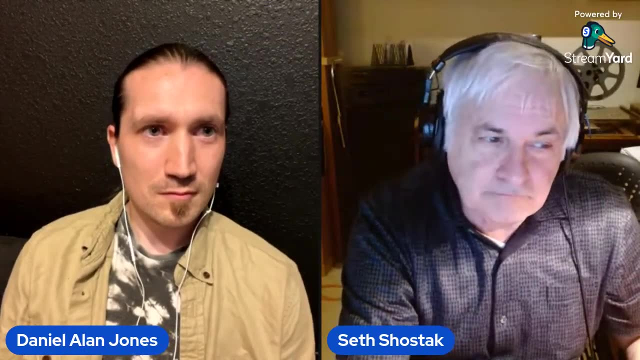 5,000 years or something like that. I don't think there's any good evidence that we've been visited. There are plenty of stories people will tell you about And polls show that roughly a third of Americans. I think that's the correct fraction. 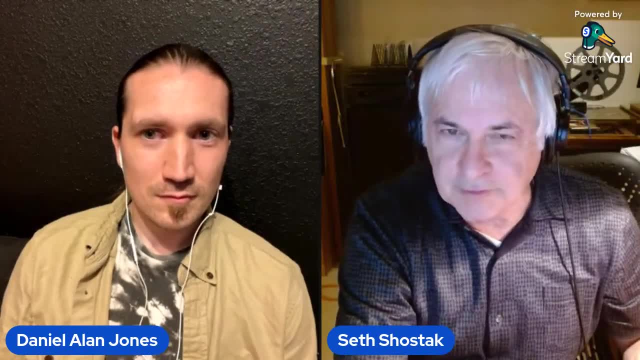 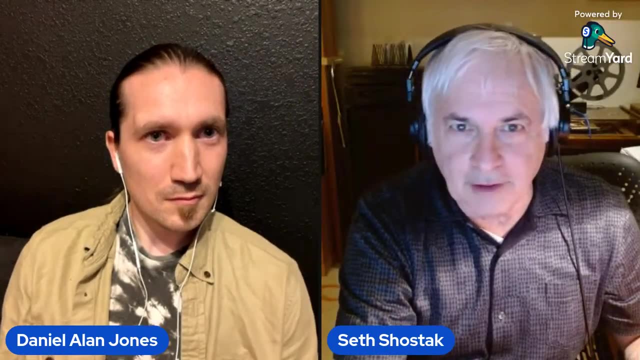 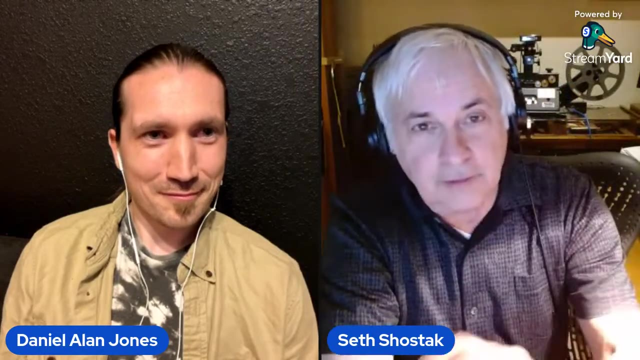 believe that not only are the aliens out there- most Americans believe that- but about a third of all of the American public believes that they have visited Earth, that they made a navigation error and crashed in Roswell, New Mexico, in 1948, whatever. But I think that if that were true, 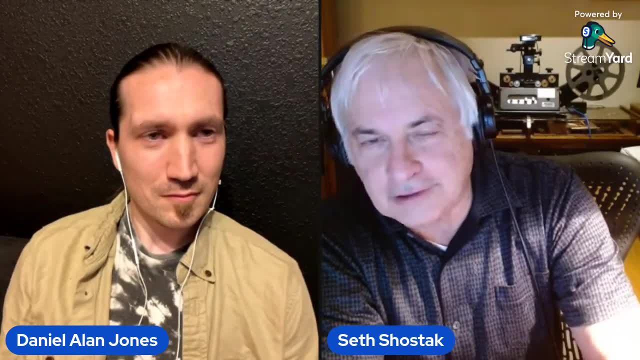 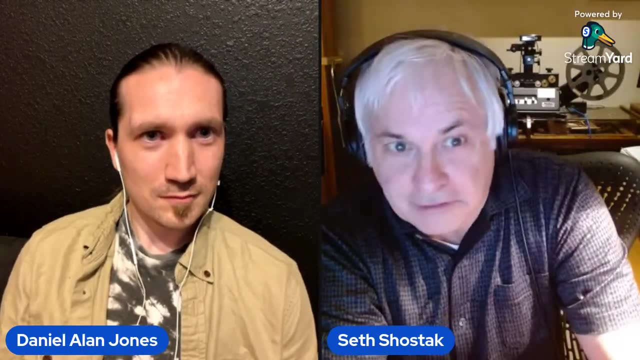 the proof would be in the fact that you you'd have lots and lots of scientists working on that right, Because that would be really interesting, I mean, if the aliens actually came to Earth right in modern times, post-war. 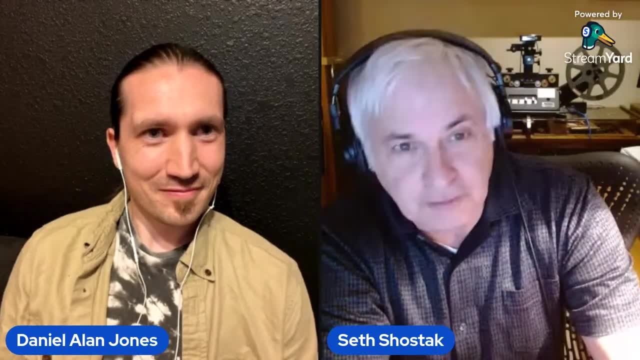 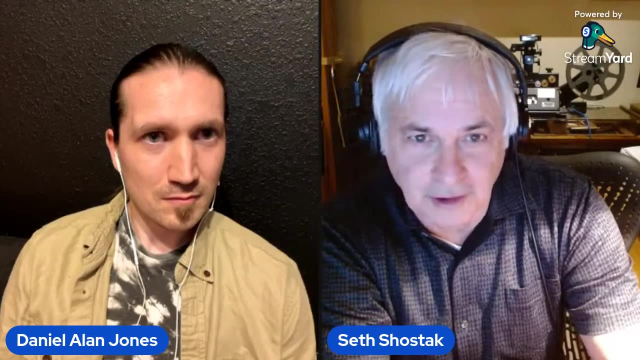 they came to Earth. you know that would be. I mean, it's hard to imagine too many stories more interesting and compelling than that. But you know, if you actually look around and say how many scientists are working on that idea, The answer is not very many, right? Because the 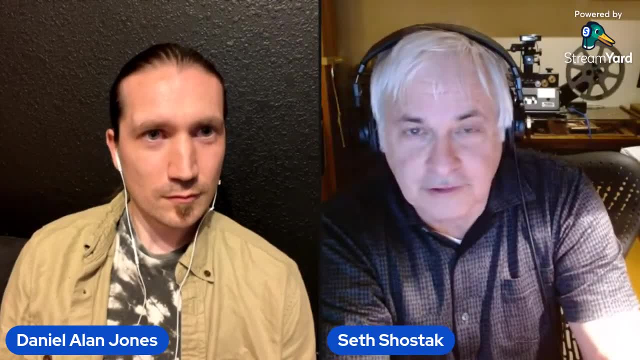 evidence is not very good. The evidence mostly consists of just stories, right, And stories are not very good. And so you know, I think that's a good question, And I think that's a good question convincing evidence or any fact you're trying to establish. 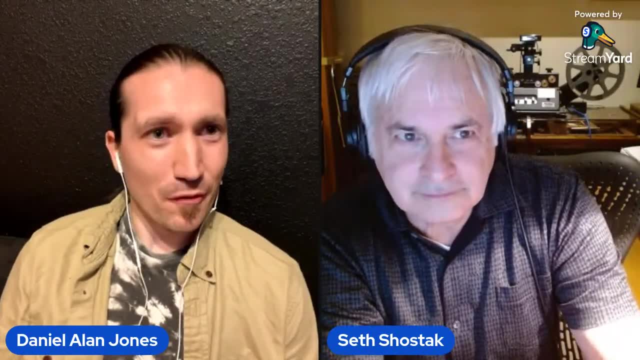 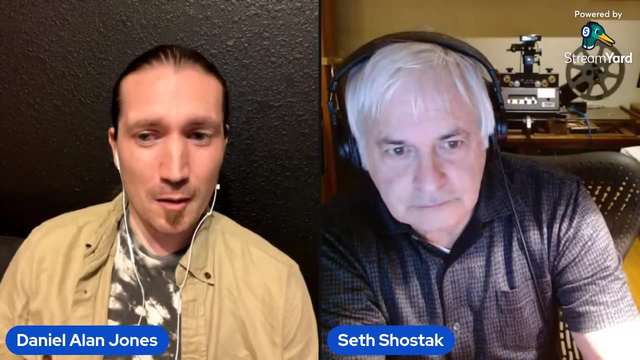 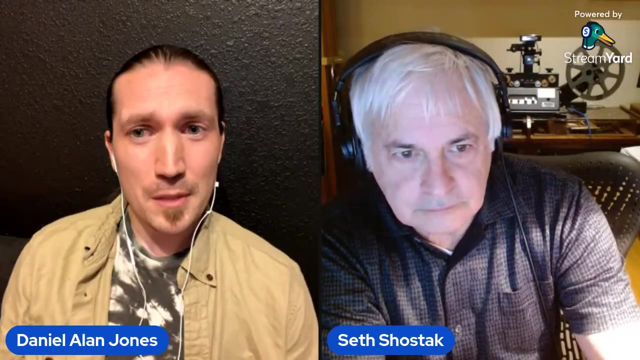 It doesn't seem like it might not be. it might not be viable for research data for purposes of scientific pursuits, And many of those claims are very anecdotal, Although some are very much convinced that ideas of alien encounters are real and that people attempting various modalities of 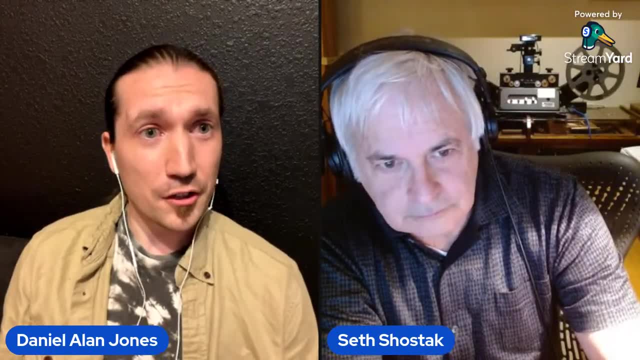 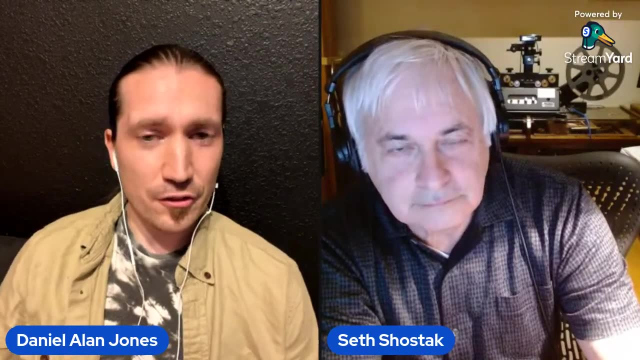 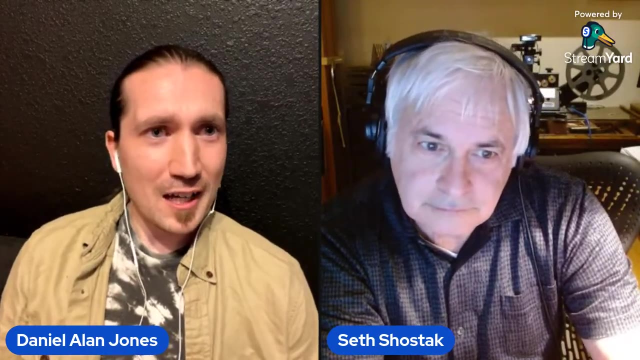 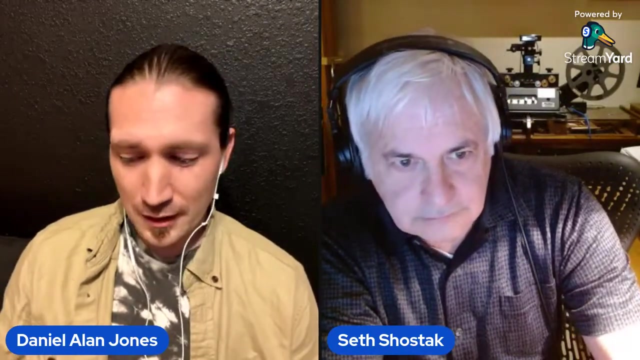 contact are experiencing something which they consider non-human in origin. When it comes to these accounts of people utilizing various techniques and an attempt to generate some kind of connection or communication, does this seem to be something that would be considered if there were a demonstrable effort that was underway, under scientific, controlled demonstration, that showed 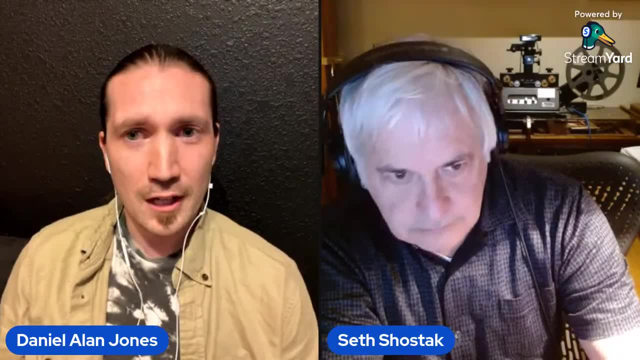 effective results. Would this be something you or SETI would consider looking into? if those out there who ascribe to these modes of communication would be considered? Would this be something you or SETI would consider looking into? if those out there who ascribe to these modes of communication? 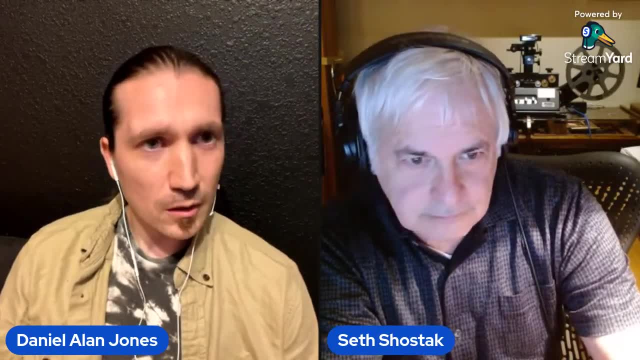 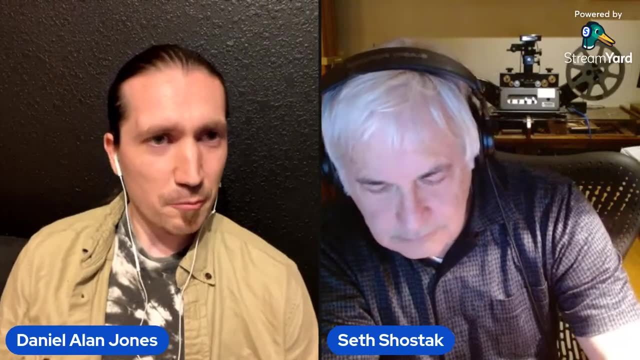 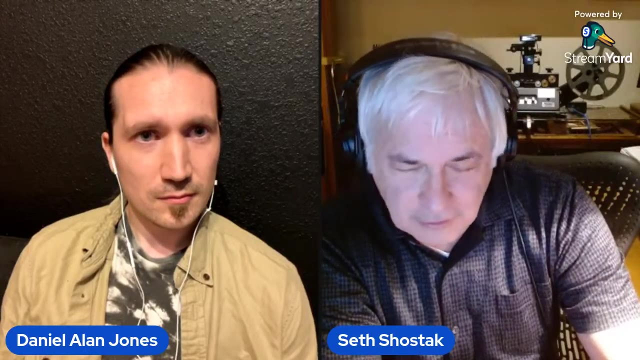 conscious contact, of human initiated contact experiences. is there anything that that you might be able to lend scientifically to those types of pursuits? well, i mean, it's being done, actually right, it's being done by a physicist, an astrophysicist, more more accurately, at harvard. 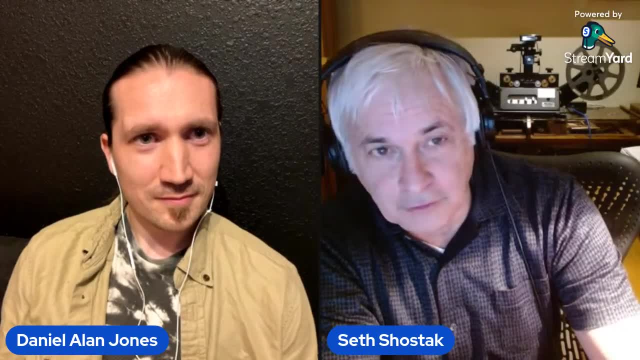 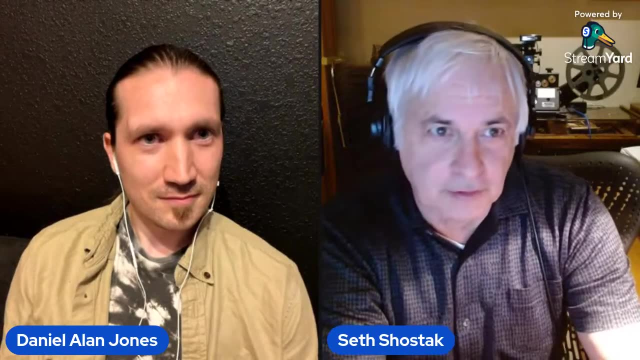 avi loeb. he's very, you know, intrigued by all these ufo reports, and so he said, you know, the whole problem with the ufo story is that it's, you know, it's mostly promulgated by people who don't have much science training, he says, and the scientists just sort of dismiss, dismiss it. 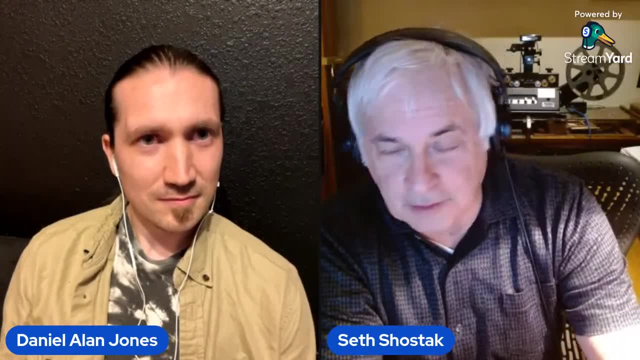 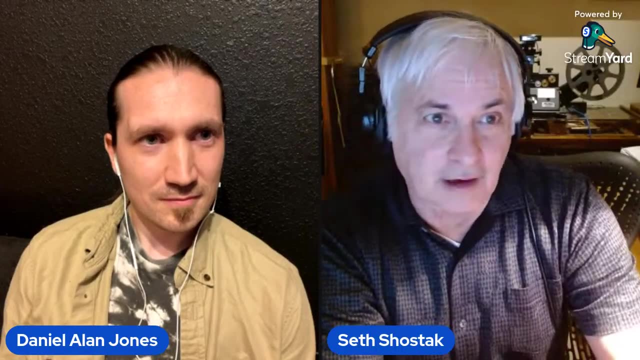 and he thought: well, why don't we just do the experiment? you know, you can believe me, you cannot believe me, but if you do the experiment and you find something positive- in other words you find evidence of visitation, for example- that becomes science when somebody else can do the experiment. 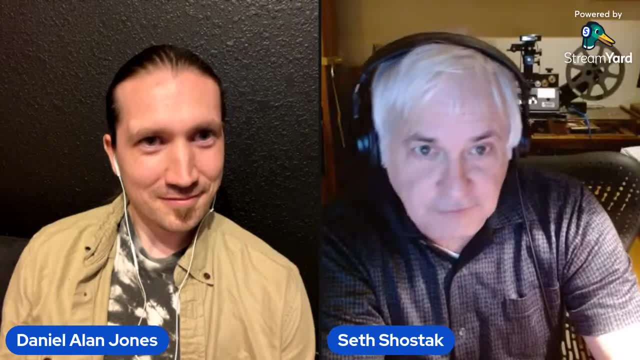 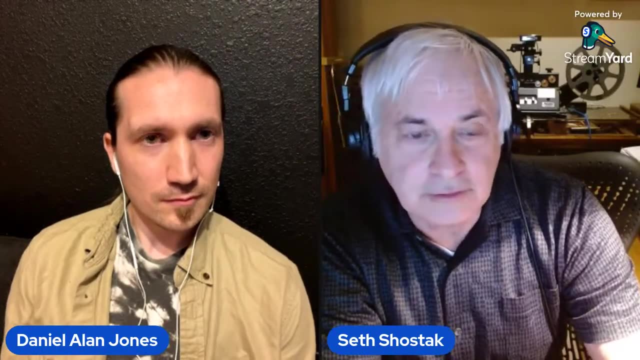 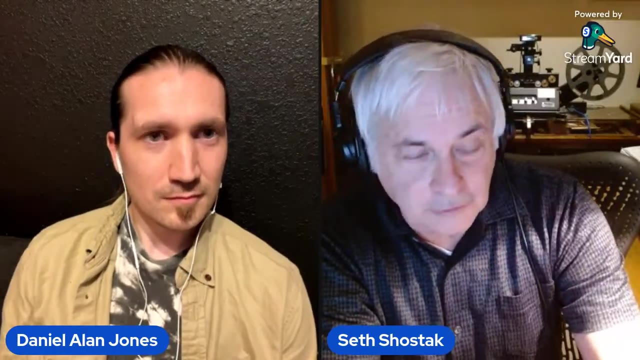 and find a similar result. right. it's not a matter of convincing people with your arguments, because those don't really amount to much in science. it's a matter of: can you take data that shows that you know we're being visited, something like that? so, uh, avi loeb has a project. it's called the galileo project. uh, he's raised some money. three: 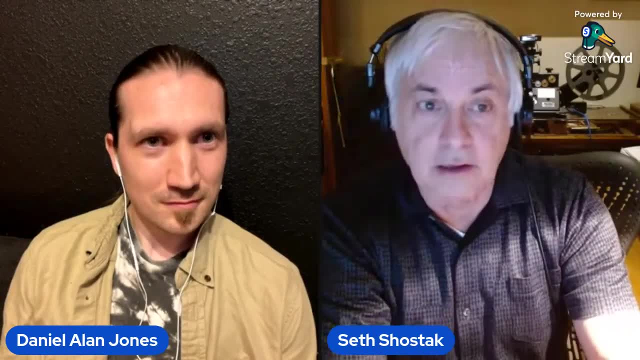 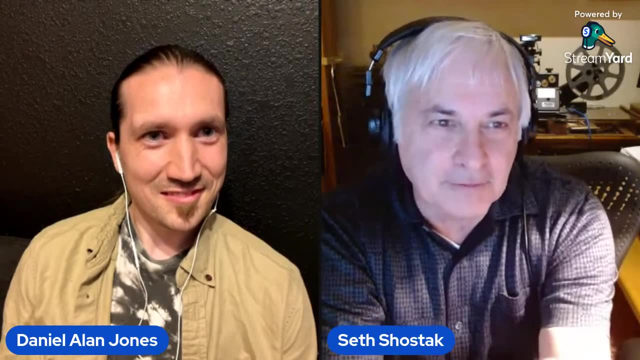 million dollars thereabouts to build equipment to do exactly what you say. uh, he's going to. you know, i mean, this is this equipment's all going to be on the rooftops of harvard university, but it doesn't matter, right, because we don't know where the aliens are anyhow. so it would be. 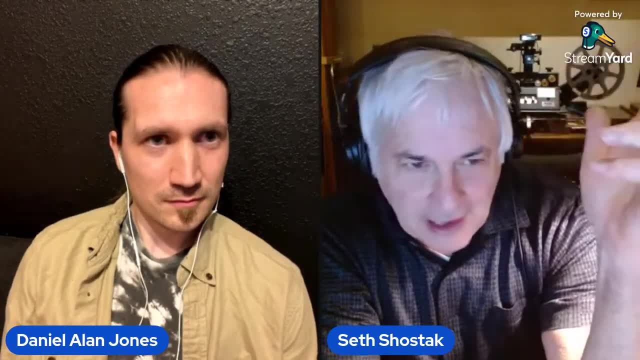 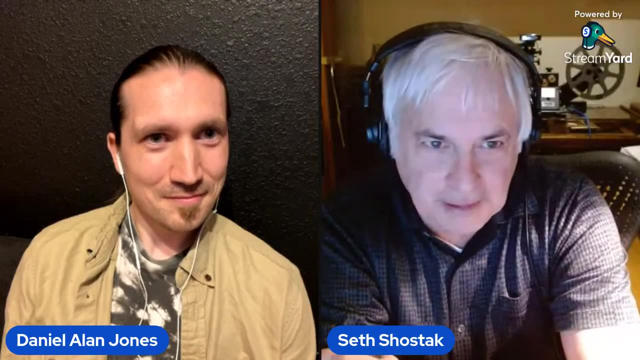 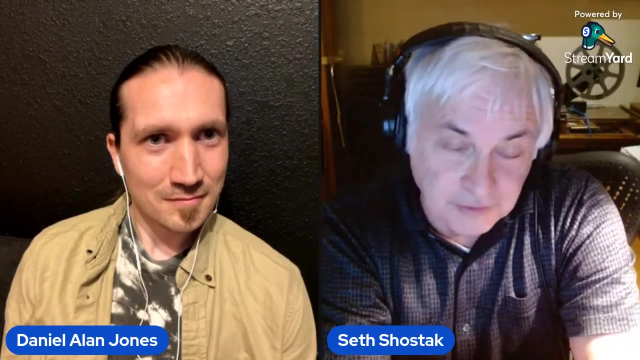 equipment that would be sensitive to, obviously, radio waves and light and stuff like that, and if there really is evidence in front of our eyes of aliens visiting the planet, we'll we'll be able to see them. i'm personally, uh, actually pleased that somebody- that avi loeb- is doing this. i don't think. 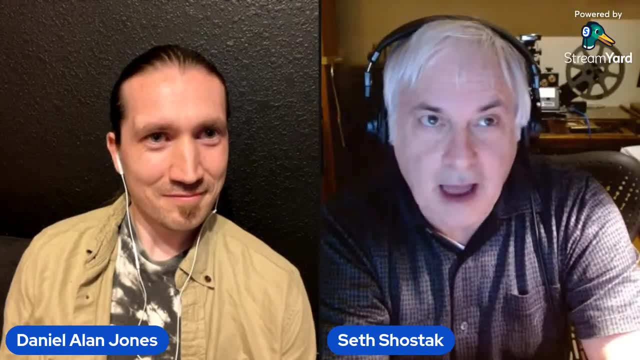 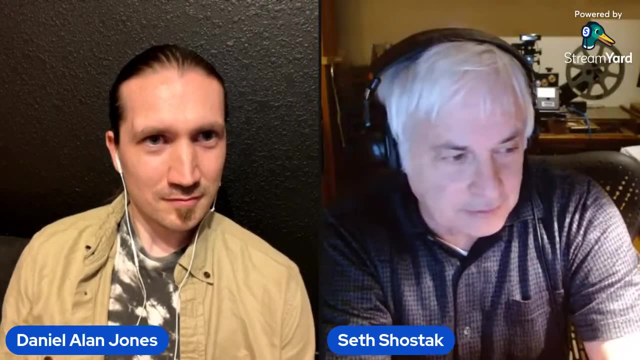 he's going to find anything. i think you know we have 8 000 operational satellites orbiting the earth right now and most of them have cameras looking down and they don't see anything. and the the usual rebuttal to that observation is: oh well, you know, the government's keeping it secret. but 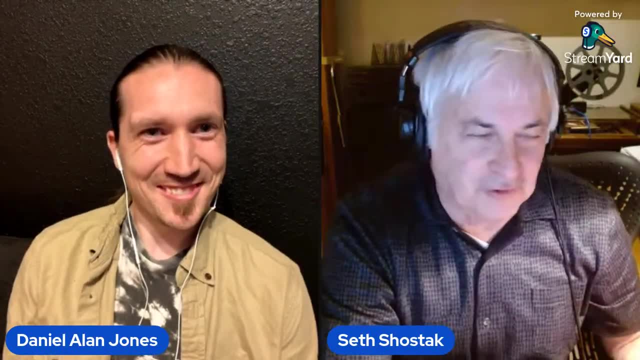 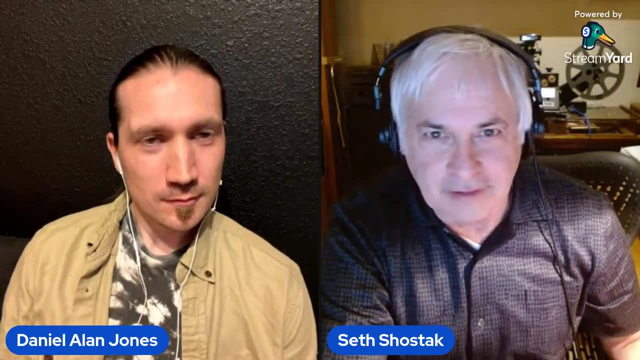 i've worked for the federal government. i had a secret clearance for the federal government and you know there was nothing that i knew that you couldn't just give away to well at the time the soviet union, and it wouldn't have made any difference. i mean, so i, i, you know, i'm skeptical. 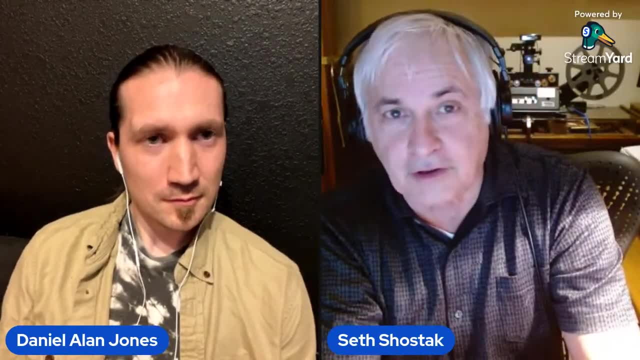 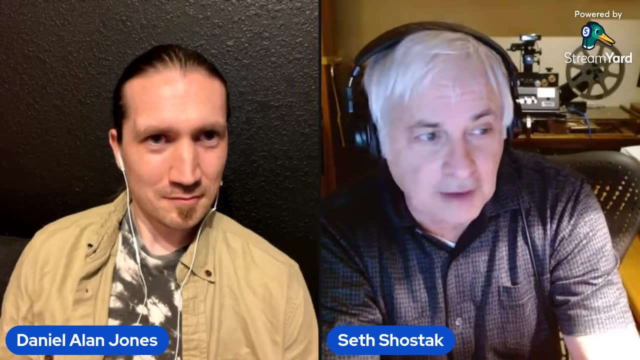 i'm skeptical, but it doesn't matter whether i'm skeptical or i'm not skeptical. the facts are that this experiment is being done, it's going to be done. they're building some equipment, designing equipment to do this, and i i fear that it probably the most predictable result of all, that is that 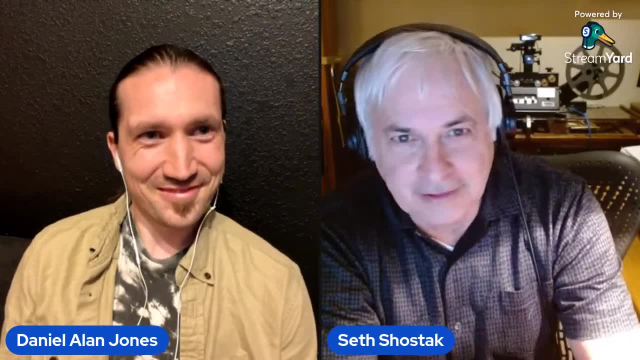 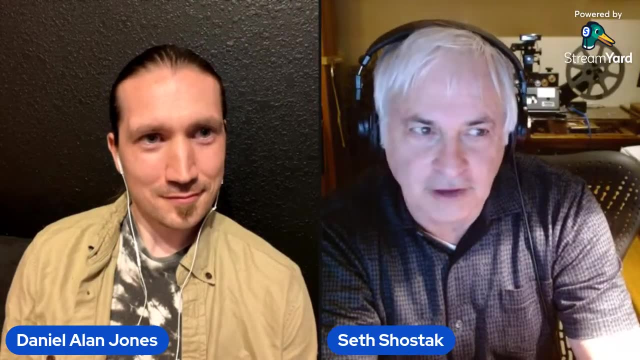 it'll take a lot of the fun out of the whole ufo story because you know if, if they can't find any evidence for visitation, you know it's going to be pretty hard to argue that. well, i mean the government's covering it up, i mean it's an international effort. well, people seem to like. 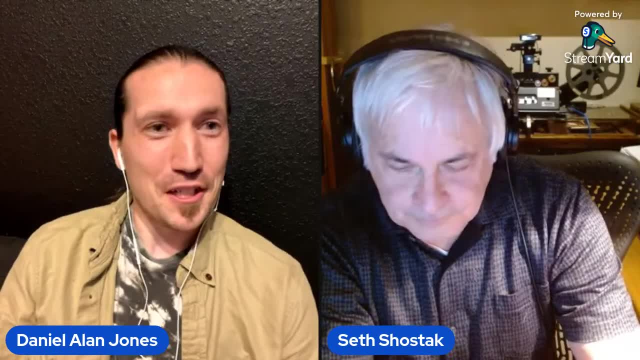 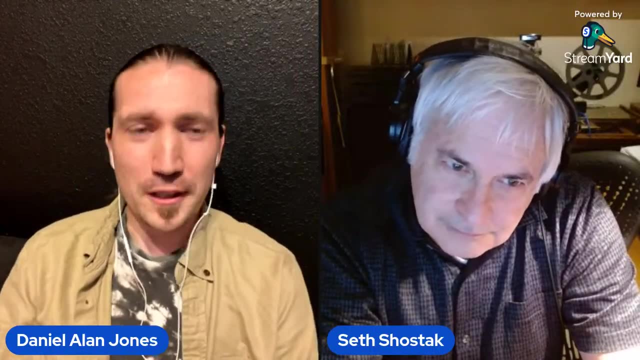 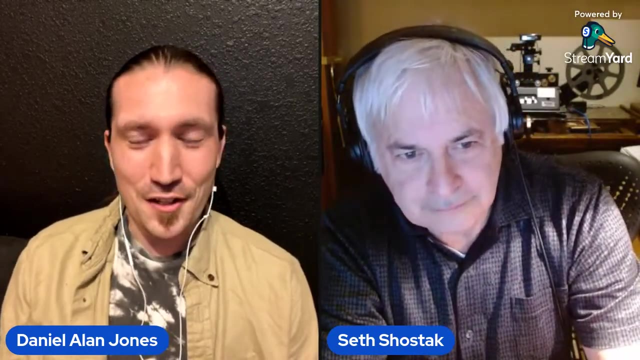 things, uh, to be more exotic than they actually are, and the issue of secrecy and defense: secrecy, um, and to posit a hypothetical to you, bringing into um the picture that people, as you mentioned, often do consider that there is some effort to cover up not only um the existence of extraterrestrial. 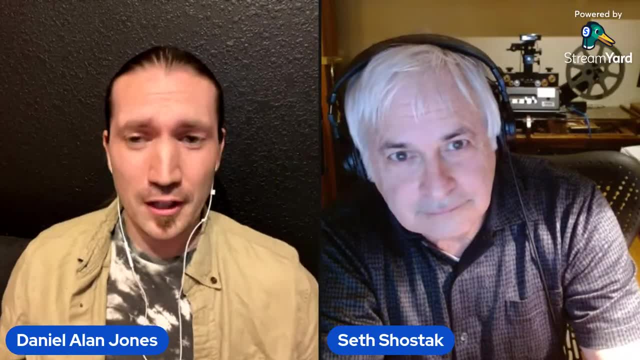 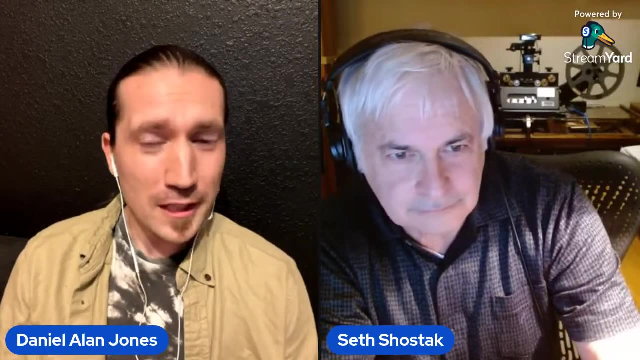 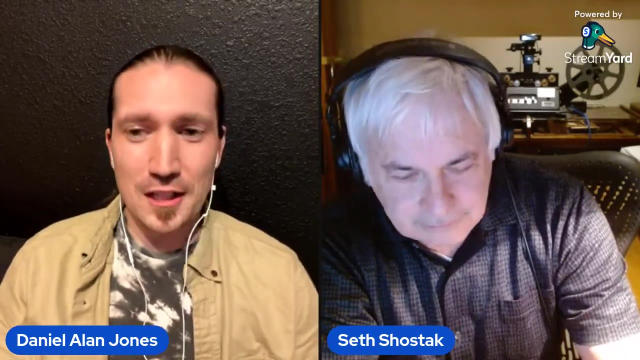 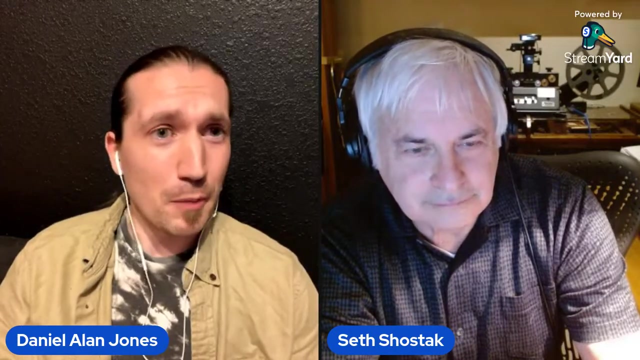 intelligence, or some non-human intelligence that exists here on earth, but that we've been able to somehow retrieve materials- uh, some debris bodies perhaps- and within this proposition, as you mentioned, the what would hopefully be the effort of numerous scientists on board to try to share what i think would probably be one of the most biggest discoveries of all of human history. 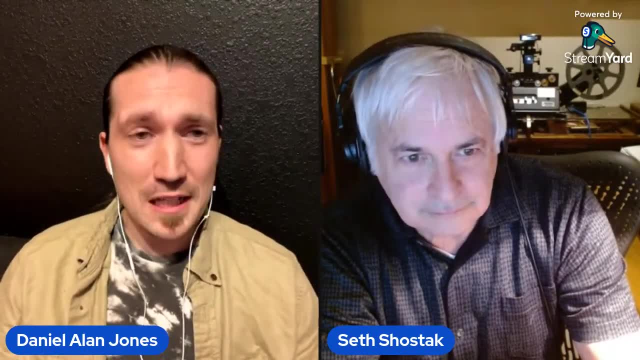 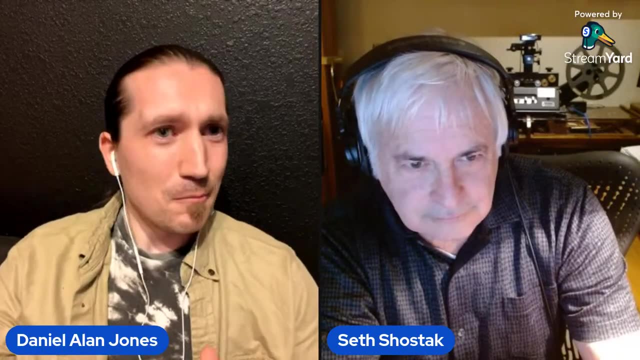 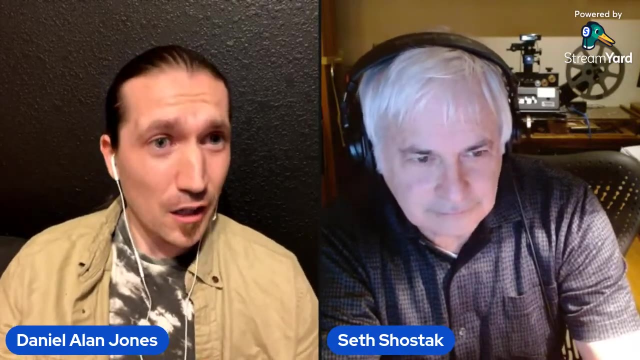 despite any of that, if, in the event that something were to actually be disclosed from the bureaucrats or the military industrial complex that says we've had red tape over this for you know, nearly a century now, or however long it is, whatever the case may be, or even if it's not government, 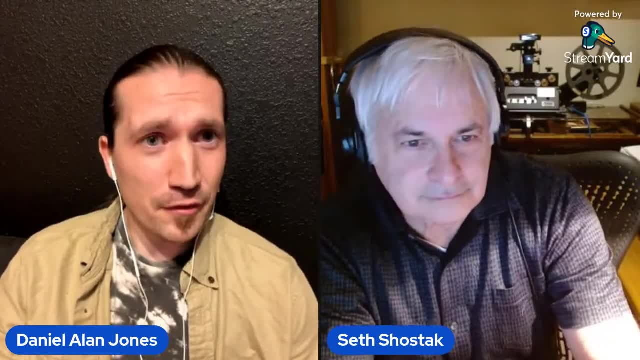 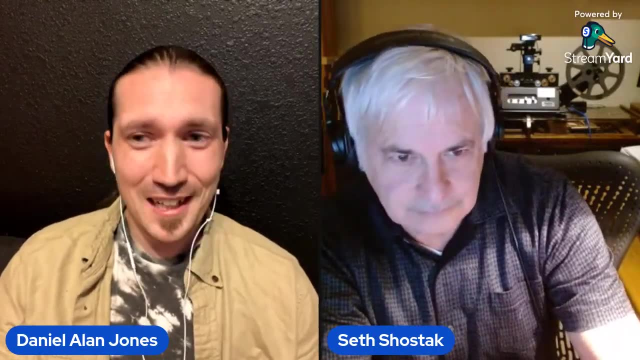 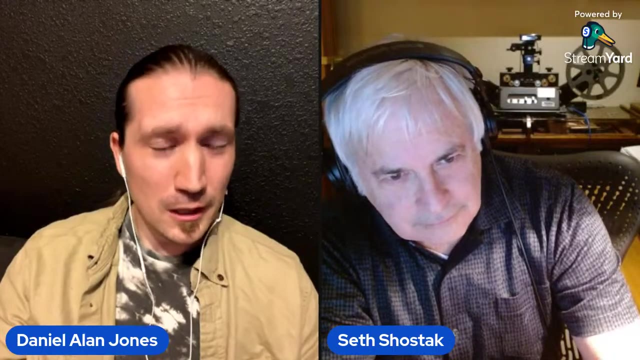 that comes forward. if someone comes forward and says we have technologies, um, and we have something, and, uh, it may even be emitting signals, uh, and have an emission uh of some kind of frequency, would that be of interest to you? would you or the SETI institute be willing to offer any? 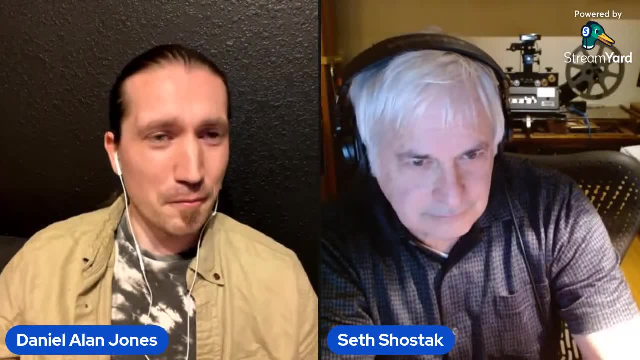 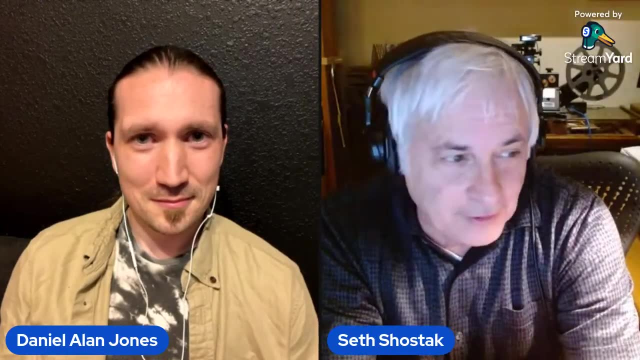 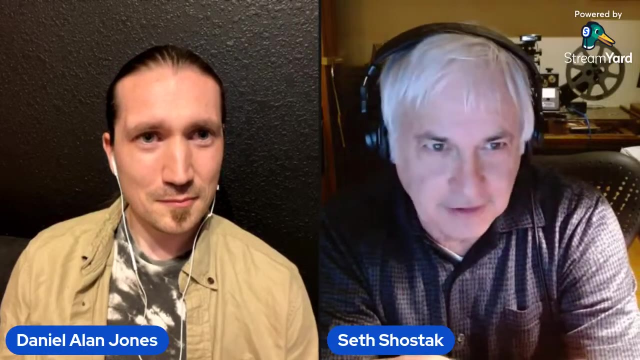 scientific assistance if, in the event, something were to be announced of that caliber? no, of course, of course. i mean, look, if there's any truth to this story. you know, um, as a theoretician, a theoretical physicist friend of mine said to me years ago, we were talking about this over a pizza dinner and he said: Shostak, if I thought there was. 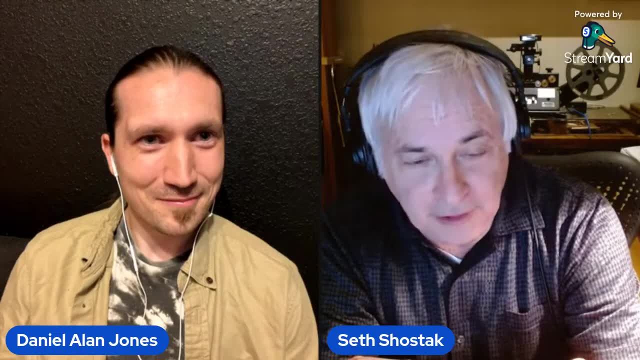 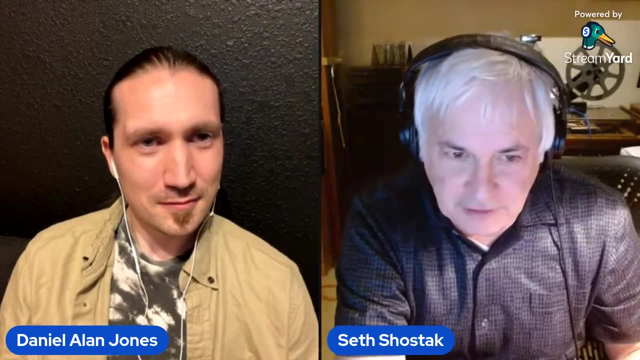 a one percent chance that any of this stuff is true, I would spend all my time working on it, but he doesn't. he doesn't spend all this time working on it because he doesn't think there's even a one percent chance that any of it is true. it would be very hard to keep this all quiet. Americans love. 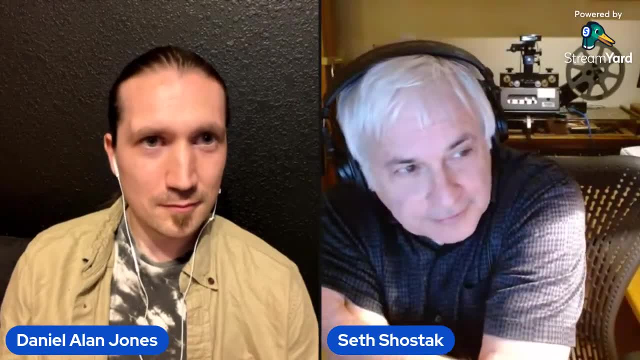 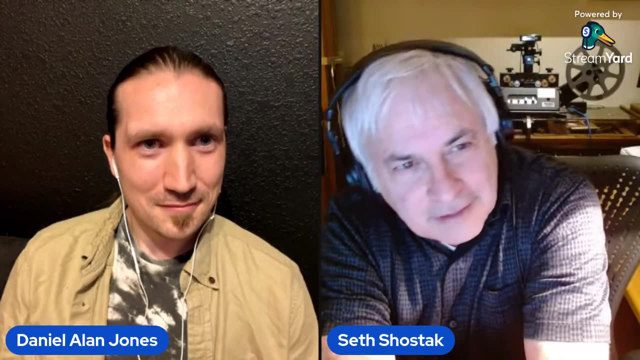 conspiracy theories. I mean, and I've lived in Europe and they're not so keen on conspiracies there as they are here. but you know, all right, so what? but but you can, you can believe on this it's, it's. to me it's very much like the. 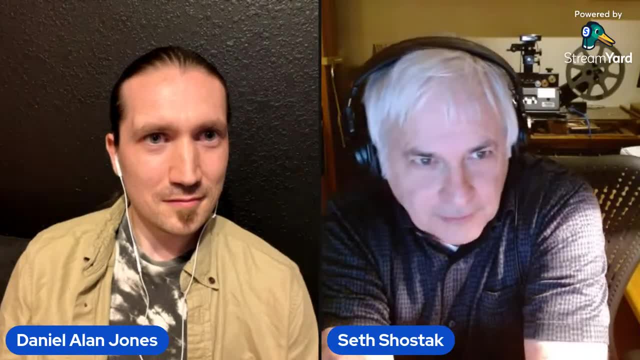 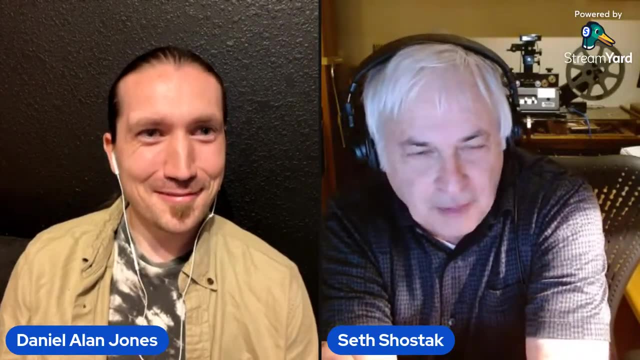 stories that you hear about how some guy developed a carburetor that doubled the mileage on his for his car right, but that the auto companies immediately bought it up and buried it right because they didn't want- or maybe I guess it's the oil companies- because they didn't want, you know. 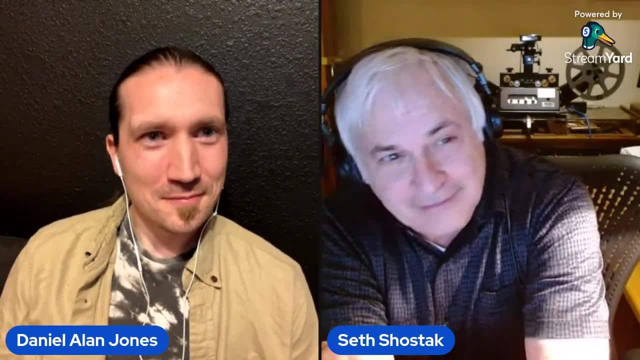 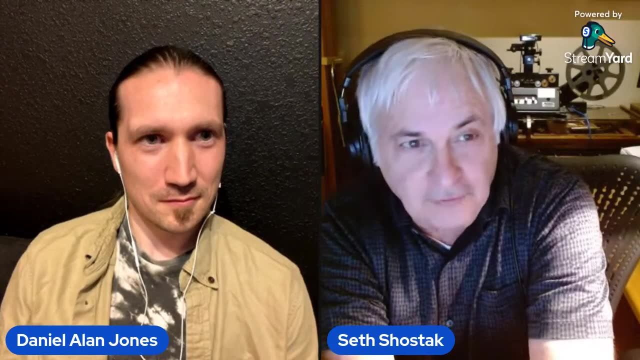 cars burning less gasoline. I don't buy that. right. if you really had a carburetor that could double the mileage in your car, I mean, you know, if I were an automobile manufacturer I would offer that as an option, right and? and even if they didn't, you know you'd have some company spring up where they just 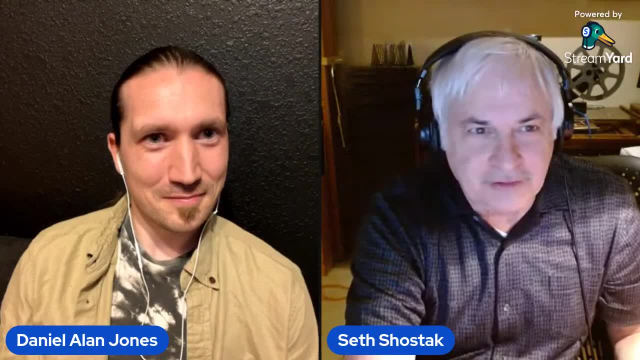 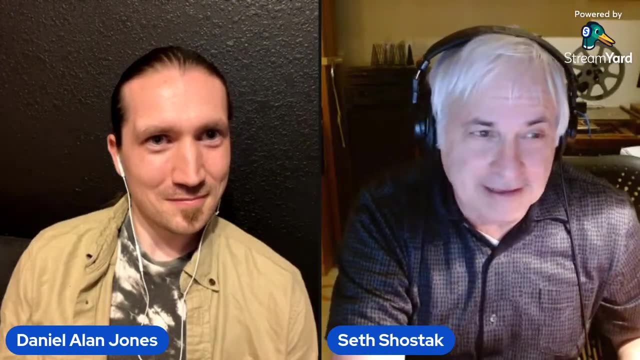 manufactured these things and sold them on the internet. I mean, you know this, this idea that if we're being visited, it can somehow be covered up by every government in the on the planet. it doesn't. it just flies in the face of the rationality it does, it doesn't. it doesn't matter what you do, it's. 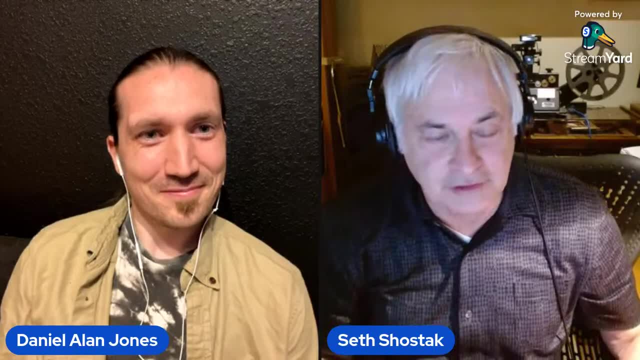 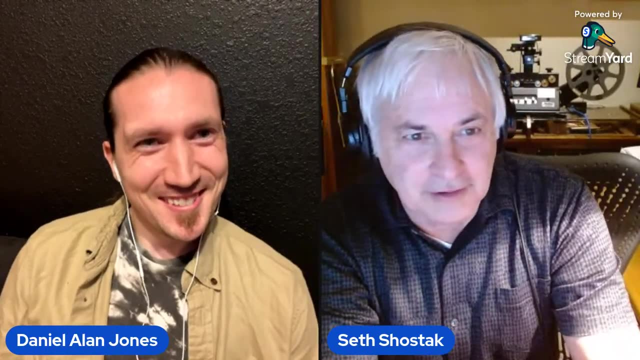 Doesn't make any sense. Doesn't make any sense. It couldn't be a more interesting story than to think that we're being visited. And, by the way, I suppose that the FAA would have something to say about it too, because maybe these aliens aren't filing flight plans. 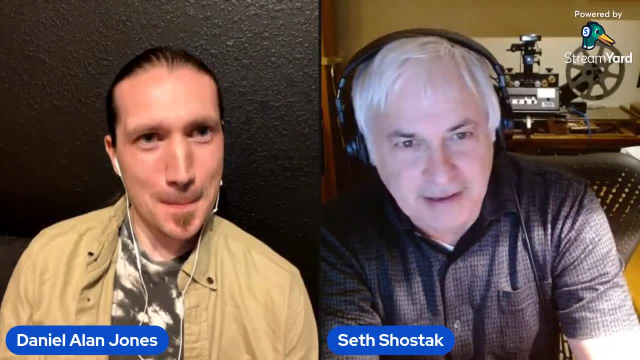 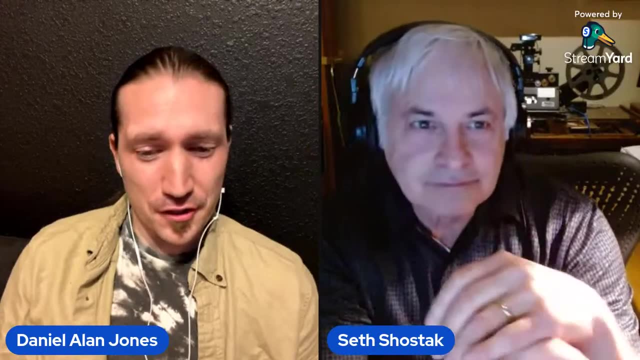 You know you take a trip to New York and you know you get intercepted by aliens. That's not a good thing to happen, Right, And that's one of the reasons why it seems like a lot of these modern iterations of some investigative effort on behalf of the government. look into these things by way of threats because it threatens airspace. Not necessarily that the aliens are threatening, although maybe some people consider that could be the case. It seems to be more or less a matter of if there are objects up in airspace. we don't want any collisions. 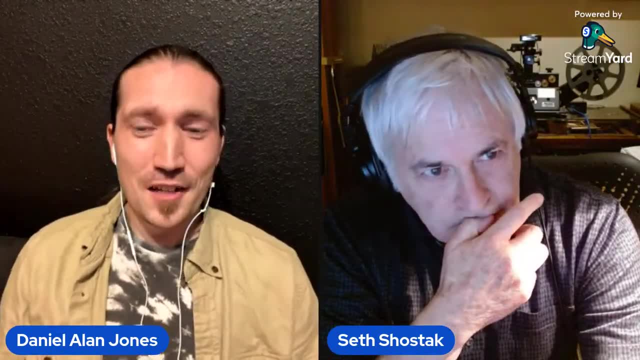 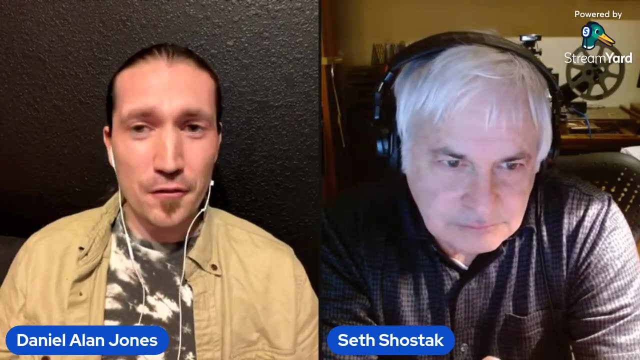 We don't want anything to happen, But people are curious and, as you said, sometimes even conspiratorial to the notion that maybe there is something. And I would say that if there is, despite all efforts, that it deserves to be in the hands of people. 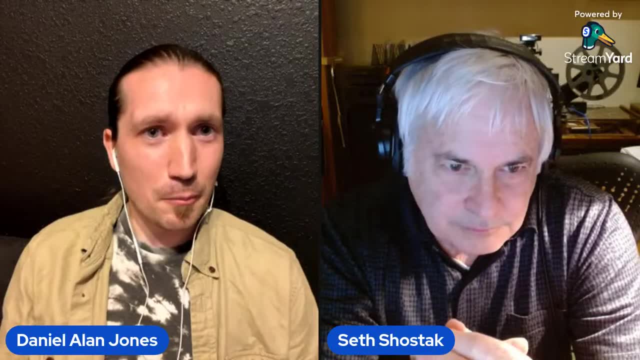 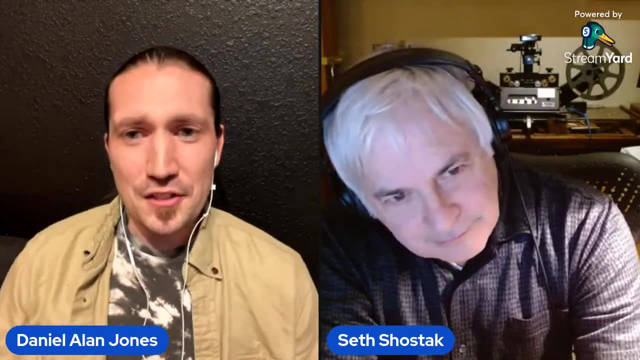 such as yourself, who have the accolades and know how to be able to approach it scientifically and get it to the people, And with this we can shift gears a little bit back into the idea of where we're going and in the scientific direction when it comes to some of these things. 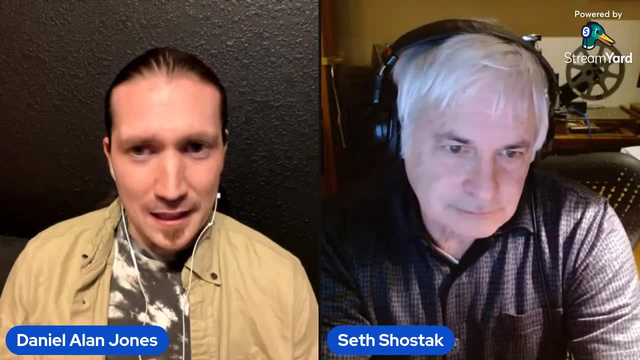 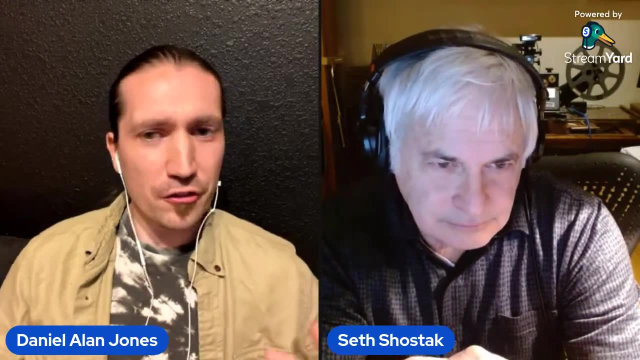 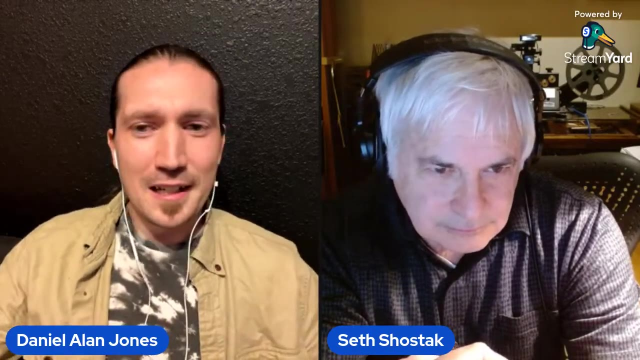 If, in the event that you know, detections were made and said he was able to bring forward some irrefutable evidence, what would the process be? to go from discovery to declaration, Because many people don't understand science and how things don't just happen. 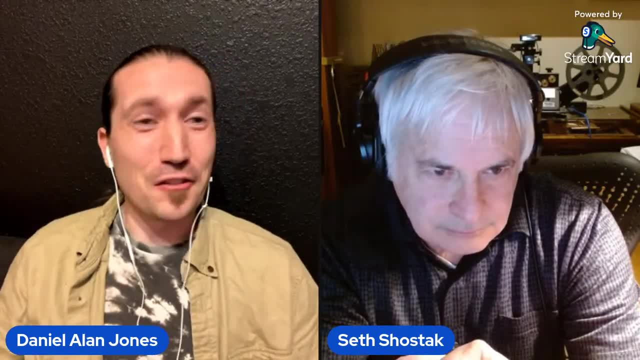 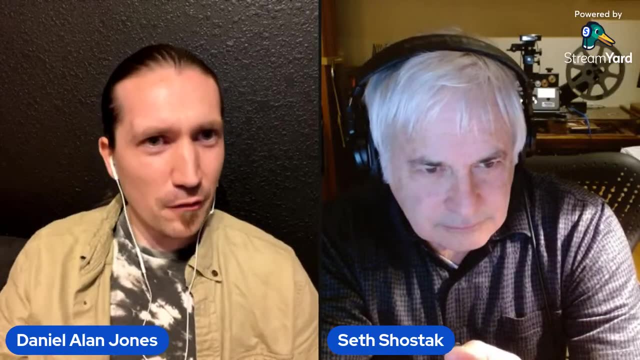 You know, social media can be very spontaneous and things can go live and all of this, but it's not something that happens all at once And can you maybe share a little bit about that process from discovery to declaration when it comes to something of this magnitude? 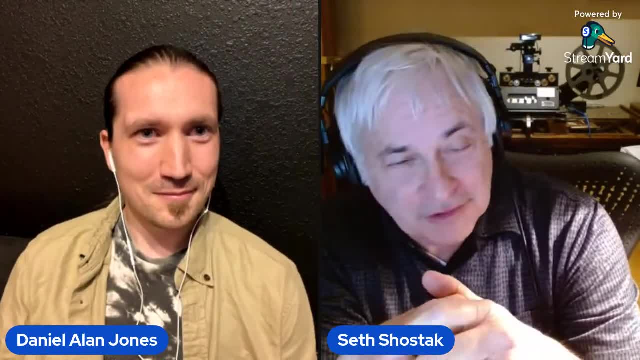 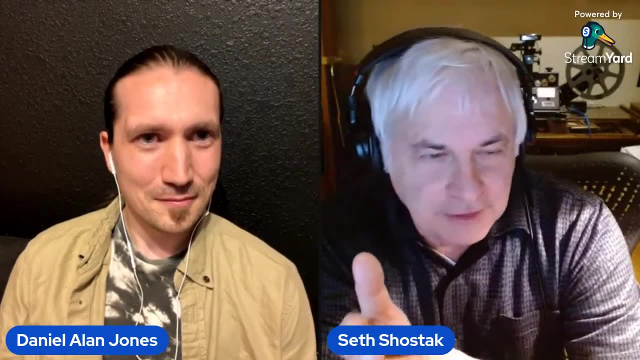 Well, actually it would. it would be pretty much like you would see it in the movies. to be honest, if we were to pick up a signal tonight, right, All right, The Institute doesn't have any. They said The Institute doesn't have any policy of secrecy. 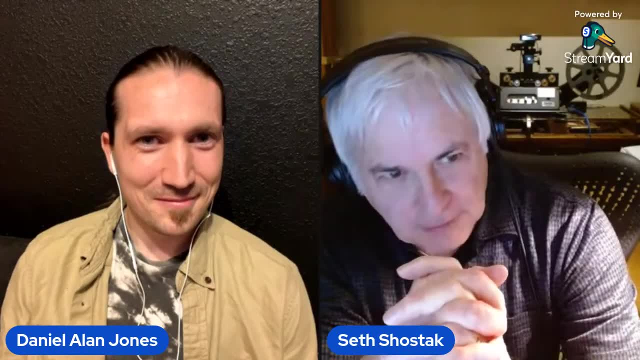 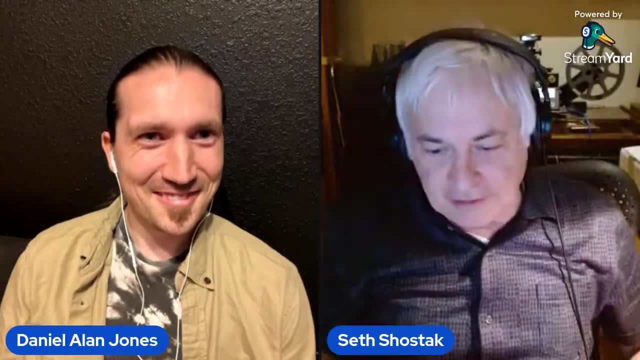 You know, nobody has ever told anybody working there: look, if we pick up a signal, don't say anything about it. We're going to have to clear it with the CIA or who knows what Right, Nobody's ever been told that. 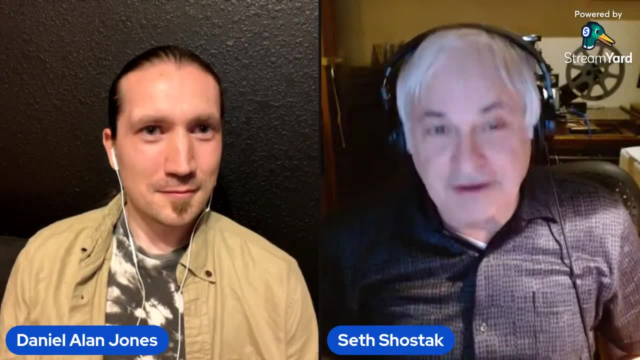 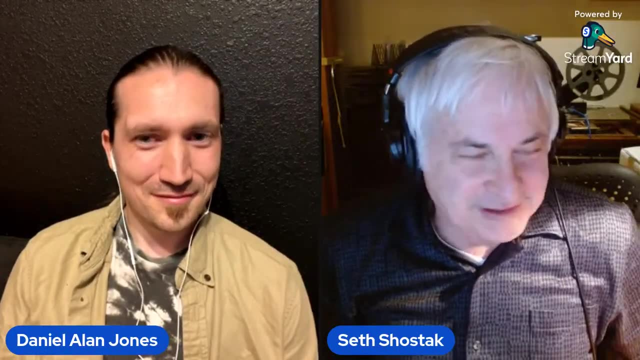 So, of course, if we were to pick up a signal tonight, even if we hadn't yet confirmed it, you can be sure that everybody involved would be, you know, updating their Facebook page to say: hey, we found a signal tonight and it's looking pretty good. 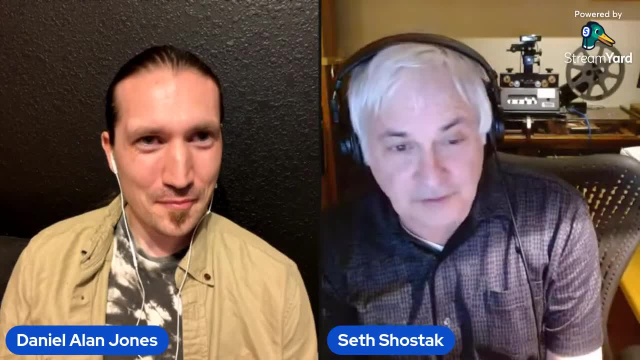 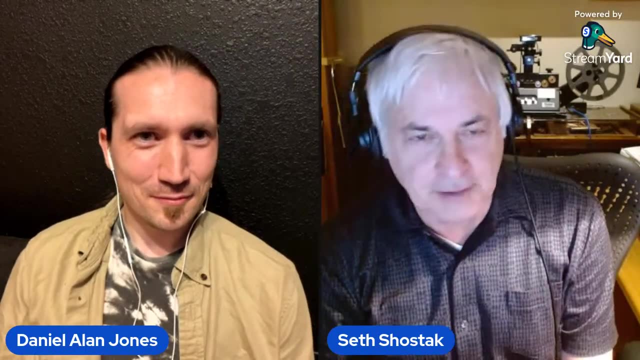 You know, of course they would. of course they would, And, And we've had false alarms and you see exactly that happening Right, And you know we had. Perhaps the most compelling one was in 1997.. We picked up a signal that you know for a while, about a day. it looked like it was the real deal. 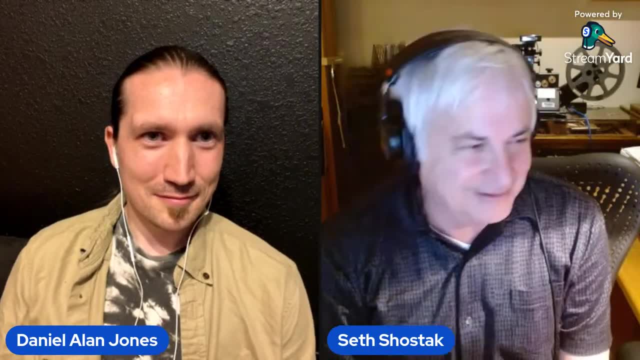 And you know, nobody had told us. well, don't tell anybody, It didn't. And in fact you know, a few hours into it The New York Times was calling me up. They already knew about it in New York. 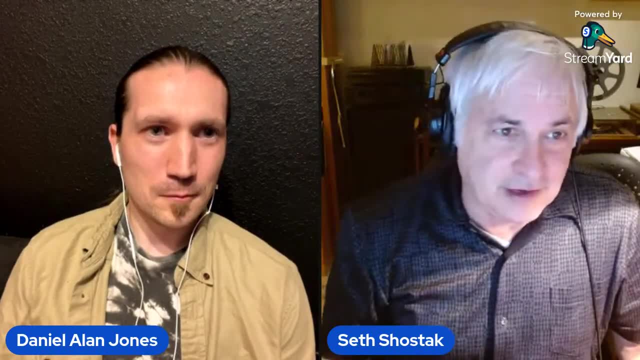 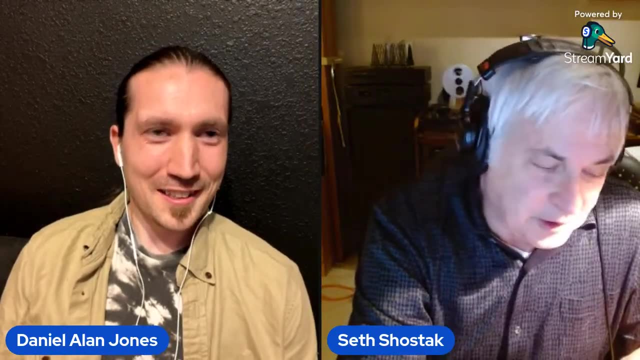 So that's actually the way science works. I mean, you make a discovery and you know there's There's no protocol you're going to listen to, You're just going to tell everybody, Right. So that's what would happen. 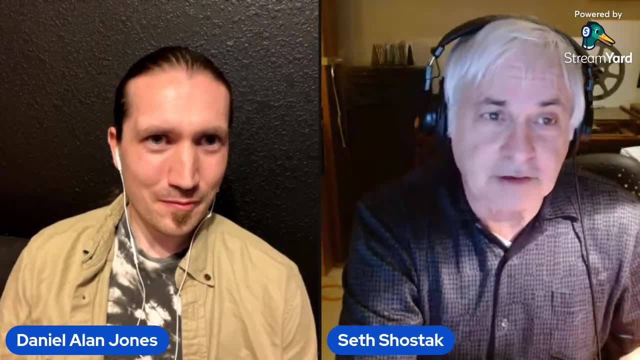 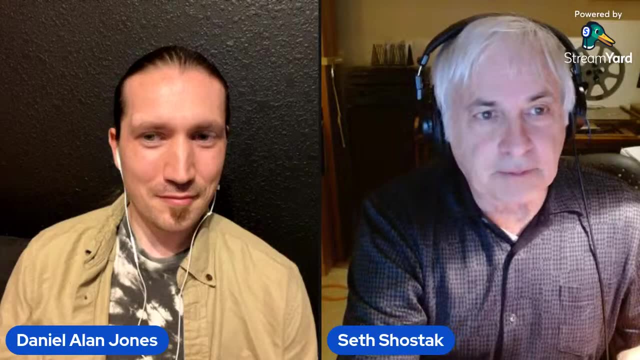 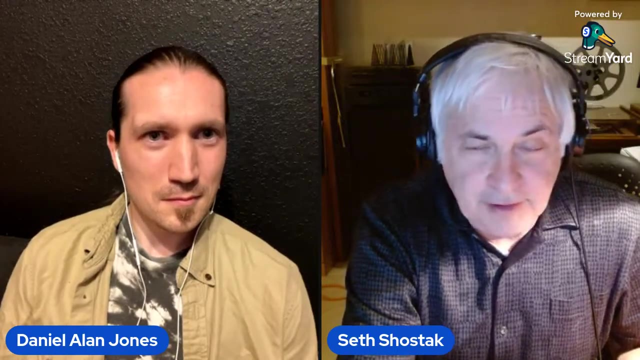 It would be a very big story, And that's actually a good thing, because that means that other people in other countries, with equipment that's not identical to yours will be prompted to also look and see if they can find the signal Right. And if they can, you know, if you find the same signal, but in two different parts of the world, the two different teams of people you know you're going to be inclined to. 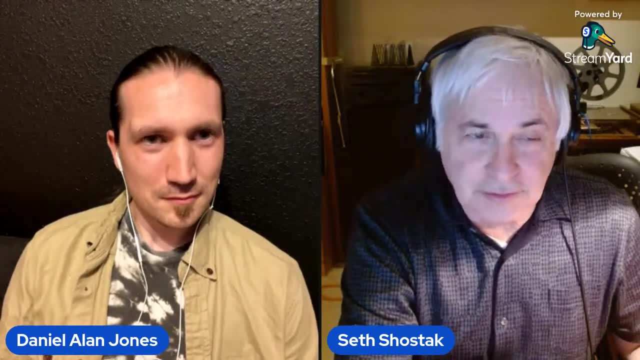 Believe that it's for real. If you can't, you're going to dismiss it and say, yeah, well, there's something wrong with those guys' equipment. So it's a good thing actually, And you don't want secrecy. 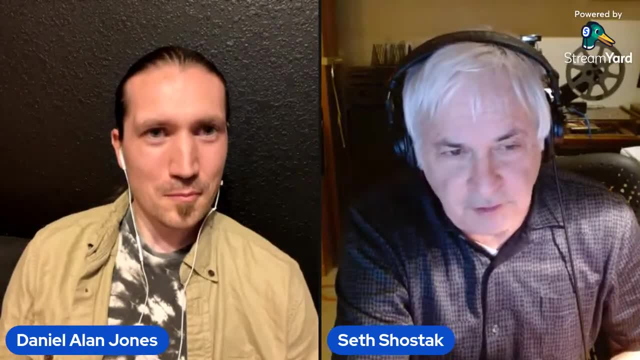 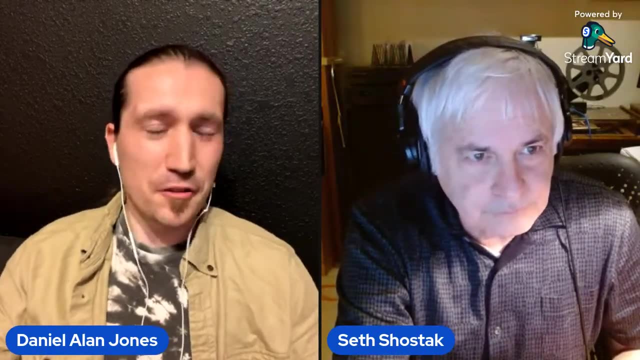 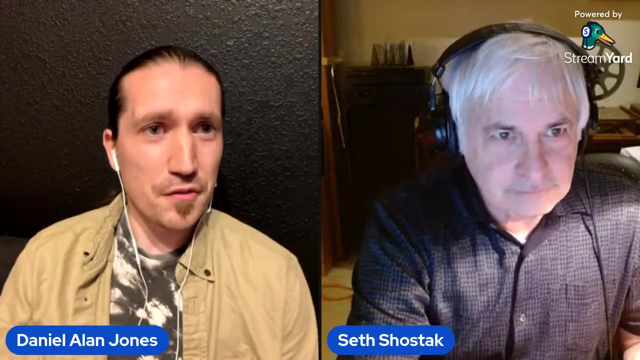 You, just you know, science is very open and that there's very, very few secrets. Well, with those types of discoveries potentially being made and announced to the world, it would seem that a spur of innovation would rise up to introduce several, you know, pre-existing disciplines of science. 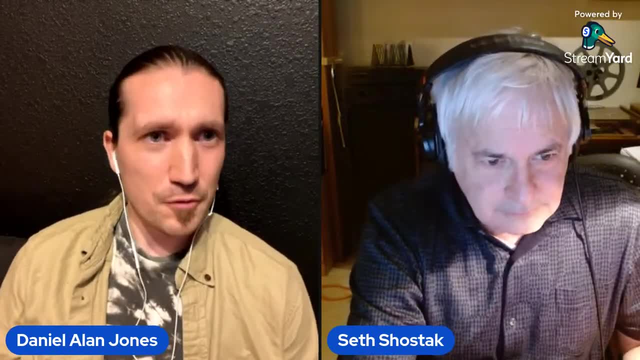 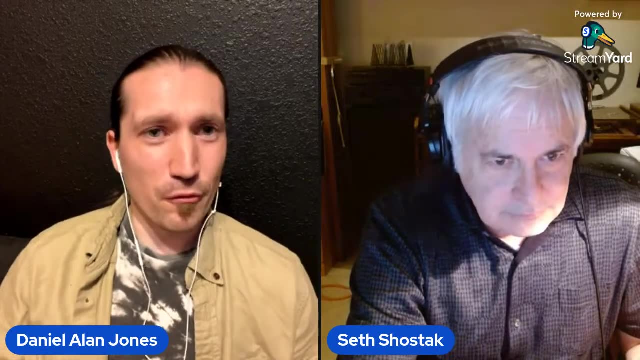 Having these, maybe new possibilities, Possibilities of sub-genres and things emerge in a way that might liken to what we could call cosmic anthropology, And you mentioned a little bit before about the idea of, you know, a sociological outlook and things. 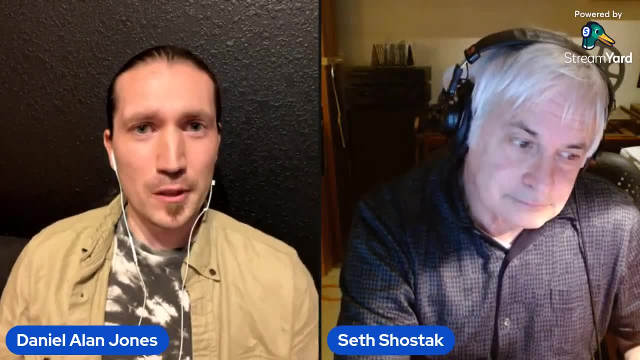 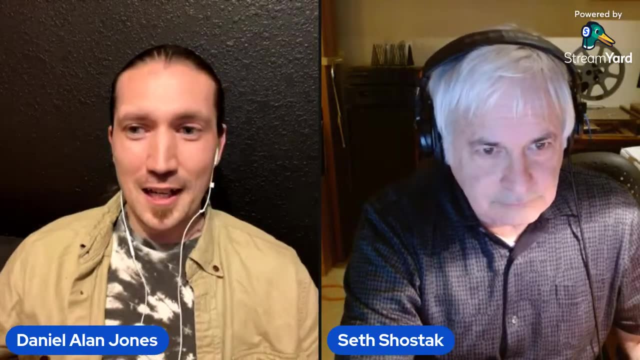 What would you say might be some of the disciplines to come, in the event that we not only make the detections, we declare it here in the world, we raise the standard of awareness in the public and in our societies to know that we're not alone in the universe. 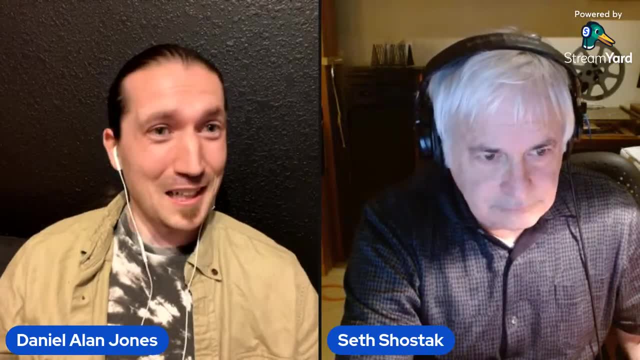 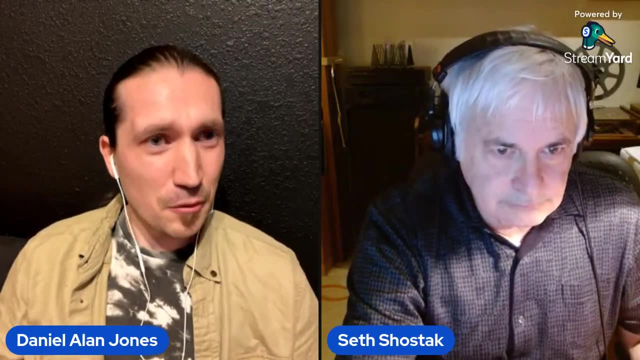 We now know, without a doubt, with, again irrefutable Evidence, that there are others. what would you say would be, you know, some of the different types of- uh, scientific disciplines that might emerge from this type of instance? Well, in the first instance, it's going to be mostly radio astronomy. 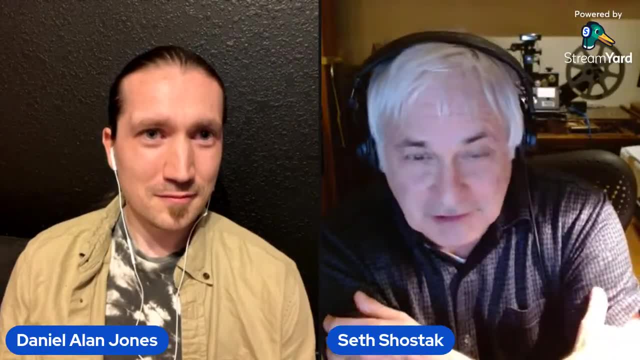 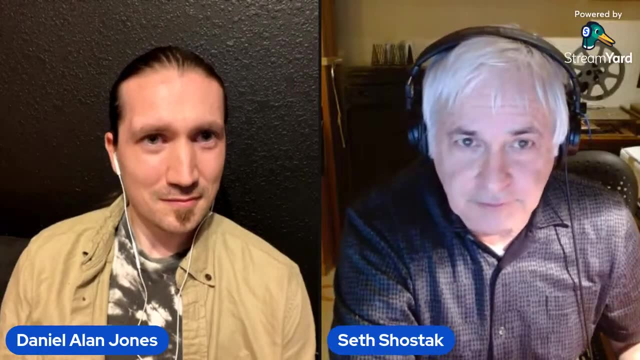 I say that not because that was my discipline, but it's just true. The first thing that's going to happen is you need people who can build the receivers and so forth, And then, of course, you need, uh, people who know something about programming and so forth to uh write the software to make all this stuff work. 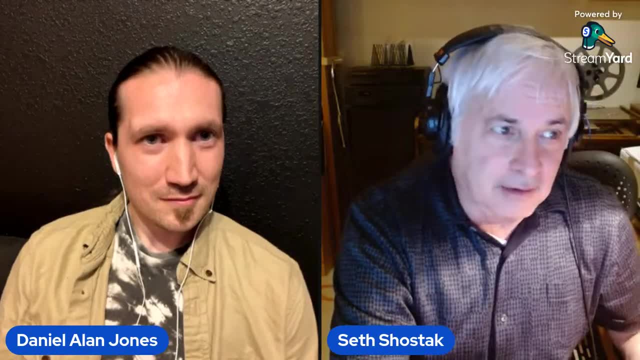 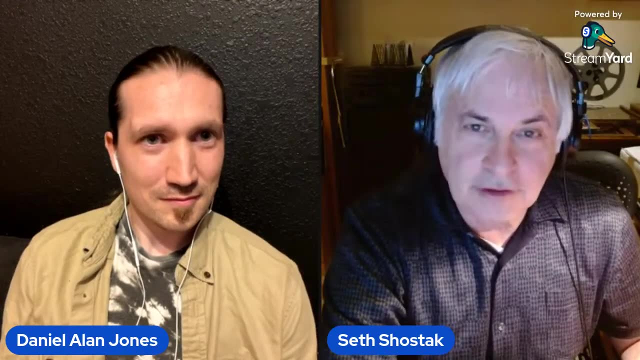 Yeah, Yeah, That kind of thing. But if you've actually made a discovery of another civilization, another society you know, out there in space, okay, I, I, you know, you would want to know more, you would want to know. well, are these guys biological or are they just some sort of machine intelligence? 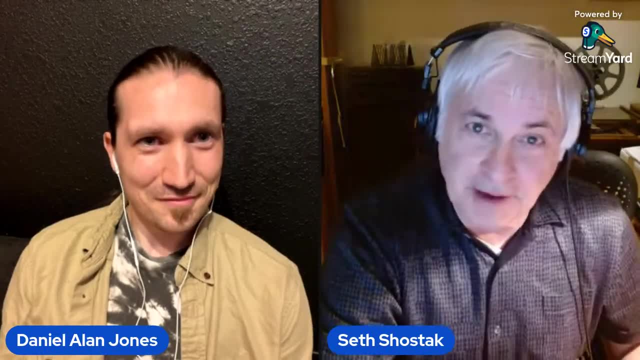 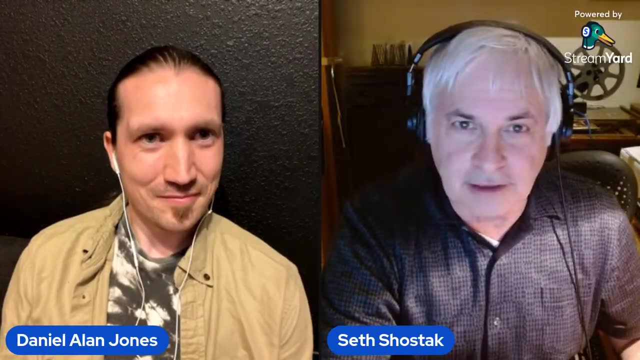 And if they're biological- and I'm a biologist- I want to know more about their biology. You guys don't have DNA. Presumably you have some other molecule for encoding. you know your genome, So tell us about that and that kind of thing. 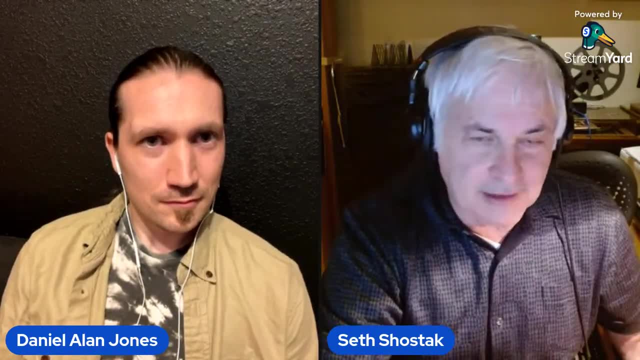 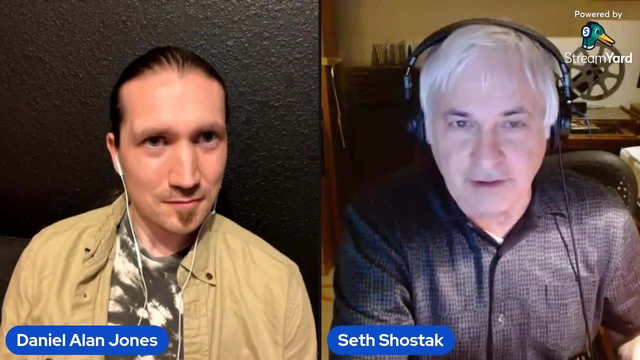 I mean it might be. It's very tedious because you have to go back and forth, you know, ask them questions, set up a language- actually a common language to begin with- and then ask them questions and wait for answers. All of that could take quite a bit of time, but what you would know very quickly is the direction from which this is coming. 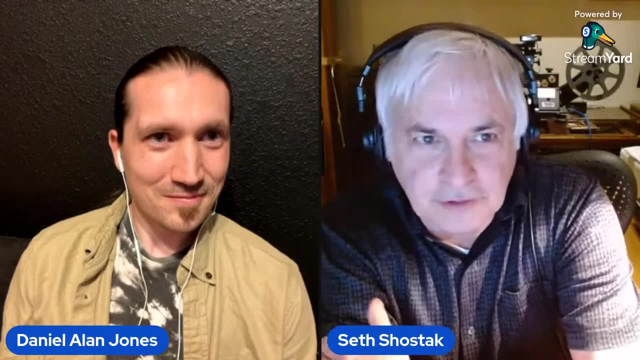 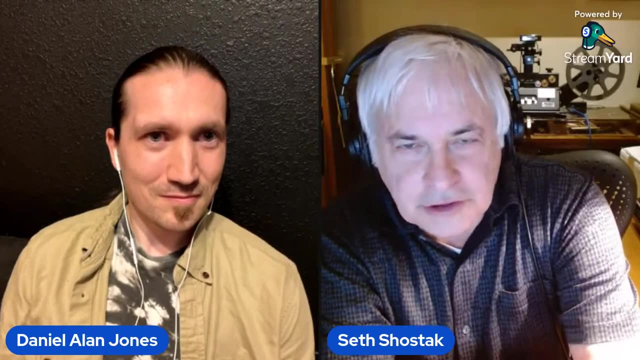 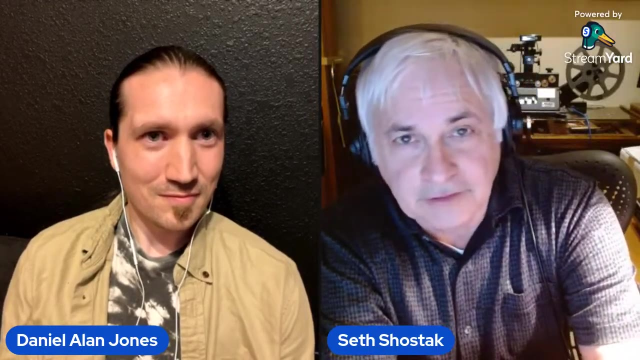 And you know you'd look on the uh, the photos of the sky that are routinely made by astronomers, and you could, I think, without much ambiguity, you could, quickly trace the origin of the signal back to a particular star system, And then the astronomers would get busy trying to see if they could find any planets around that star and maybe zero in on. well, this planet looks like the best, best bet because the temperatures are not too extreme. 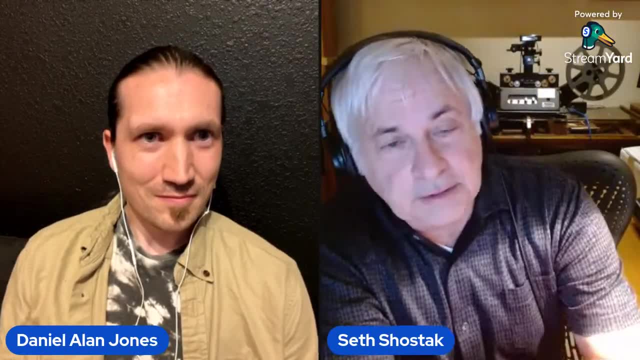 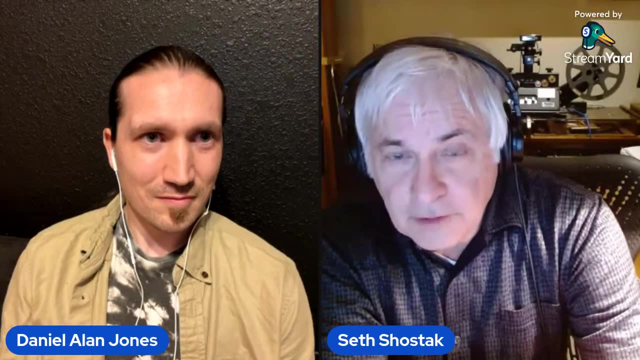 So you could have oceans and so forth and so on. I mean, you would be doing all that- just what's known as astrobiology, really Uh and and. but if you picked up a signal, you would also want to know or be able to answer the question that the public will ask, which is well, what are they saying, right? 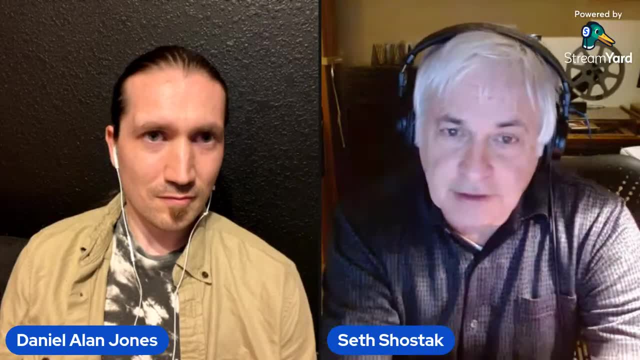 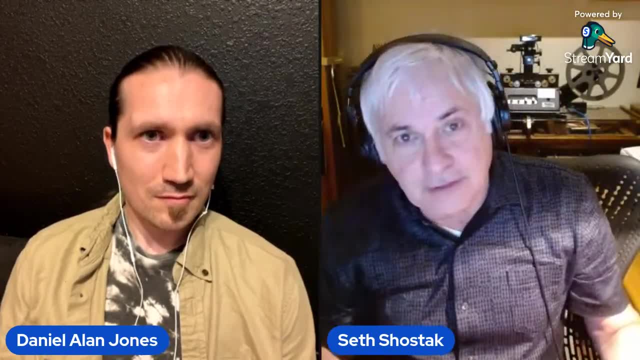 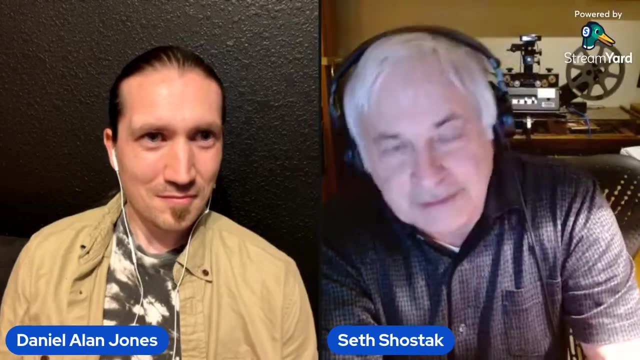 You first have to pick up the modulation on the signal. In other words, you got to pick up, if you will, the sound right On their in their transmission. And that requires building a different kind of receiver than we normally use for SETI. 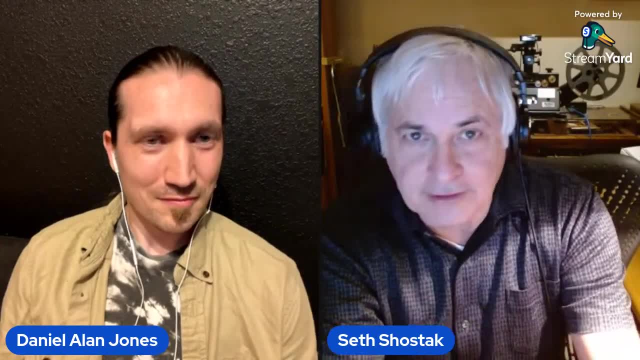 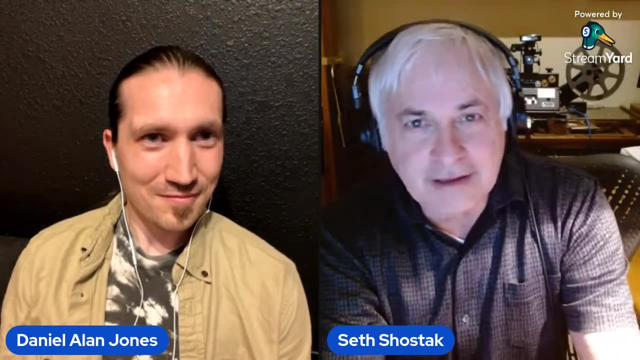 Various technical reasons. but you know you've got to build that. Now you record the sound and now you bring in people who you know are the kind of people who could have figured out the hieroglyphics in the 1830s and have them look at it and 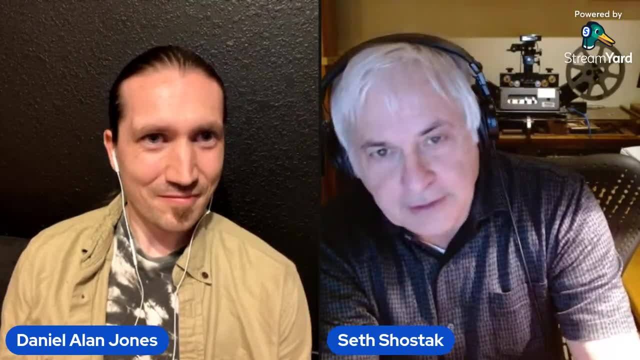 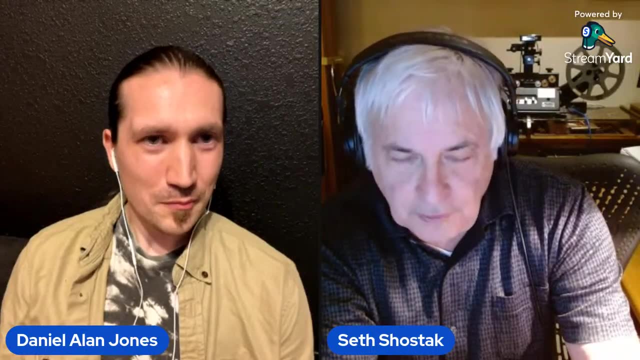 see if they can make anything out of it. You know that kind of thing. Yeah, Yeah, Yeah, Yeah, Yeah, Yeah, Yeah. you would involve people of very diverse backgrounds. So that's good, Nothing wrong with that. And the more people involved, the better. The fewer people involved, the worse. 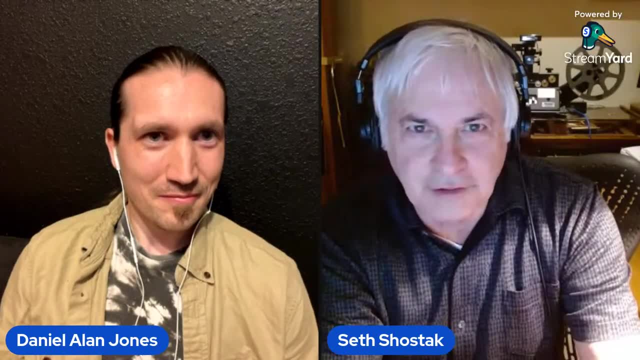 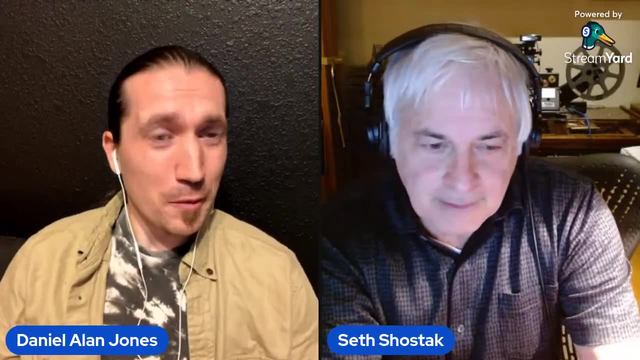 because now you're going to start fooling yourself into thinking that you understand it, whereas in fact maybe you don't Right? Well, you know, it's something I think, as you mentioned, it's going to be an exciting time, a lot of potential on the horizon of the scientific frontier, And 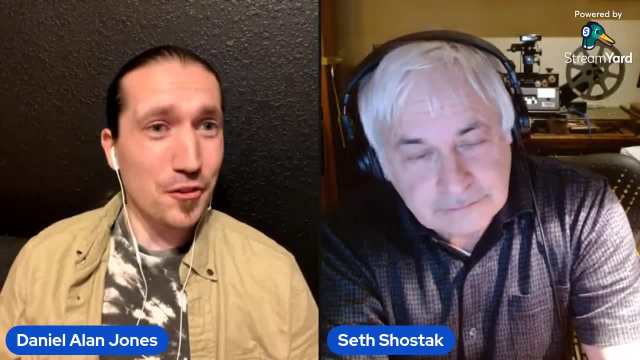 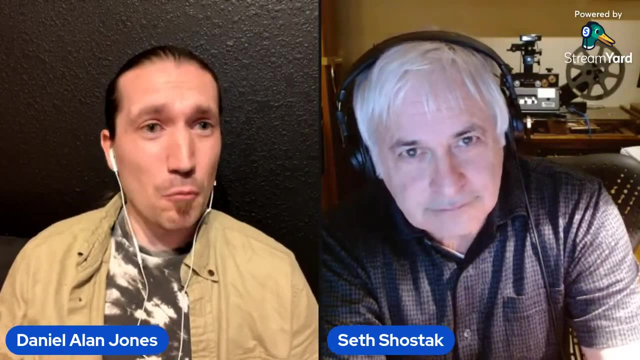 it seems amazing to consider, as you mentioned, astrobiology, perhaps astroarchaeology, astrolinguistics, many different innovations, And when, as you mentioned, we need more people. there are a lot of young and curious minds out there who are interested in this. 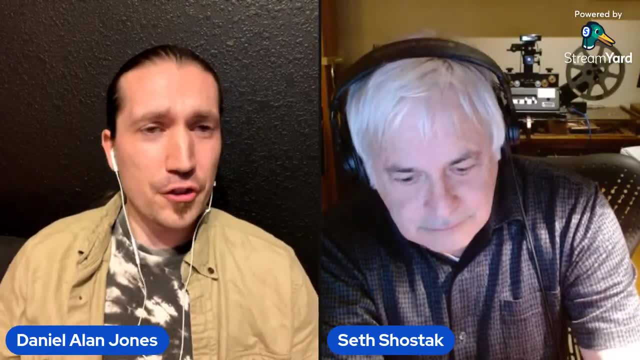 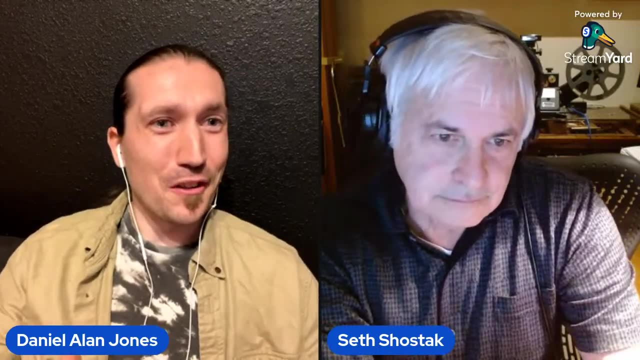 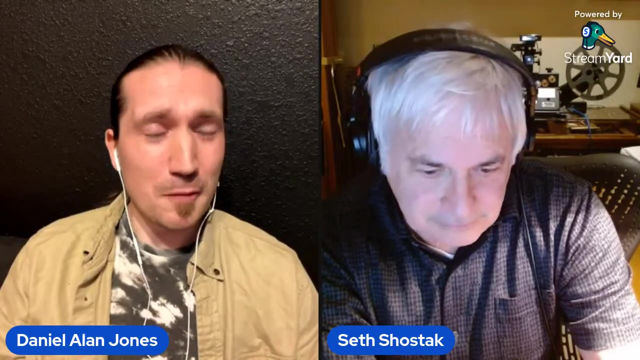 And, in closing, what would you say is a send off for those who are interested: You received the Carl Sagan Prize for Science Popularization And, as Sagan was one of the biggest popularizers, as for science and astronomy in general, in a similar light, you're doing very much. the 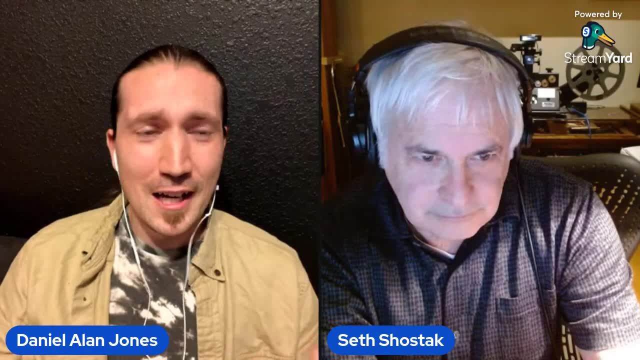 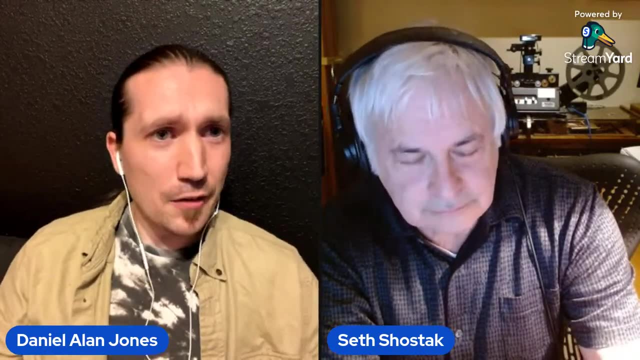 same effort And I think that's important. to see that people know that this is science is fun, it's exciting. What would you say to people who are going to be the upcoming generations to help carry on this legacy and what they can do to get involved, whether it's citizen science or 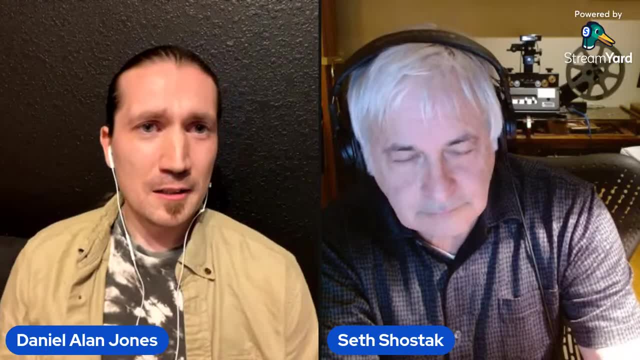 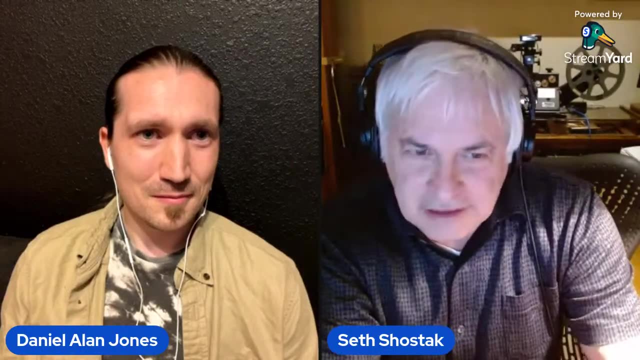 academic research. How would you respond to that? Well listen, I would just tell them to follow their interests. right? We don't spend- I mean, SETI is an extremely small niche activity- only because of the lack of money. right, That's only the only reason. 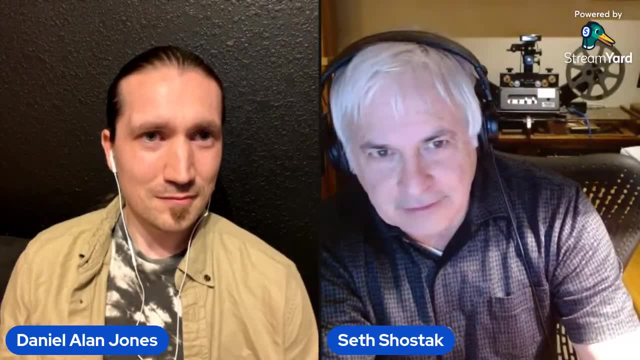 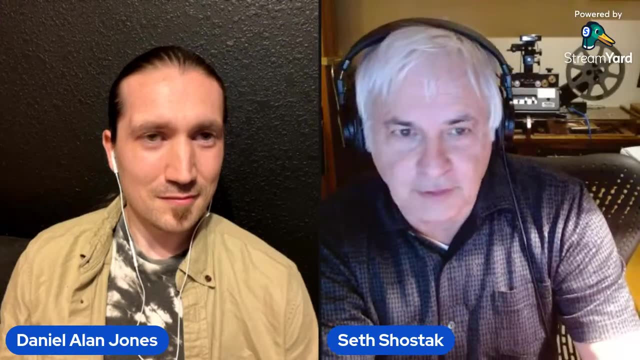 When I joined the SETI team, as I say, in the late 1990s- or actually not even as late as that, it was the early 1990s- there were like 50 people. That was the NASA SETI program. 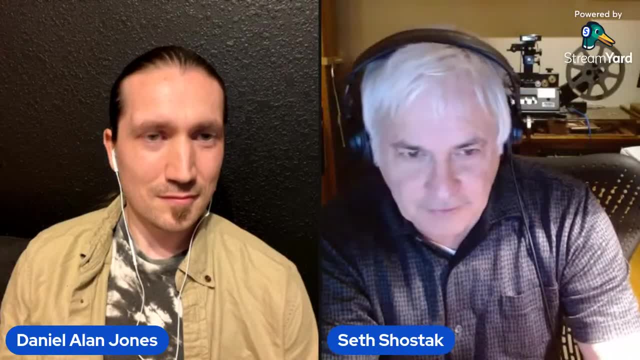 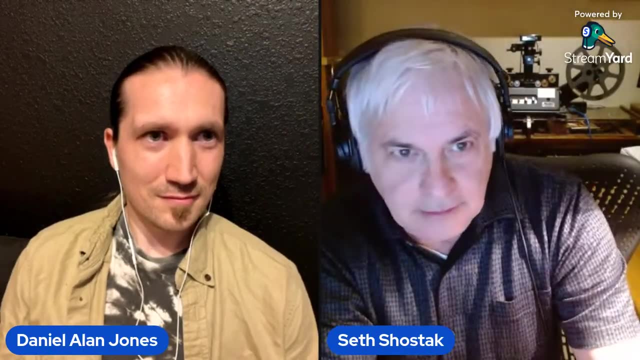 But when the NASA program got killed, you know the number of people involved in SETI. you can count on. you know your two hands. It's a very small number, but that's money. that's money And in the future I hope that that will be better. So if you're somebody who's been watching, 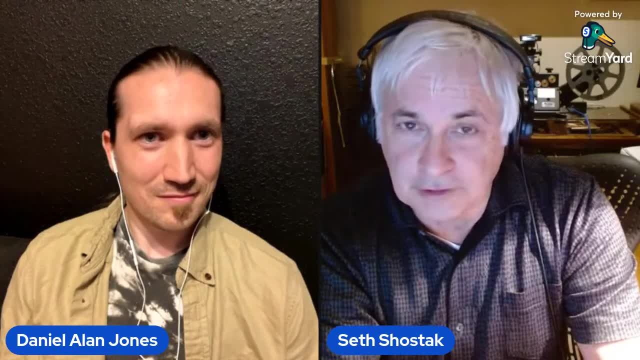 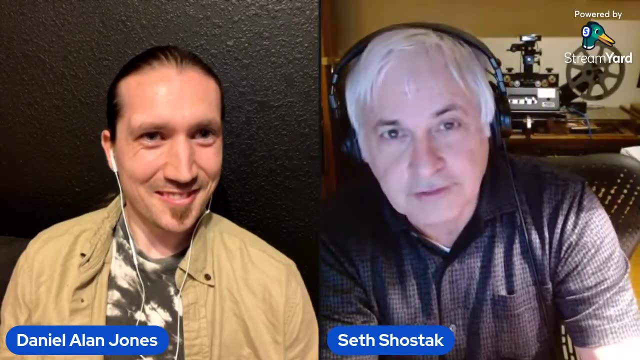 this and you think, oh well, you know, that sounds like something I'd be interested in doing. all I can do is tell you the stuff that you already know, but I'll tell it to you anyway. And that is, you'd be most likely to get a job in this field if you know something about the. 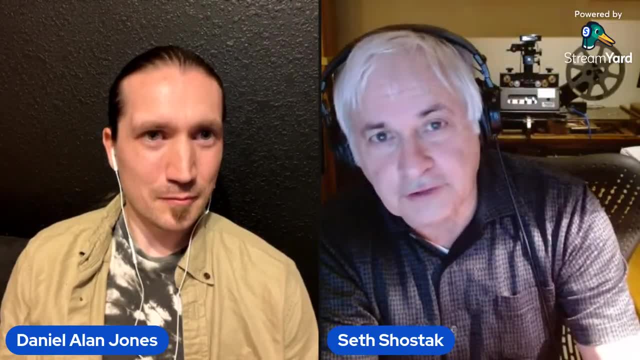 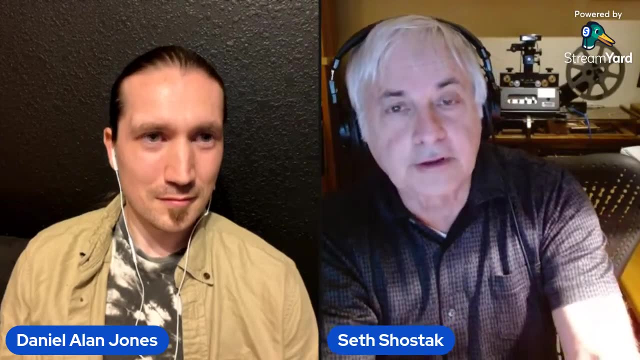 disciplines involved, And that's astronomy, obviously, but also physics, double E, you know, electronics to develop the equipment, and so forth. But there are other things like geology and biology and so forth, all of which pertain to the question of life beyond Earth And studying 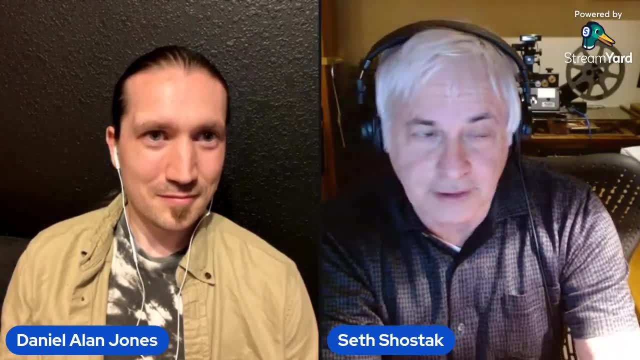 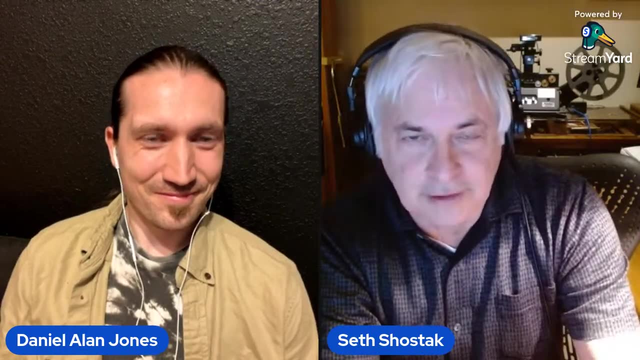 any of those would be helpful. Probably you've got to get an advanced degree. I'm thinking of all the colleagues I know at the Institute, and there are very few people there that don't have a PhD, So I mean that are doing the science. So you know, that's something else. 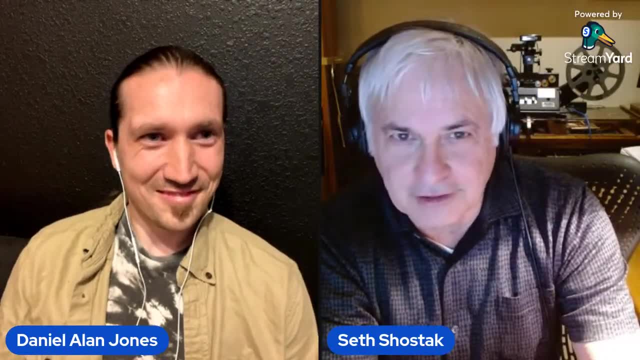 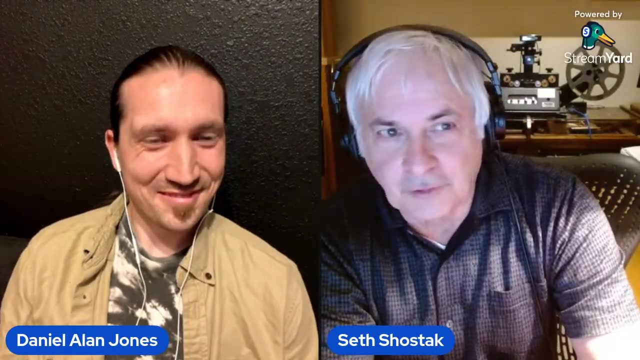 and maybe that doesn't appeal to you going to school for that long, but actually it gets more interesting the longer you stay at it. So you know there's no secret sauce here. It really isn't. If you want to do this, you can do it, but you just have to prepare yourself, You know. 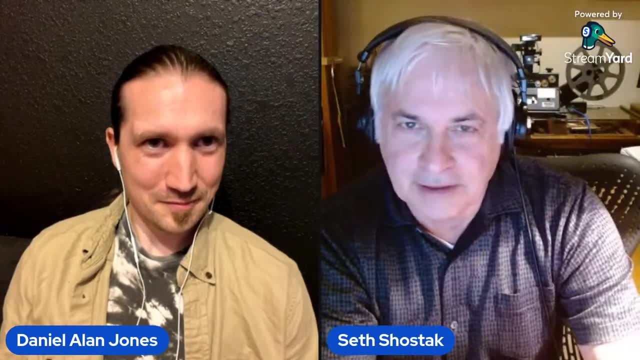 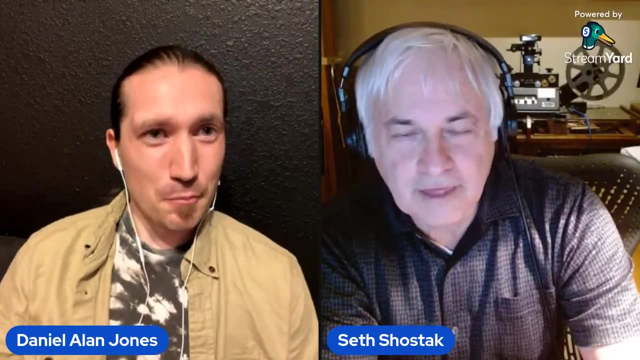 you got to know the territory, as they said in the music man, Awesome. Well, for those who are interested in following with the work that you're doing, looking into any of the books that you've published or maybe coming out with at some, 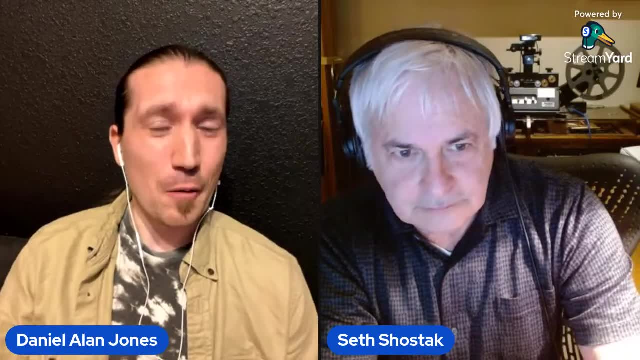 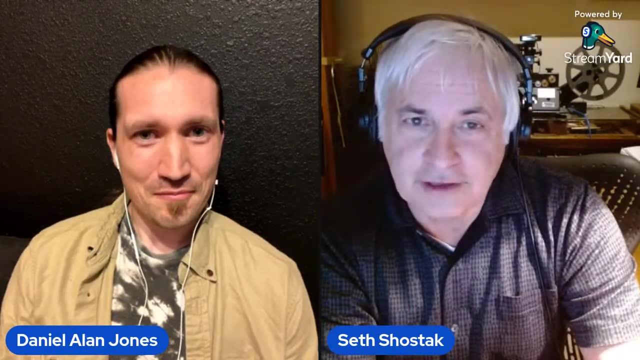 point soon or attend any events that you're going to be making appearances at. where can they go to find out more? Well, you can always go. I mean, obviously I have plenty of colleagues- but just go to the SETI Institute's website.